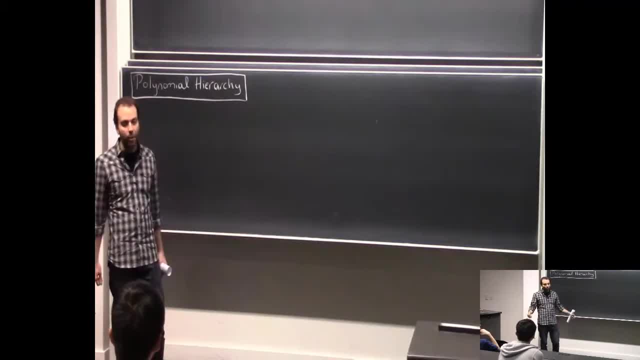 complexity classes, like you know well. obvious examples are like: P- polynomial time, NP- non-deterministic polynomial time, log space, L- non-deterministic log space, NL, P space, polynomial space, X- exponential time- non-deterministic exponential time, and so on. so, so there's a big zoo of complexity classes actually. 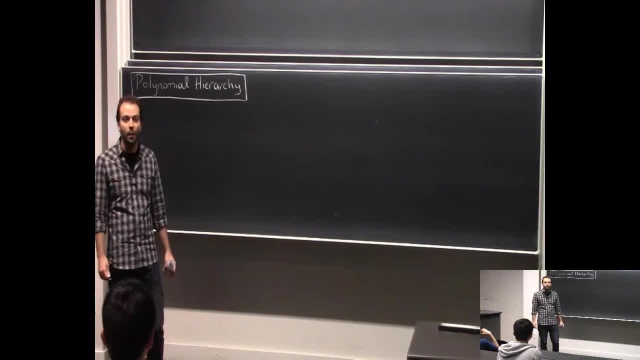 and you can. you can google complexity zoo and you will. you will see that zoo. there are thousands of complexity classes and one of those important complexity classes is the polynomial hierarchy. so I'm gonna introduce this to you. it's yeah, as you'll see, it's kind of 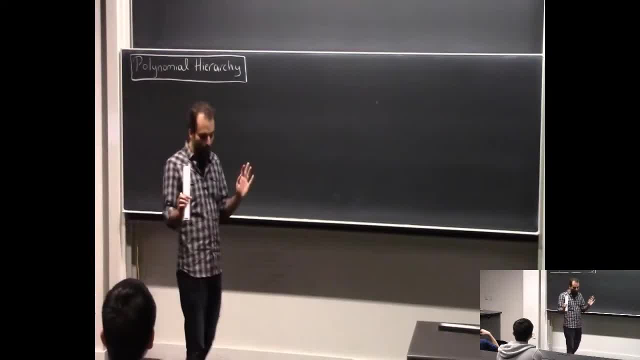 like mind-bending a little bit. like the first time you see the definition of MP, it's kind of can be a little bit mind-bending, like you're not used to that kind of definition, and then here you'll see that there's like a hierarchy of 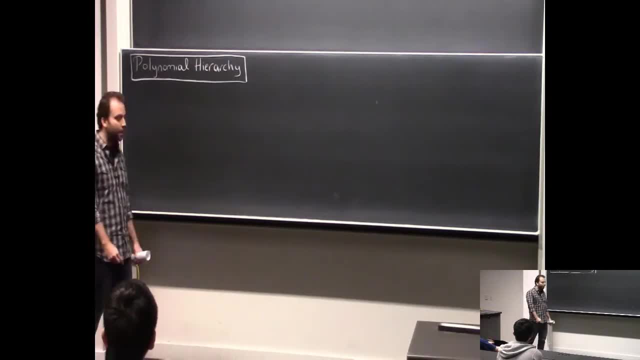 mind-bending going on, okay, and but it's cool, like when your mind is being bent like that, then you really know you're learning something new, okay, so first I want to, hey, I want to remind you the definition of coin P. so I'm told that. 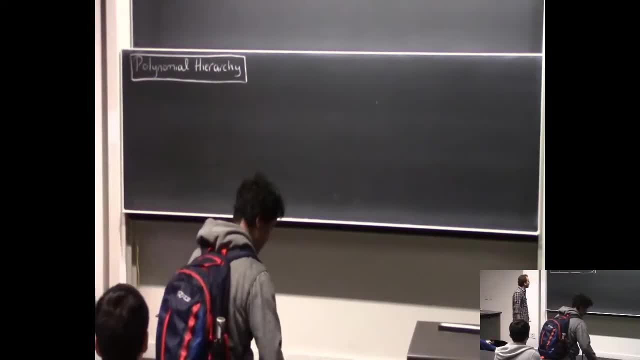 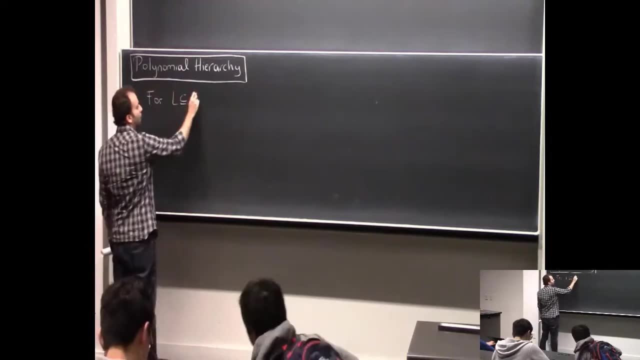 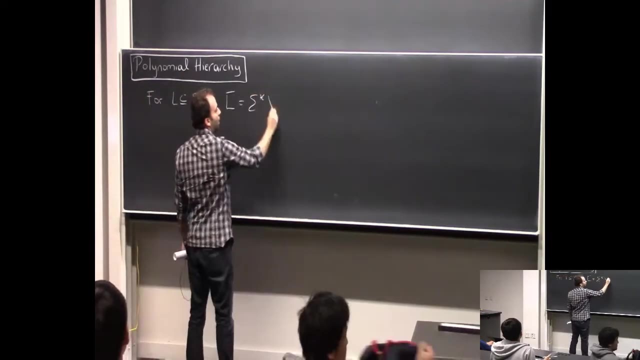 you know you're comfortable with coin P, more or less, but let me just remind you very quickly what coin P is. so, for instance, I forgot to point out- for instance, the same thing we've defined in Sky Innovation Laboratory. for example, if we take a DeepSabochure, 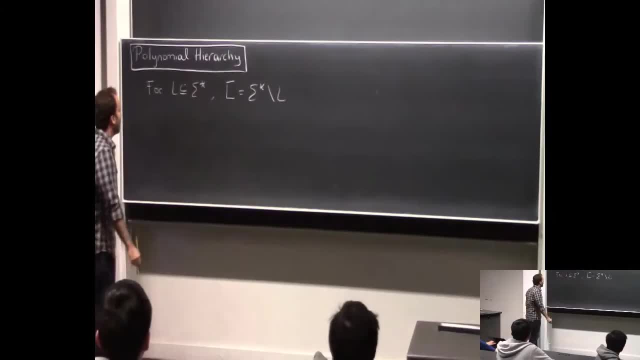 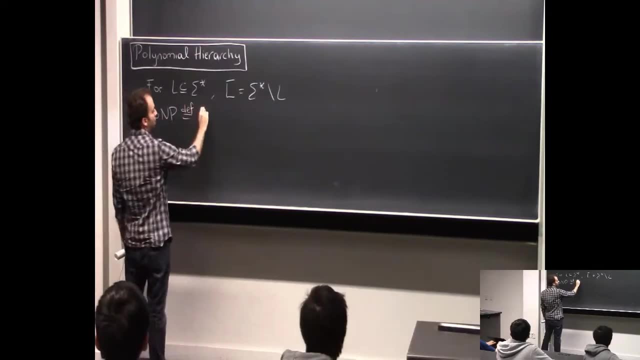 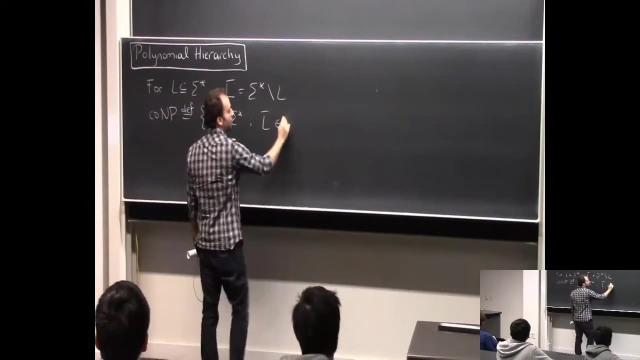 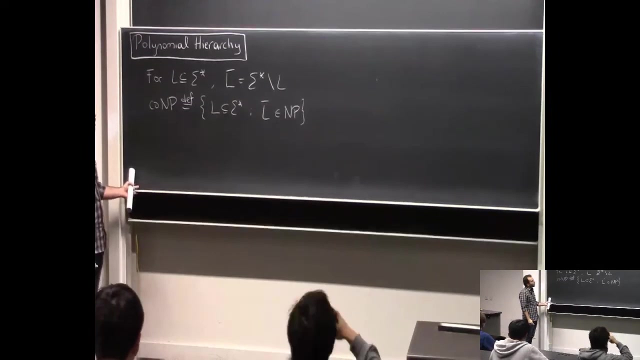 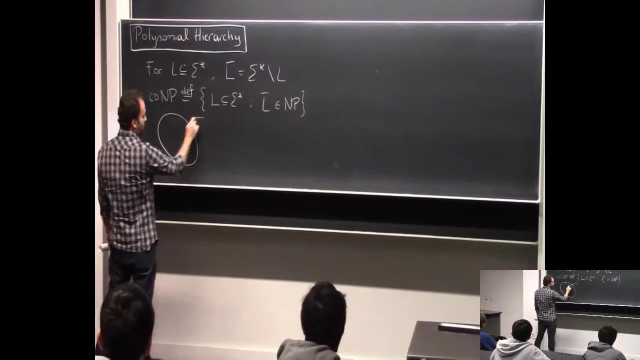 algorithm and you know, put L phonetically and we 차 salt L, a language Sigma in Sigma star. the complement of L is Sigma star minus L, and then we can define co and P way to define co-NP. And we know that, for example, if I draw these things, I guess 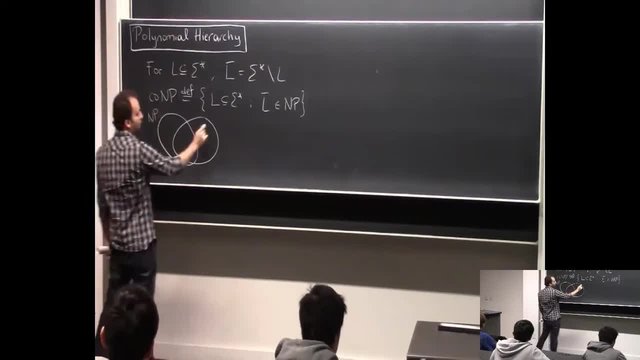 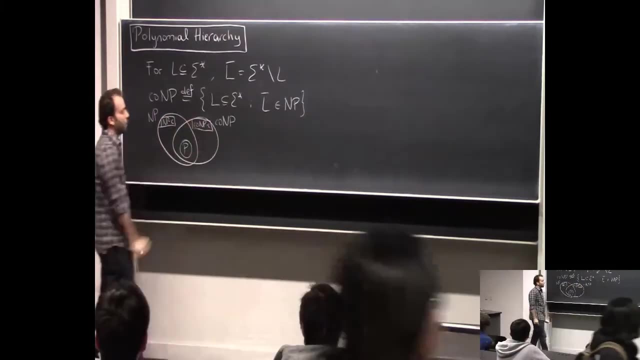 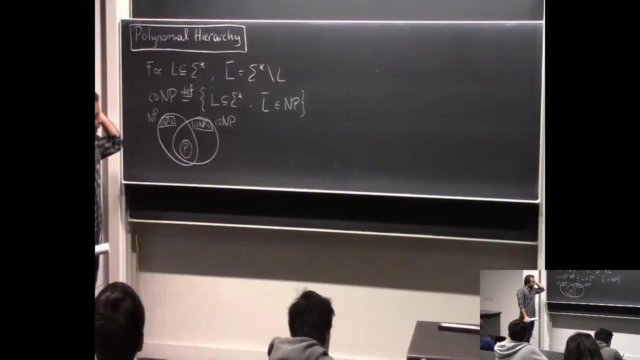 So this is, let's say, NP, This is co-NP. NP lives here And you have your NP complete languages here And you have your co-NP complete languages living there. So we believe these complexity classes are different. So you might say like: 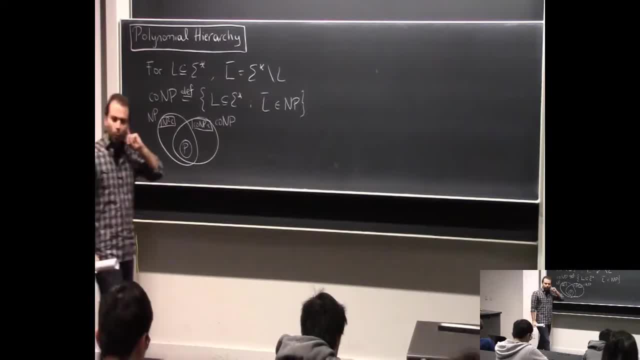 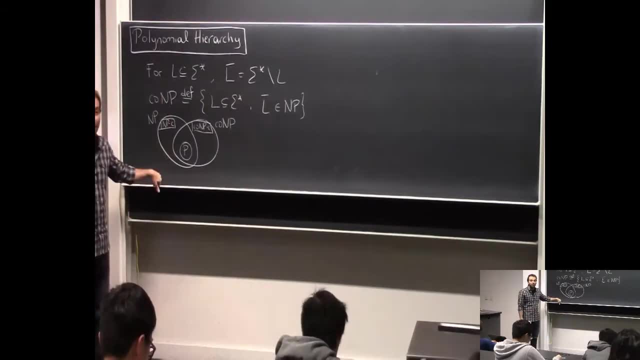 what's the motivation to define co-NP? Well, the motivation is well, NP is a one-sided definition. It requires you to verify efficiently, yes, instances. But there are a number of reasons to define co-NP. There are a number of reasons to. 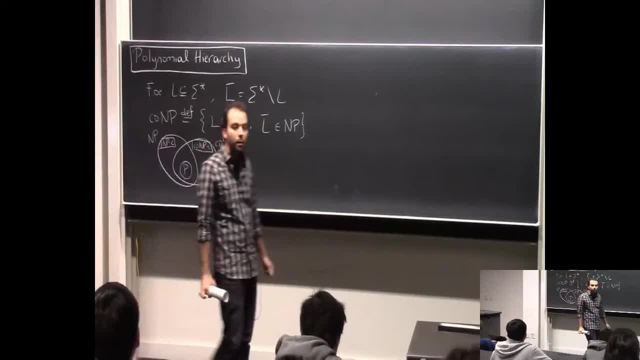 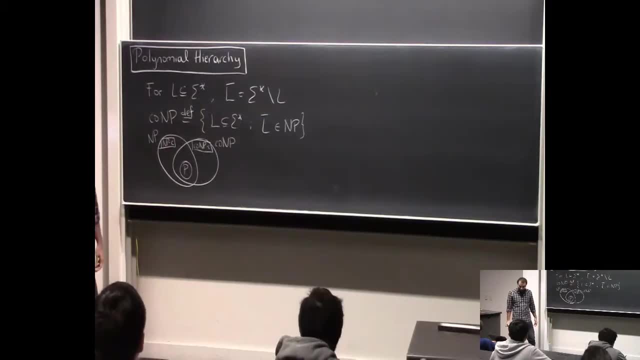 define co-NP. There are a number of reasons to define co-NP. There are a number situations where you might want to verify no instances efficiently. So, for example, if you take the complement of SAT and if I say this complement of SAT, 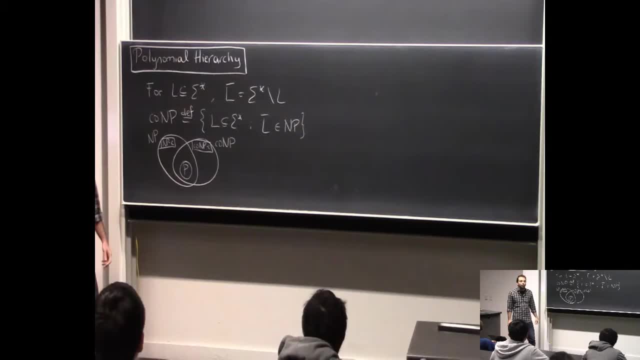 in NP. well, you know, if you think about it, you're going to run into trouble. How do you come up with a short proof that verifies that a certain Boolean formula is not satisfiable, right So? but these problems, not SAT or like not. 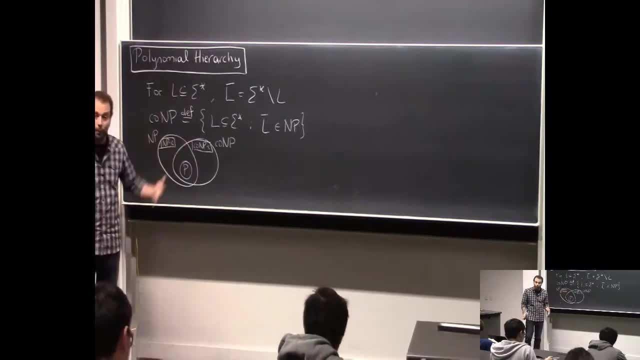 click or take any NP complete problem. look at its complement. These problems live in some natural complexity class. The natural complexity class that they live in is co-NP. Okay, so now I want to actually define co-NP in a bit different. 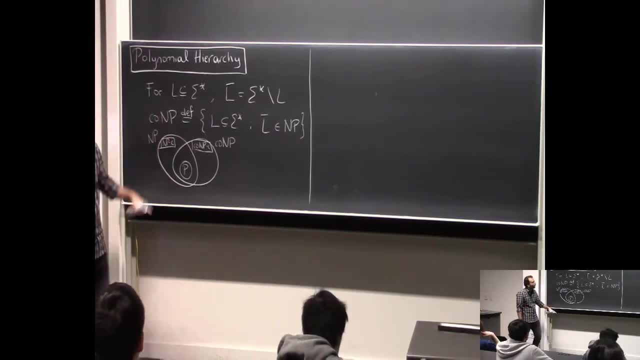 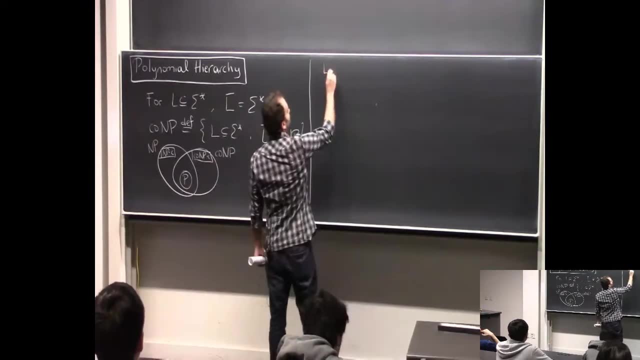 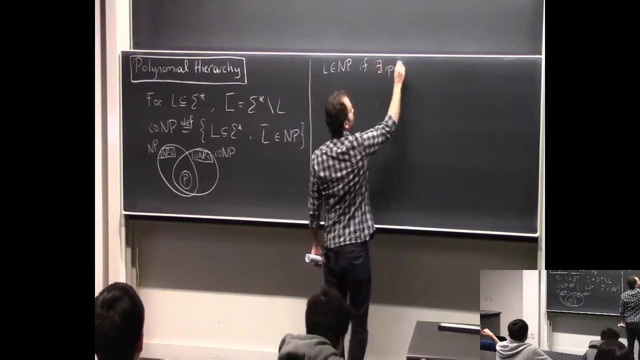 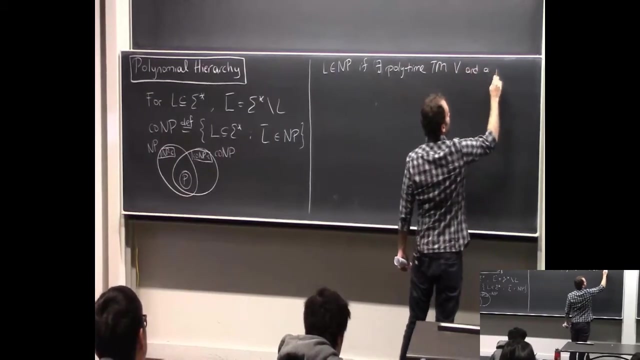 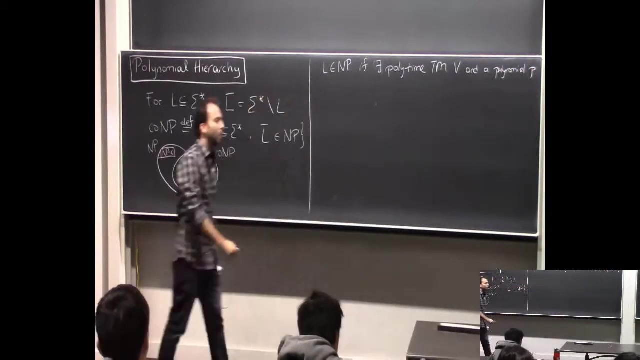 way that resembles actually the definition of NP. So first let me remind you the definition of NP very quickly. So we say that L is in NP. if there exists a polytime Turing machine, V, and a polynomial, let's call it P. So there are various equivalent definitions of NP, but in this 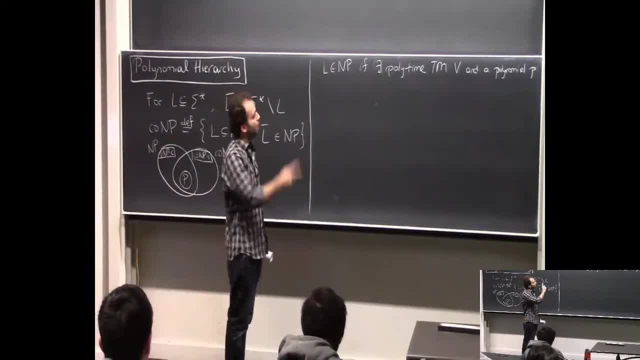 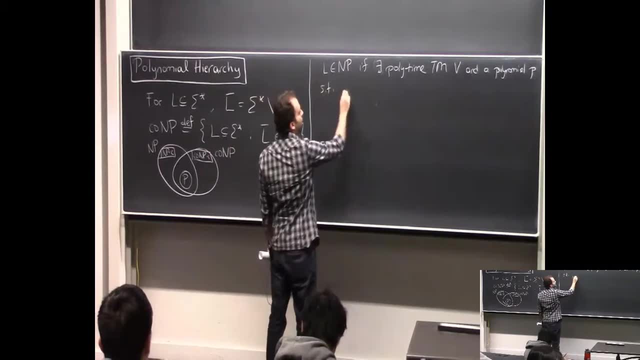 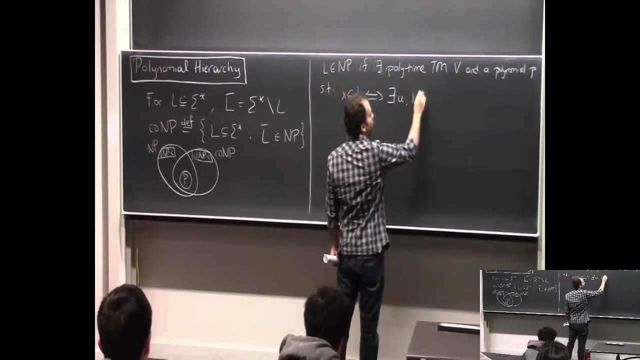 lecture I want to use this particular definition. So L is in NP if there is a polytime Turing machine, V, and there is a polynomial P, such that X is in the language, if, and only if, there exists some U where the length of U is equal to. 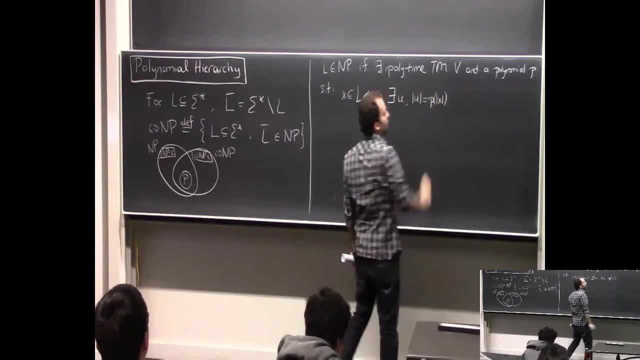 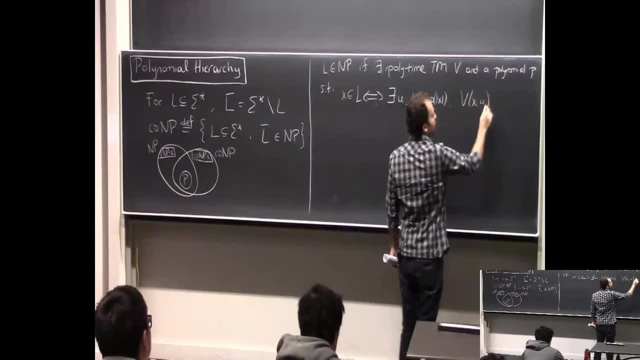 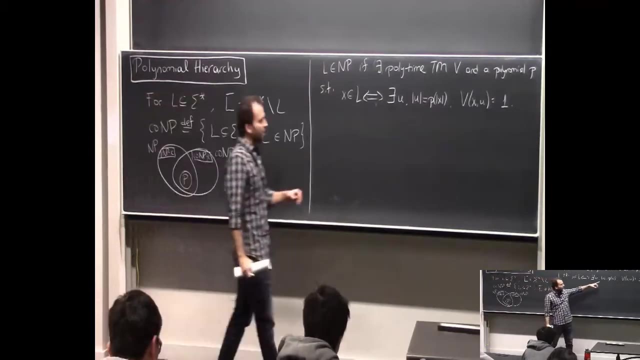 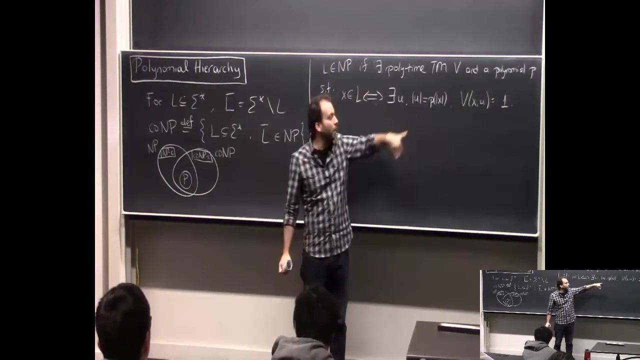 this polynomial, with the input being the size of X, and V is one. So one thing that I'll just highlight here is that I'm insisting that the certificate U is exactly of length P of X. This is okay to do If this was less than or equal to. 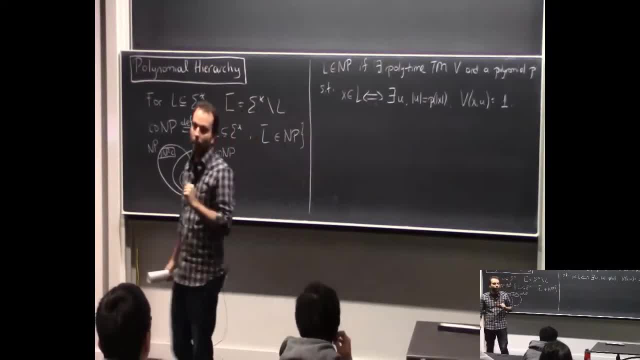 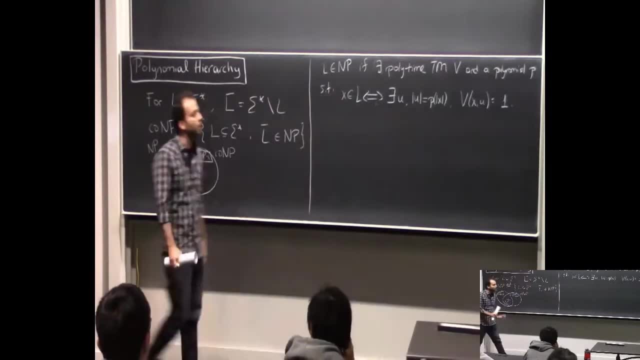 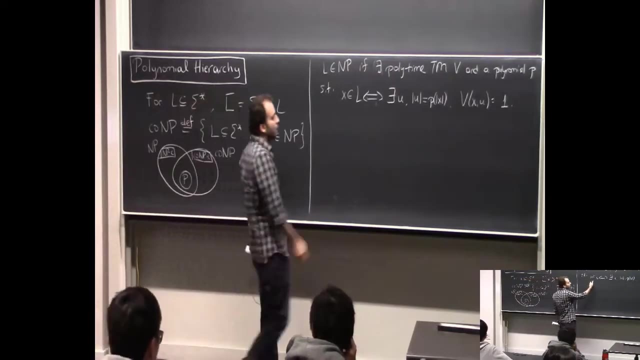 I mean, I can like artificially pad the proof string. So this is not a problem, but it's a convenient. it's going to be convenient for us to say that it's exactly P of X. Okay, good, So that's the definition, And then you can say, okay, look, this is the. 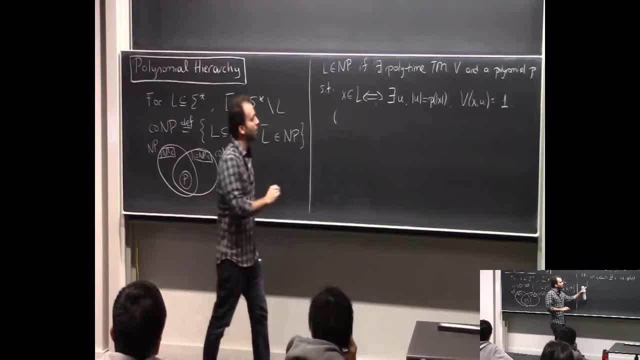 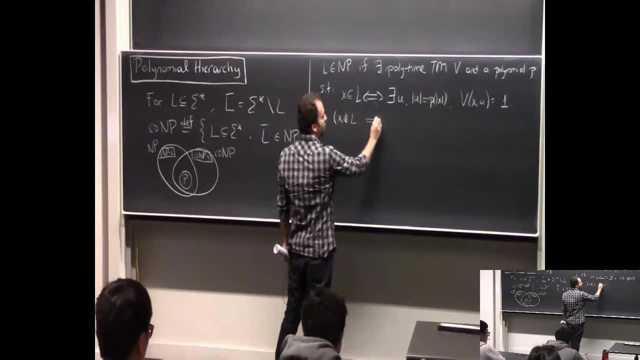 många. I can rewrite this condition This: you can see that you get type affix Here. there also has a speckle, but you just accept this thing as the name Or you can push selection out. So this is also the name of a row call. 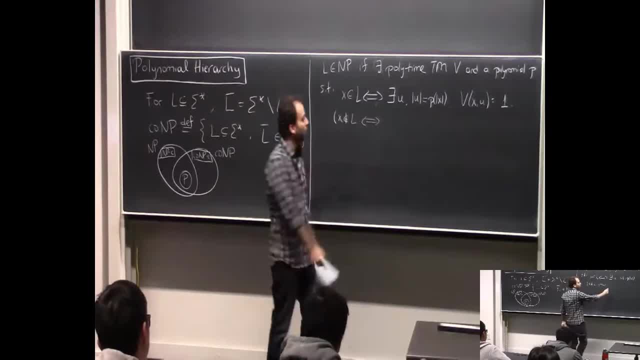 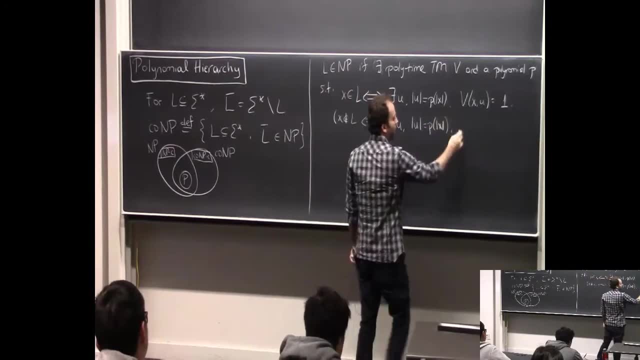 of the space, these, equal to What is find onion, is I say Pt, dash cube times plus distinct. You know, you don't know T is, but you already added in and now we are allWhat do we get? Can we write it out here? No, sorry Parents, how did you write U? 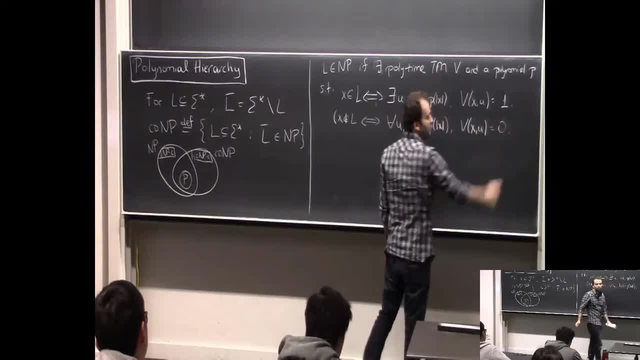 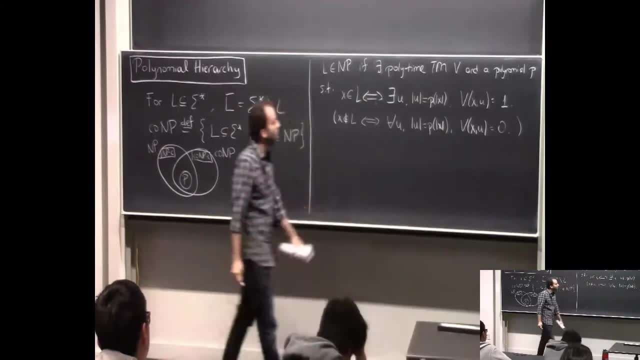 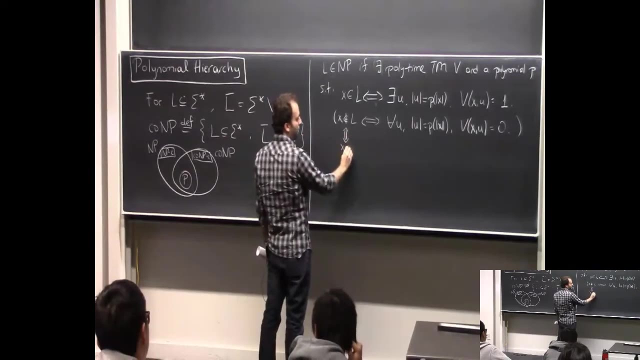 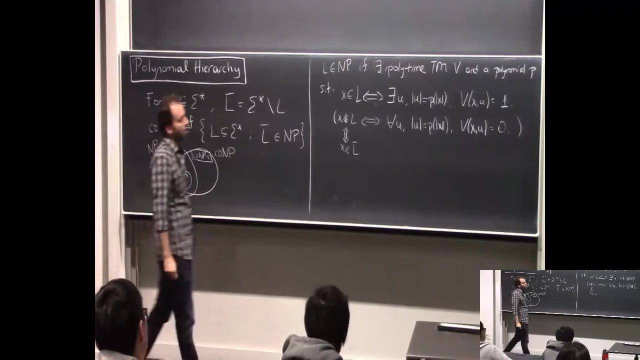 Yeah, T, OK, 16.. Right, zero, Okay, so that's equivalent. But now you can say: well, this is like equivalent to x in L complement Right. so x is in L complement if, and only if, for all u of polynomial length. 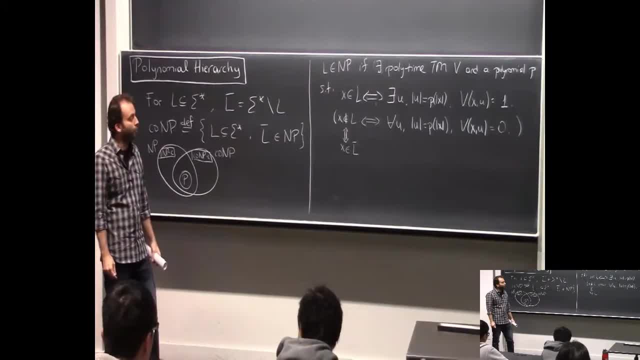 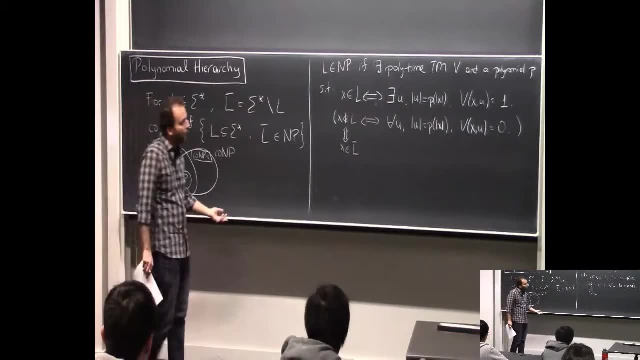 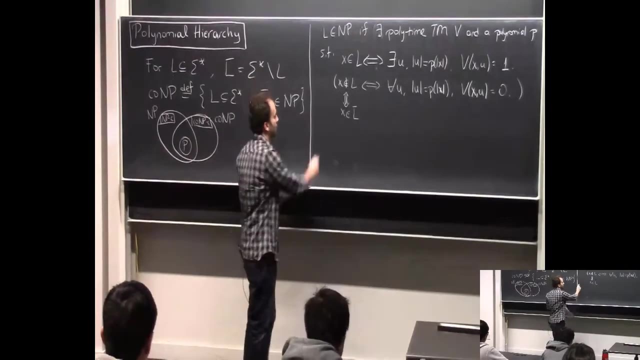 vx- u is equal to 0.. Yeah, so then you know, at this point you can say: cool, why don't I then define co-mp in this way? so I can say I will say that, so this is definition. 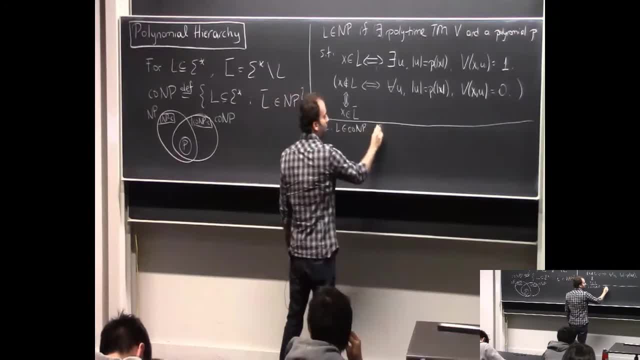 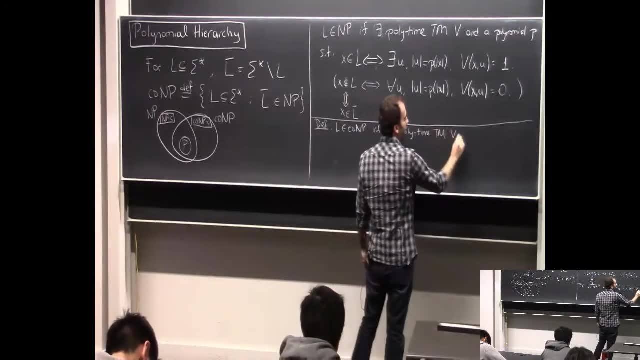 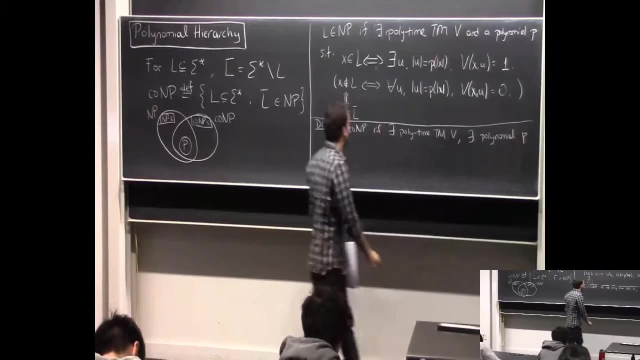 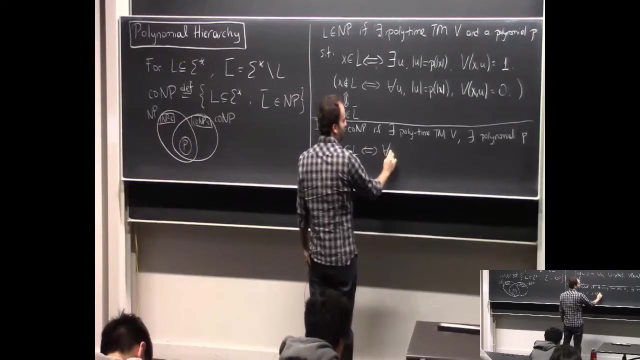 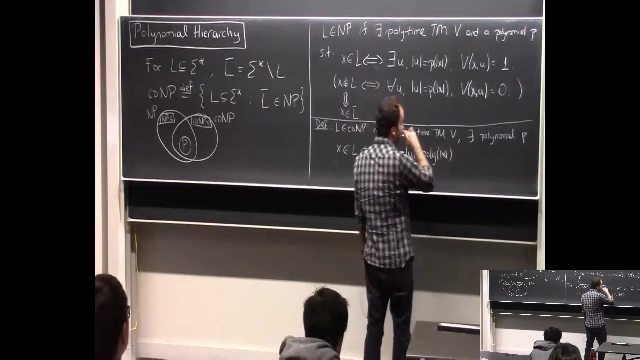 L is in co-mp. if there exists polytime Turing machine v, there exists a polynomial p, such that x is in L if, and only if, for all u of polynomial length. Now, OK, so here we have x, u. I don't want to put it to be 0.. 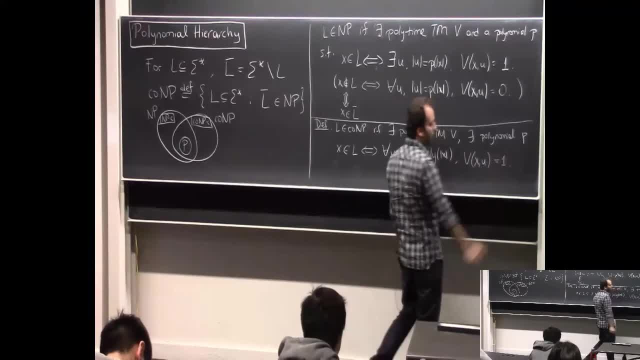 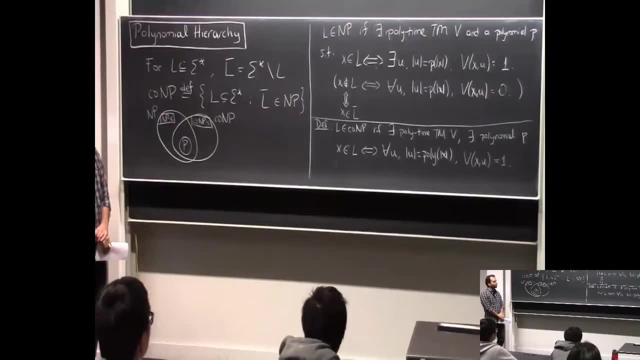 I'm going to change here the meaning of 0 and 1 and put a 1 there. It doesn't matter, It doesn't make the definition any different. OK, if I change the true to false and false to true. OK, so there are various ways to think about co-MP. OK. 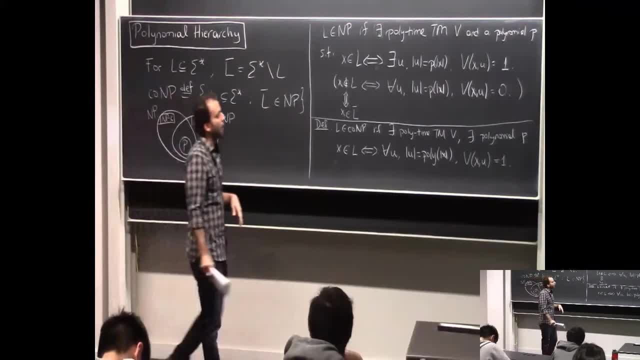 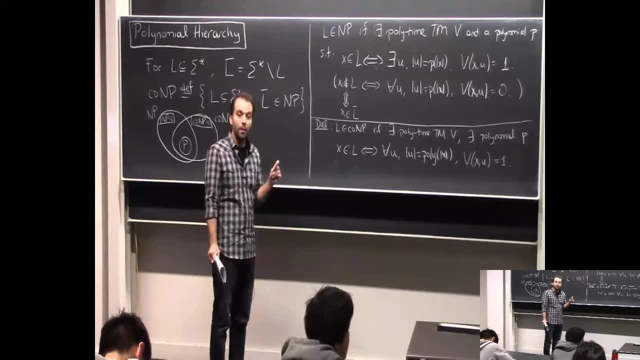 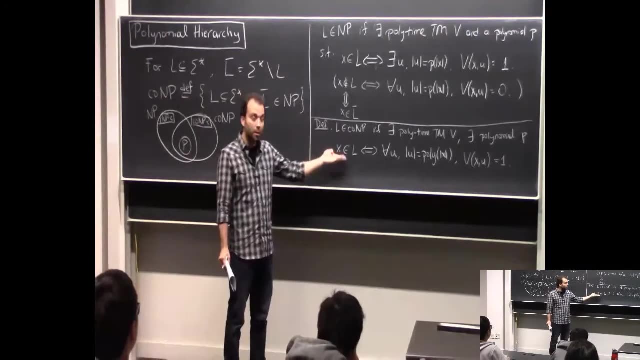 So one way to just define it this way. Another way is like: OK, co-MP is the class of languages where you can verify no instances efficiently. Or you can say it in this way, where you say: oh, the yes instances. a yes instance is a yes instance. 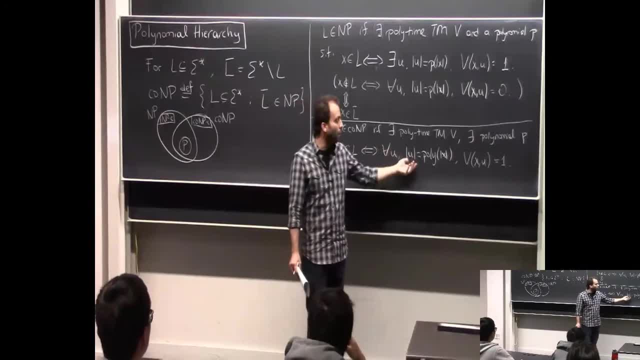 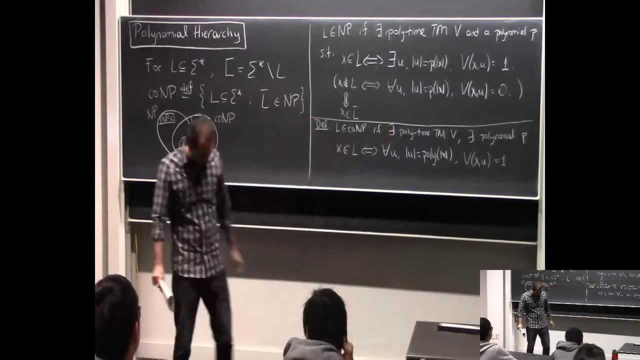 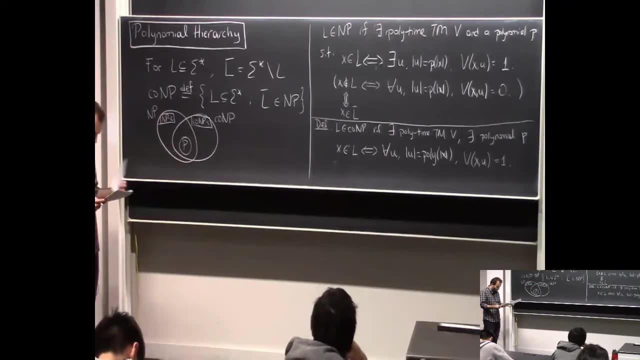 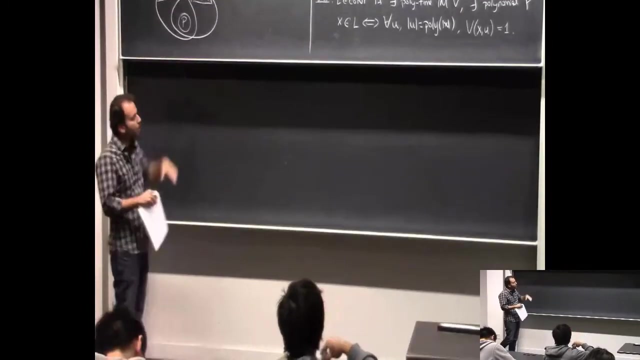 if, and only if, for all u where the u is polyominal length, vx u. there is this: verify where vx u outputs 1.. OK, so all right, All right, And now let's put this up here. So one thing. I'll make a quick observation. 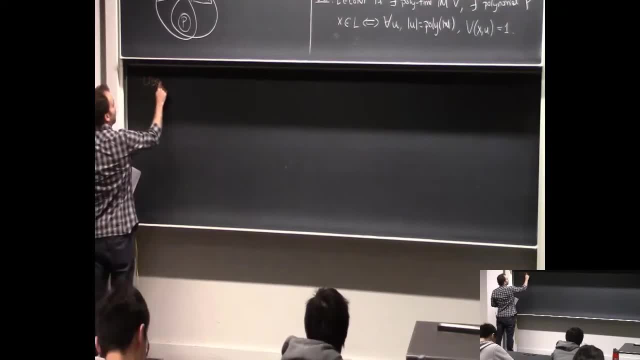 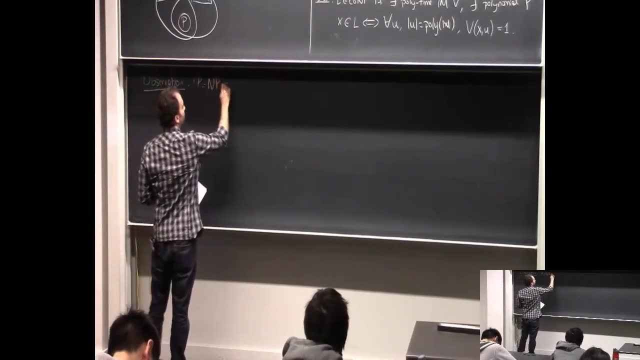 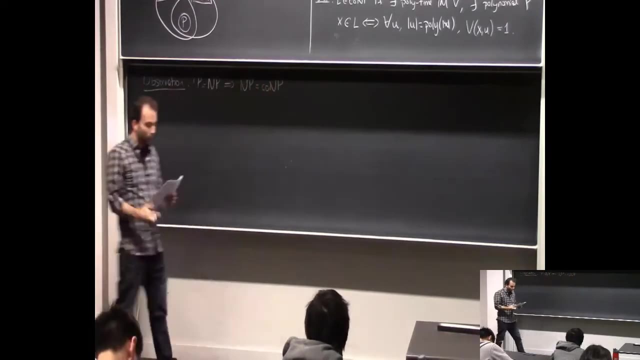 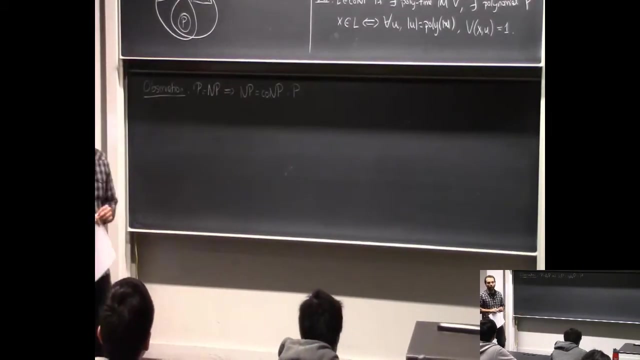 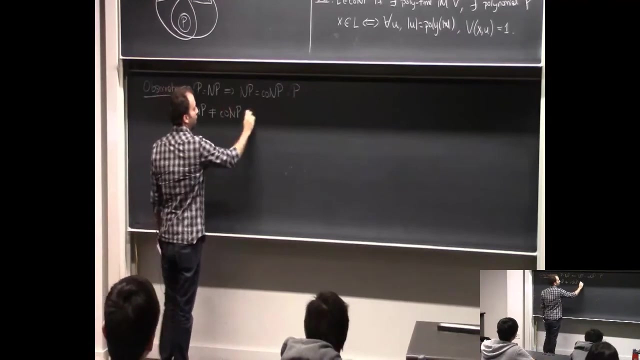 a very simple observation. So P equals MP implies NP equals co-MP. OK, and well, that's also equal to P. So why is that the case? Can someone tell me why? P equals MP implies MP equals co-MP. By the way, this equivalent saying that MP not equal to co-MP. 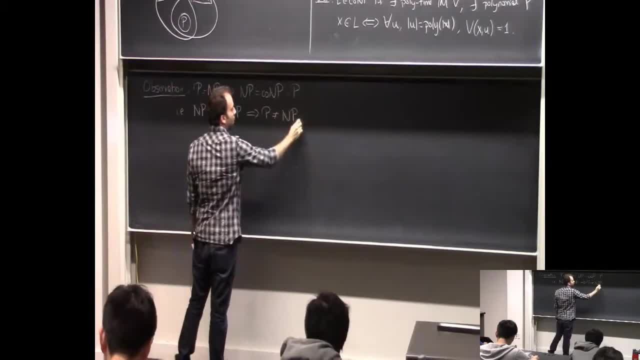 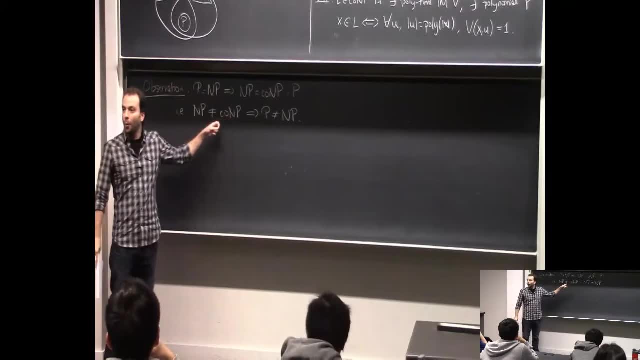 implies P not equal to co-MP. OK, Not equal to MP. So in case you were working on separating MP from co-MP, you should know that that implies P is different from MP. So why is this the case? Well, P is equal to MP. 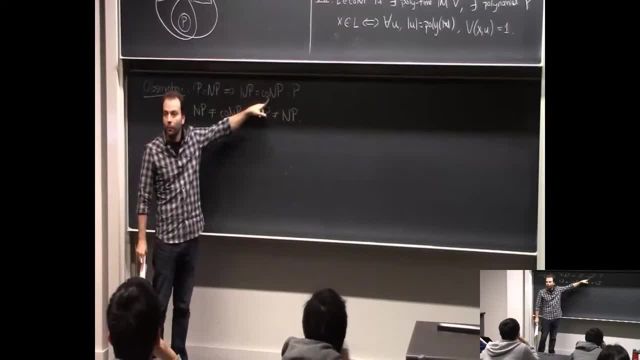 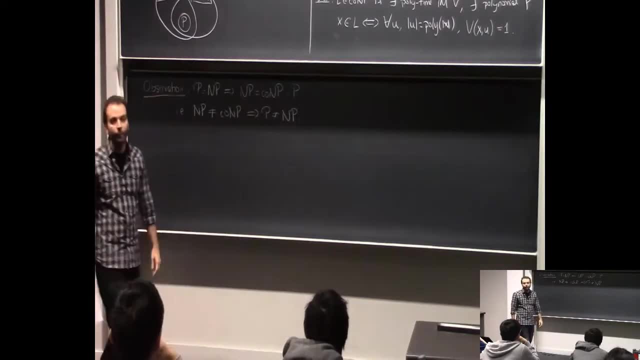 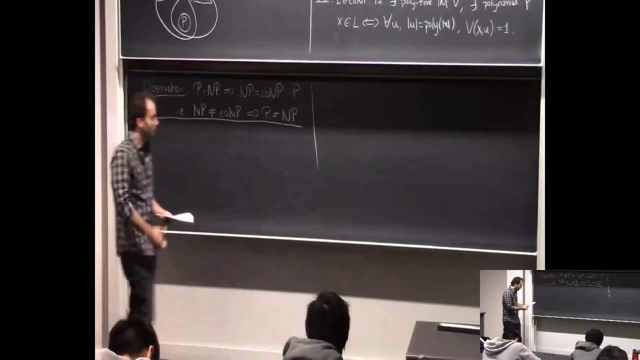 Then co-MP is equal to co-P. But what is co-P? Co-P is P OK. Take the negation of a language in P, you get something in P OK. so that's just a small observation. We might need it later. 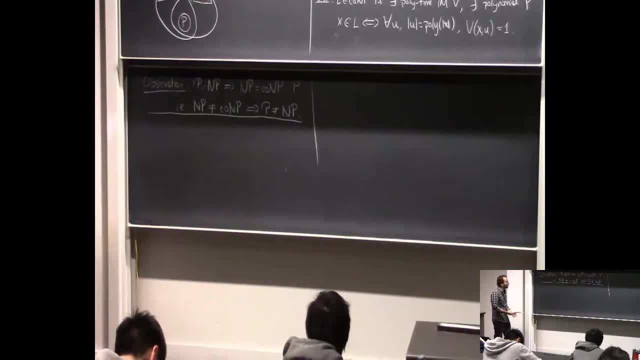 OK. so now, fine, we have this class MP, We have this class co-MP. Let me now define a language for you And let's see if it falls in MP or co-MP. So this language I'm going to call E-click. 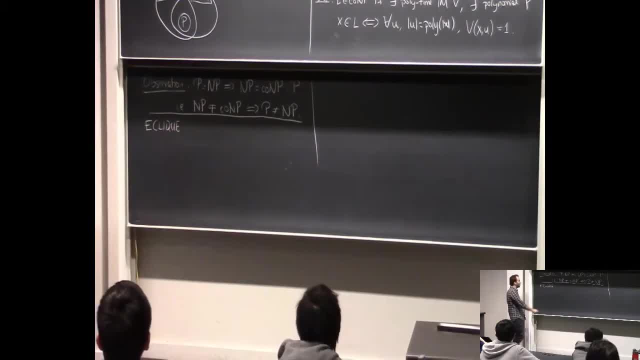 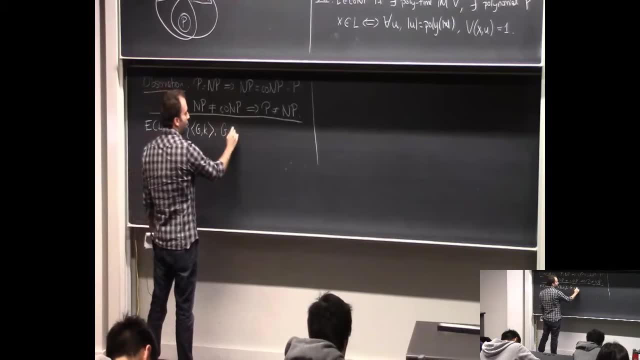 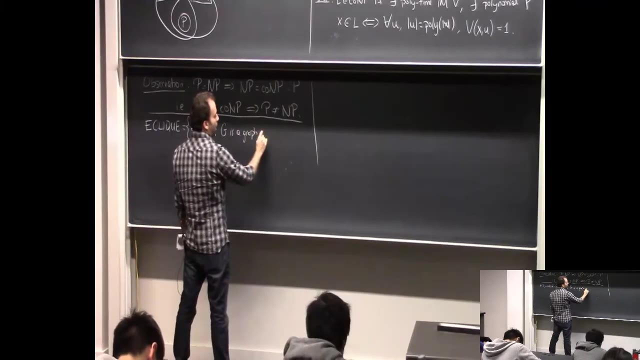 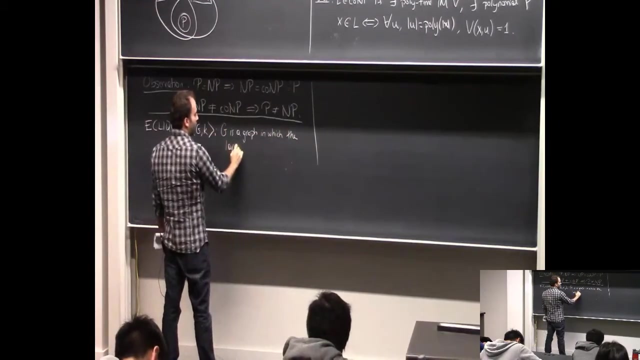 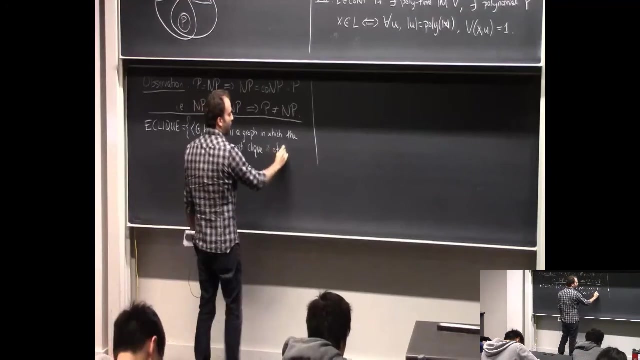 E stands for exact, exact click language, So this is the language of work. This is the words G, K, where G is a graph in which the largest click, the largest click, is of size K. OK, and when I say K, I 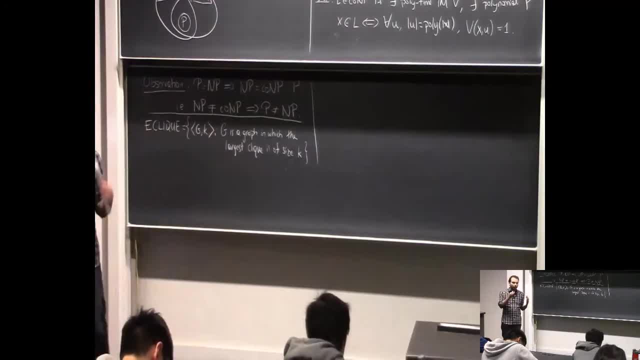 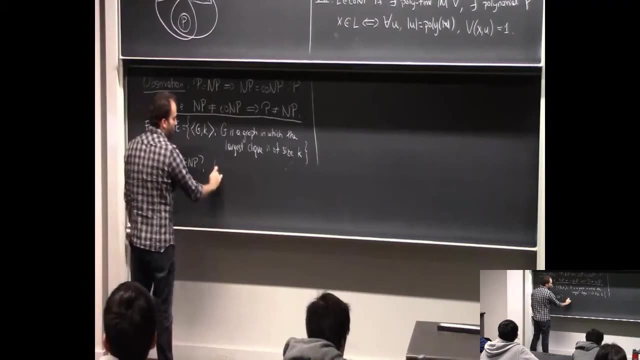 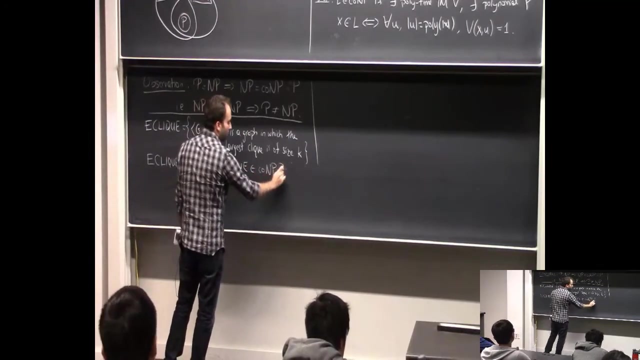 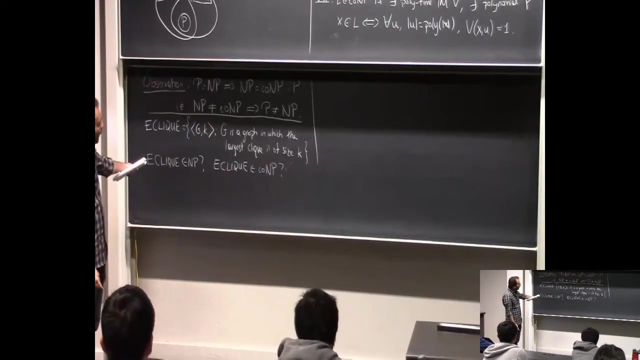 mean exactly K. The largest click has size, exactly K. So let me ask you now: is E-click in MP, Is E-click in co-MP? So how would you define E-click? How would you, how would you prove that a graph's largest click is of size exactly? 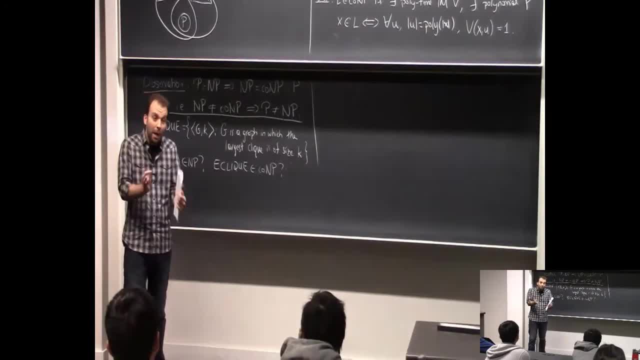 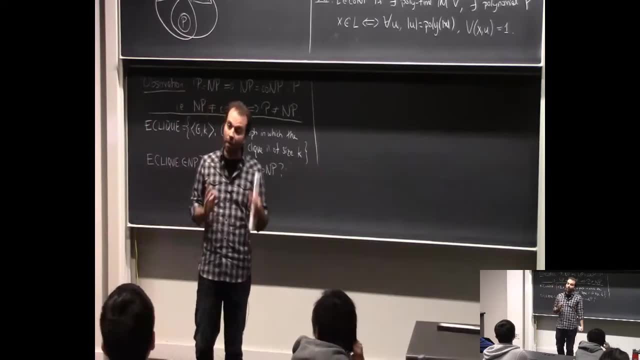 K. Now you could say, OK, I'm going to give you as proof a click of size K And then, fine, I can check that. I can say, yes, this graph does have a click of size K, But that does not prove to me that. 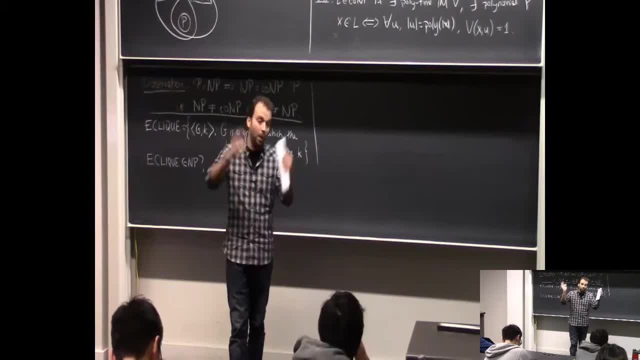 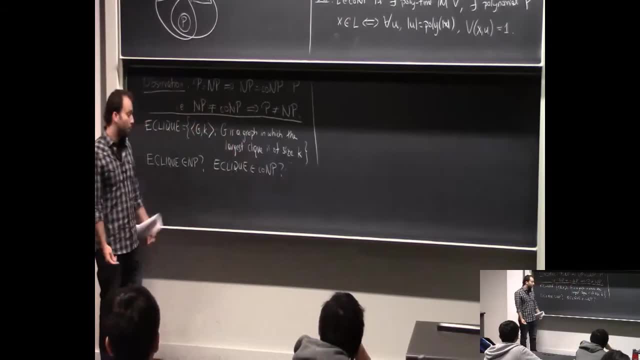 the largest click is of size exactly K. There could be maybe a bigger click. You haven't proved that to me. OK, So that doesn't work And you can try other things. I don't think you'll be successful. You can also think about: oh, can I put it in co-MP. 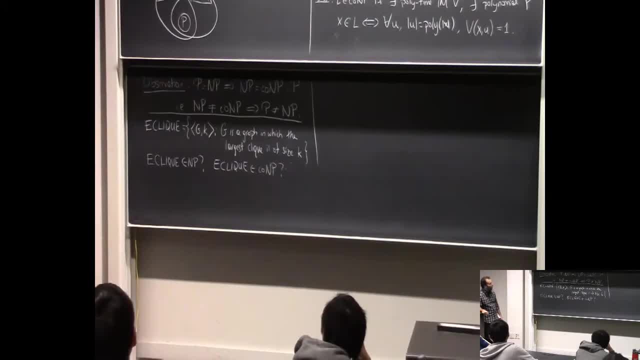 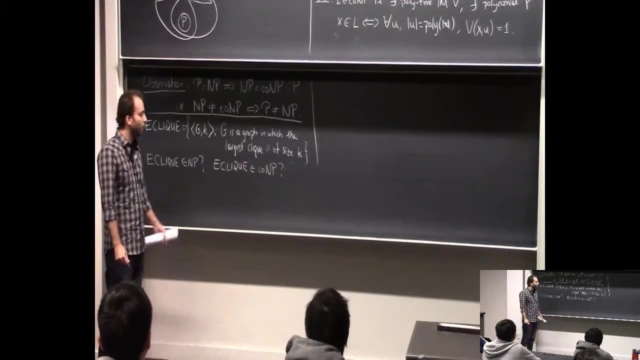 Is it like, naturally, in co-MP, How do I show that the largest click is not of size K, Right, So you're going to, you're going to run into trouble. I mean, that's kind of the point of this example anyway. 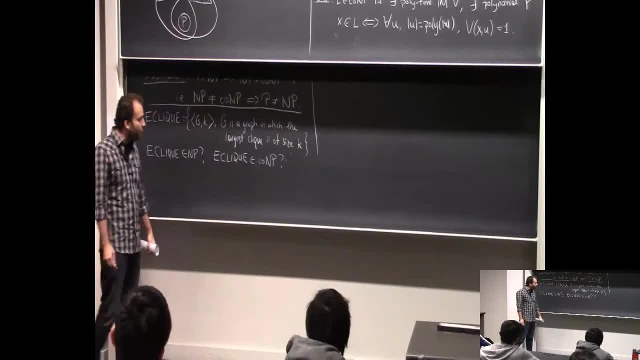 But. But yeah, I mean, what's the natural description? if I were to like write this in some sense like in English? So I would say: well, a tuple is going to be an E-click if there exists some set set. 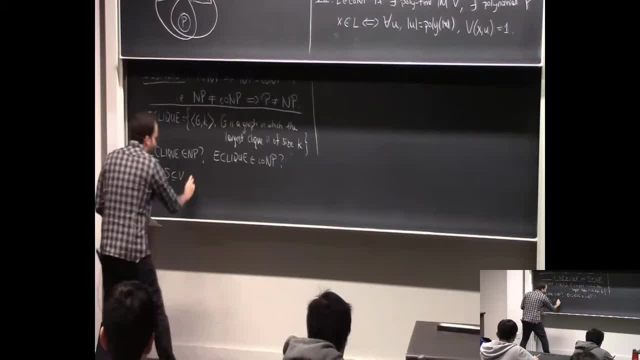 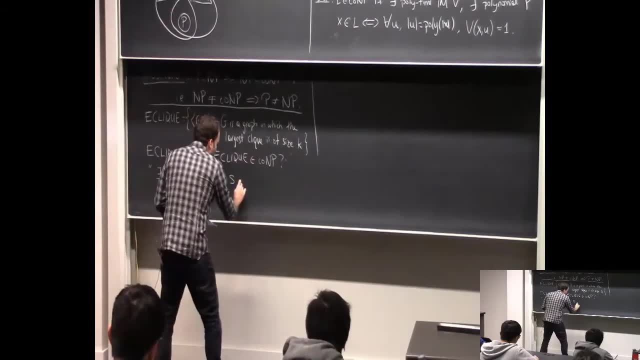 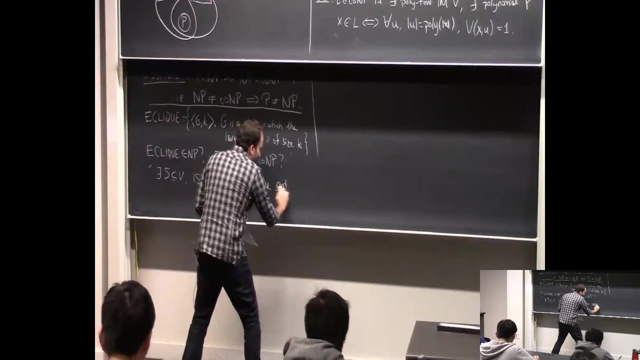 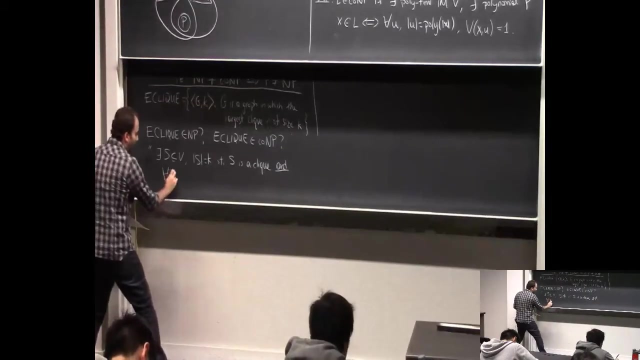 of vertices S and V, where the size of S is K, such that S is a click If X forms a click. And not only that, but and for let me write it here for all, S, prime subset of the vertices. 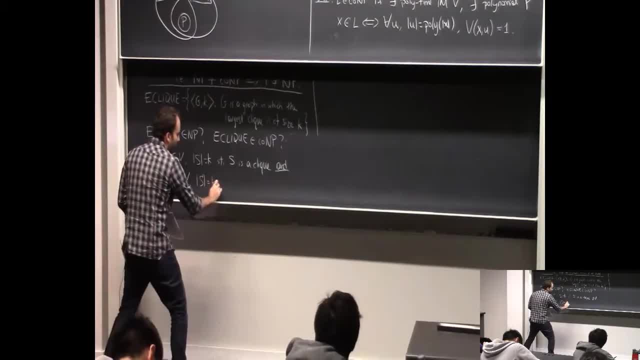 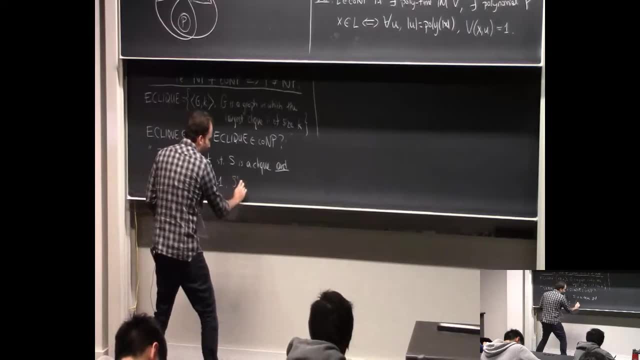 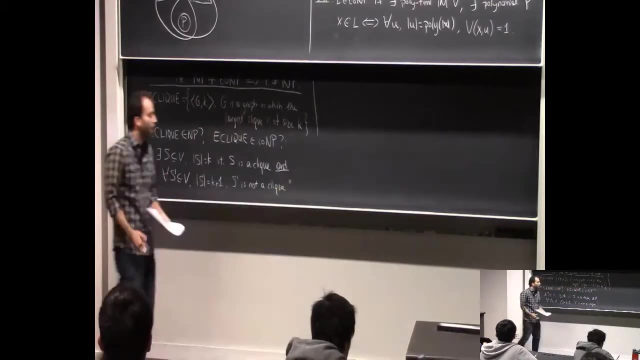 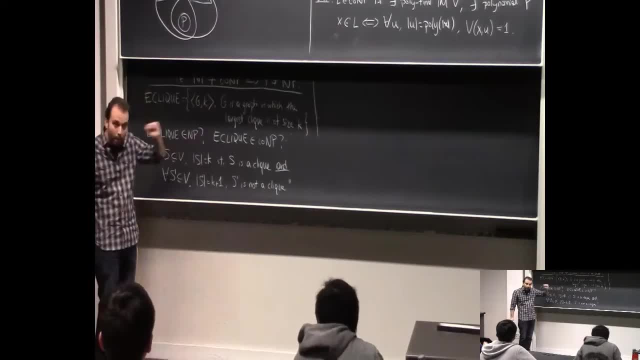 You know you want a click of size K, but at the same time, for all subset of vertices of size K plus 1, they should not form a click. So then in that case you would know: great then my largest click of size K. 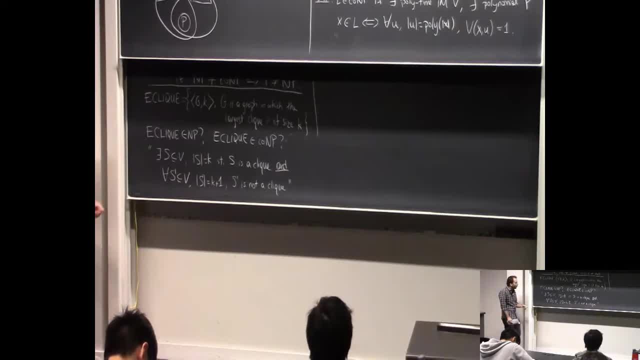 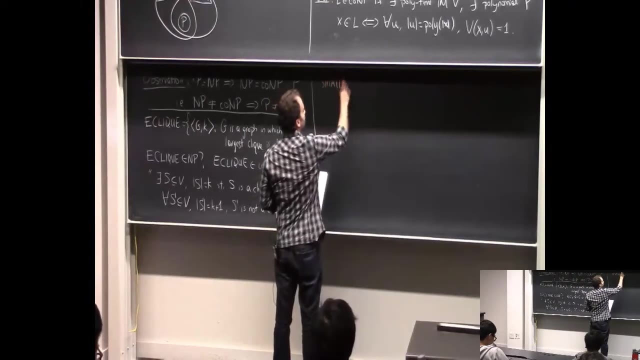 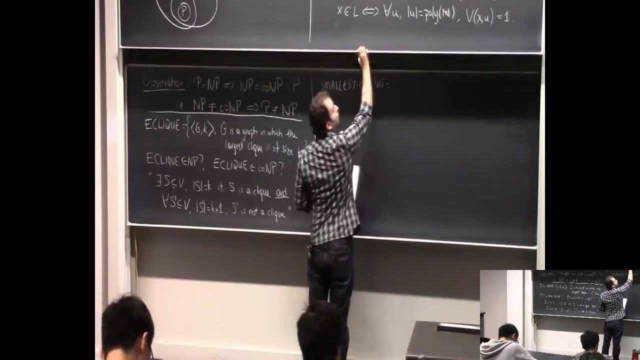 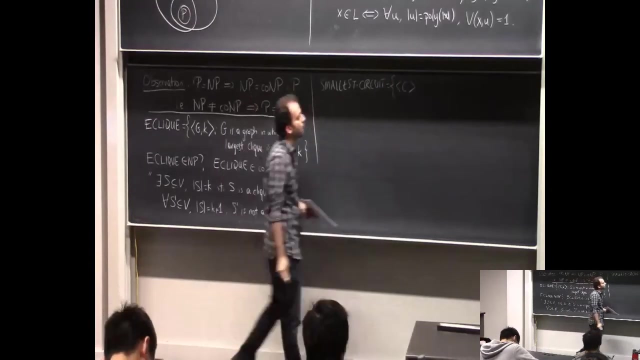 But what I like to emphasize here is the number of quantifiers there exists, plus there's a for all. Okay, Now let me give you another example: Smallest circuit- So this is the language- that consists of Boolean circuits such that C is. 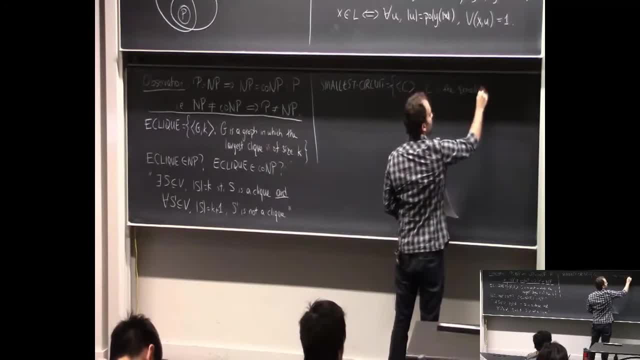 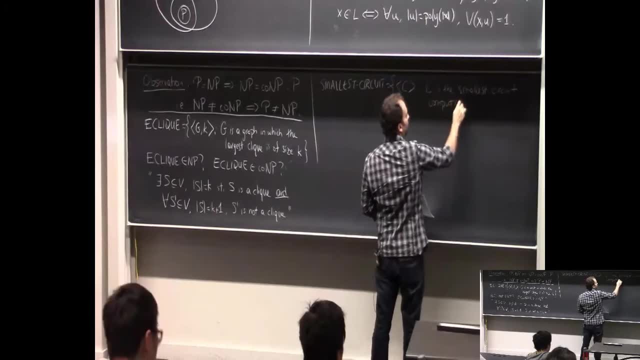 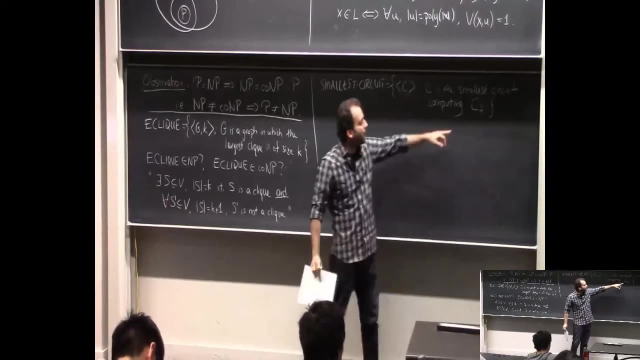 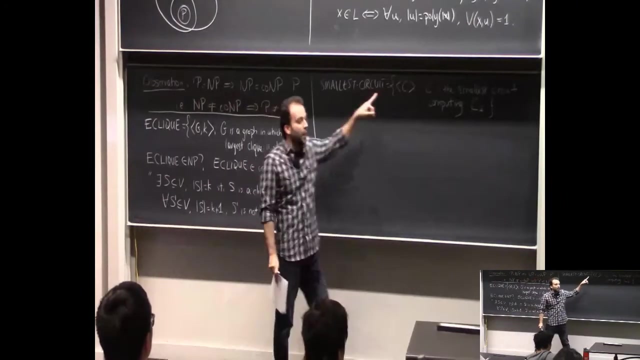 the smallest circuit computing. let's call it the function that C computes. Okay, So by C sub F I mean the function that C computes. Every Boolean circuit computes some function, Some function it computes, And I want C to be such that there's no other. 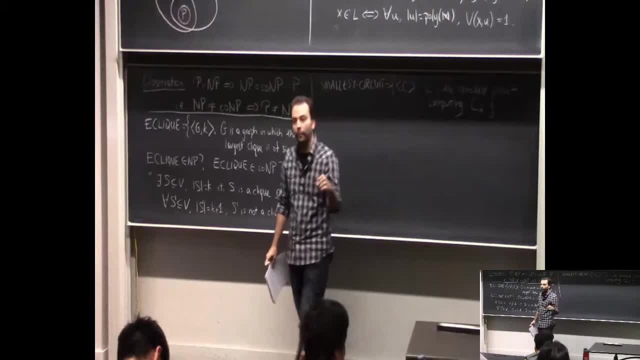 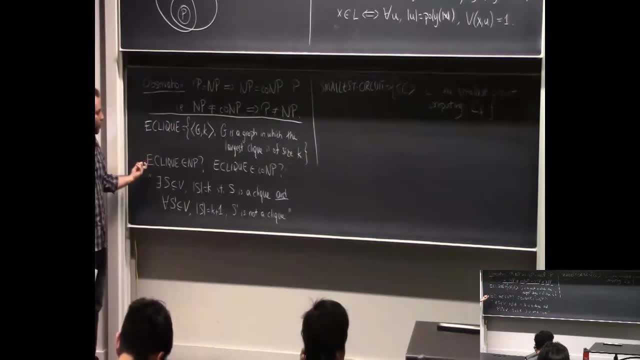 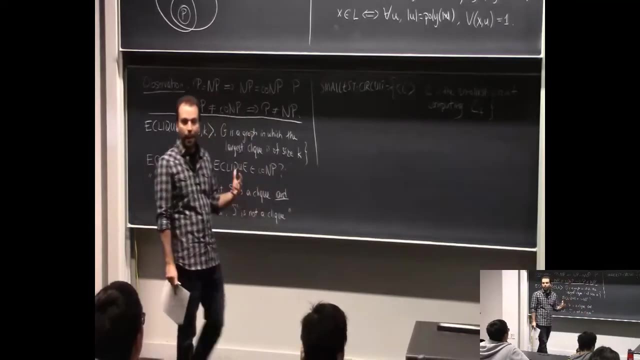 circuit smaller than C that computes that same function. Okay, So this is the smallest circuit. And again I can ask, like you know, is smallest circuit in MP or is smallest circuit in co-MP? And you can think about it and you won't be able to put it naturally in MP or co-MP. 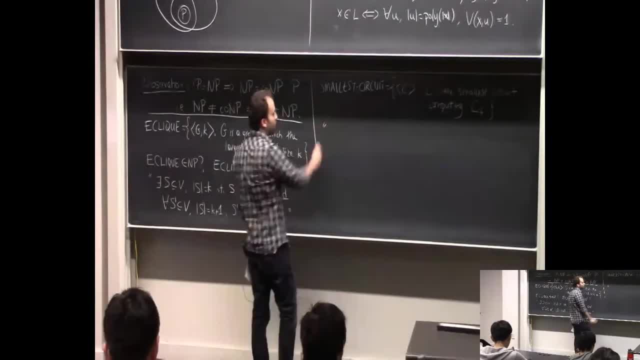 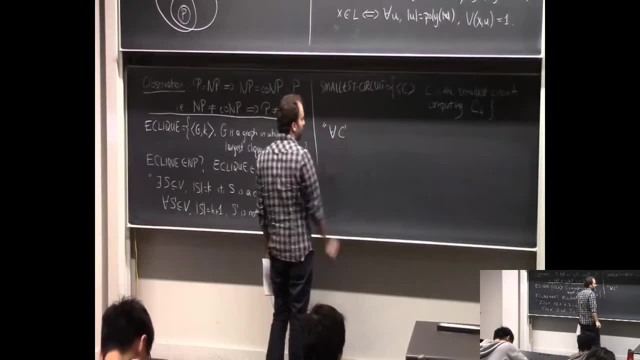 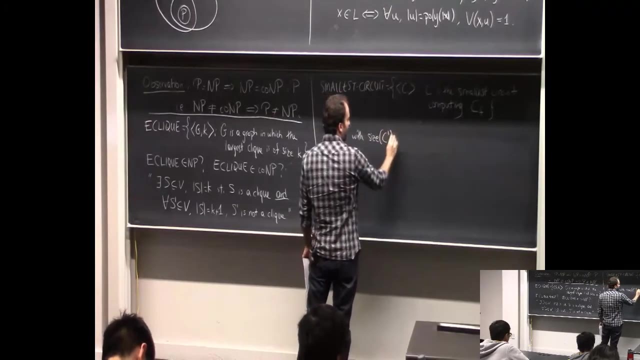 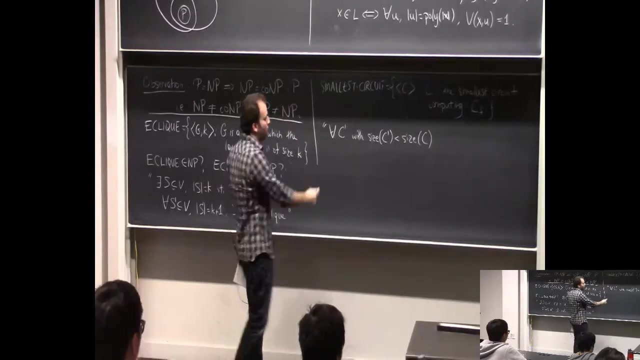 And here again let me add, like an English description to this one as well. So here it's more like for all C prime circuit C with size of C prime is less than size of C. What do I want? Maybe you can complete it. 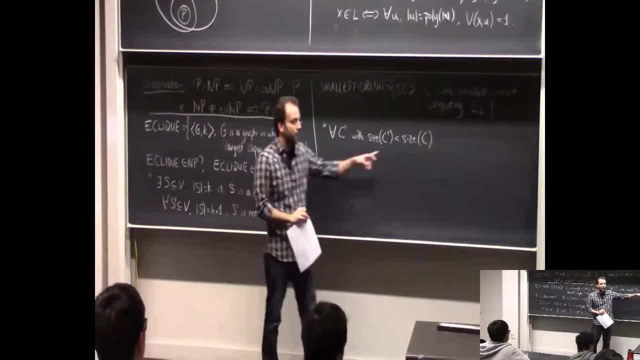 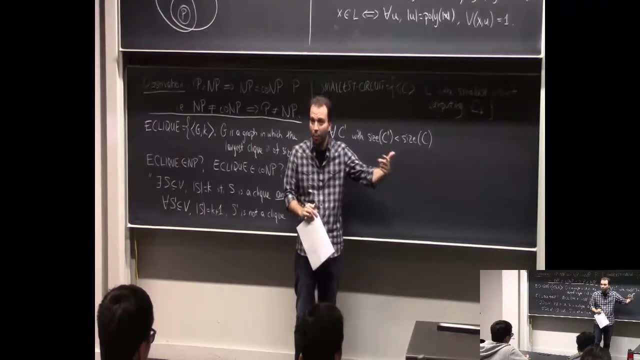 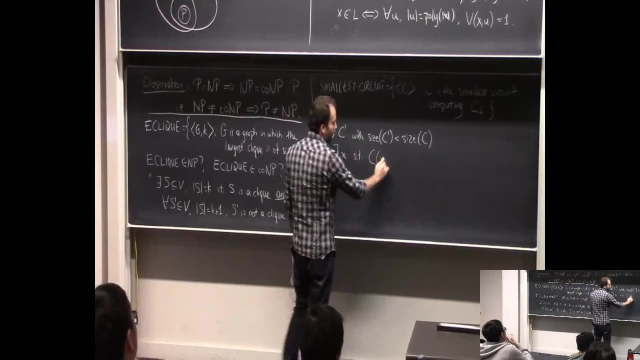 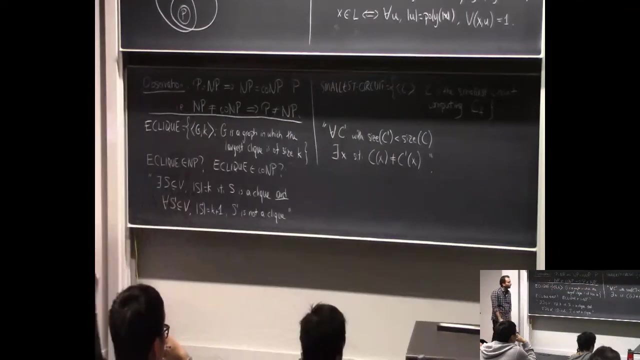 For all circuits smaller than C prime. I wanted not to compute the same function as C does, so it should disagree with C in some place. So there exists some is some x, such that c of x is different from c prime of x. Again, for all there exists. 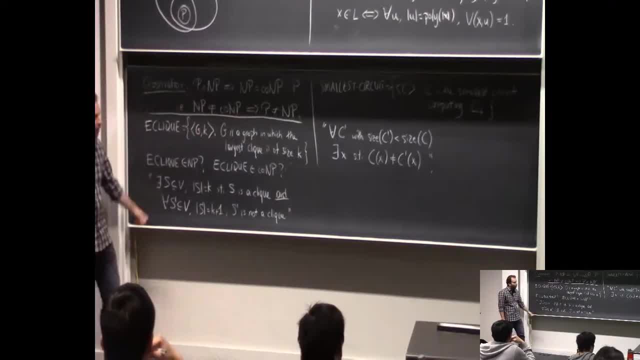 Two quantifiers Here we had. there exists for all. This is for all there exists. And now? okay, so, as you can see, it's kind of suggesting like maybe we should come up with a new complexity class to capture these problems. 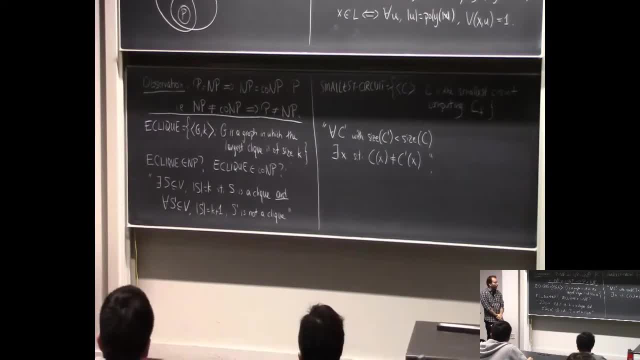 These are natural problems, right? These are not like very funky problems. These are very natural problems. They don't naturally fall in MP or co-MP. What's a natural class that we can put these class languages in? Okay, So this is one motivation for it. 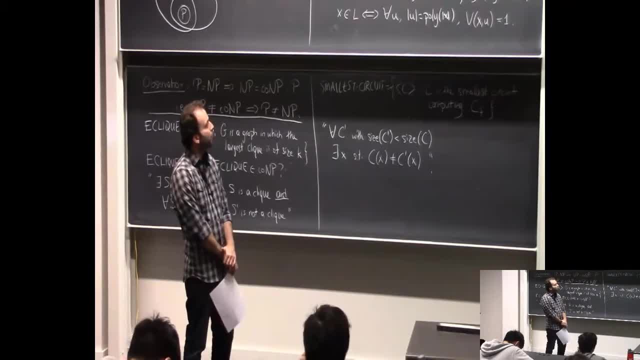 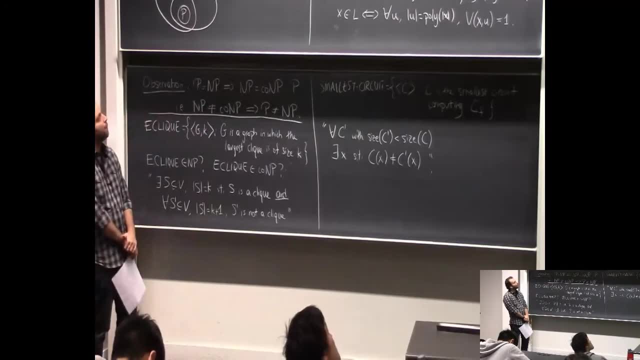 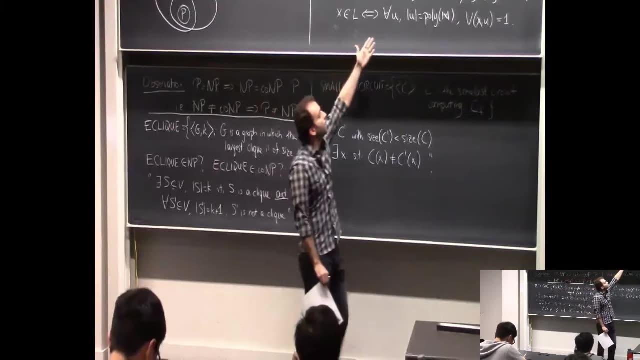 I mean also, like you know, if you imagine, like you're a researcher in the mid-20th century and you have, like, this definition of MP and this definition of co-MP, it's kind of natural to ask like, well, you know, these have one quantifiers. 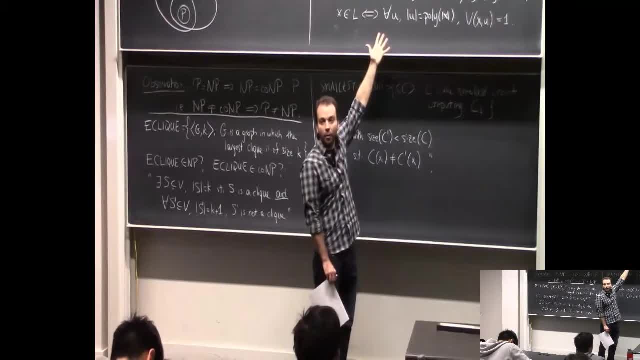 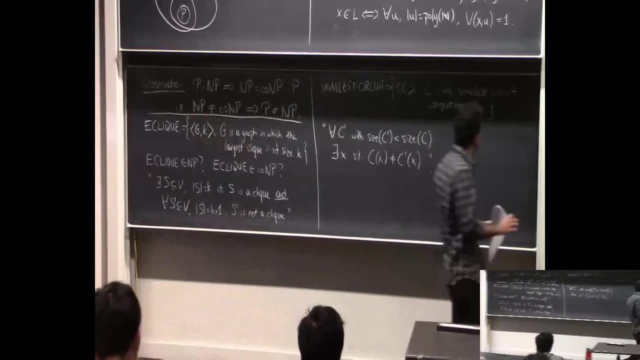 What if I add more quantifiers- A very natural thing to generalize in that way, right And see what kind of thing you get. Okay, So let me do that now. So let me actually add a little notation here that I will use throughout. 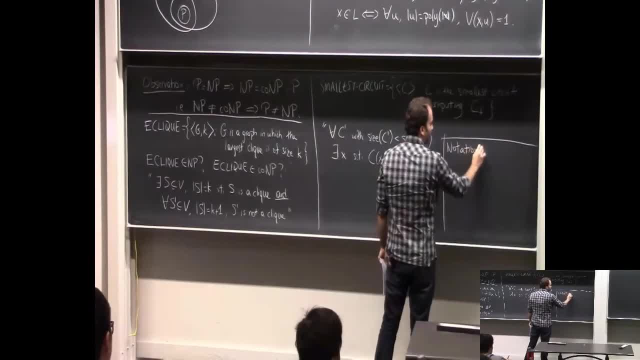 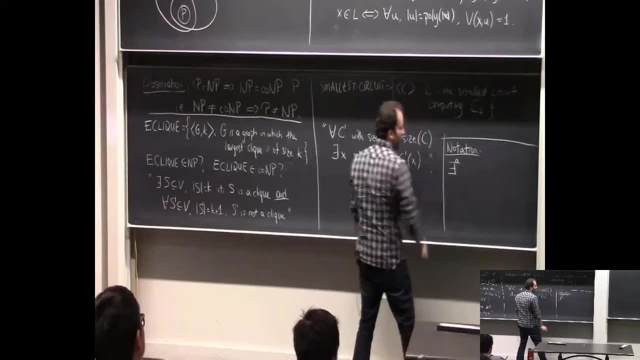 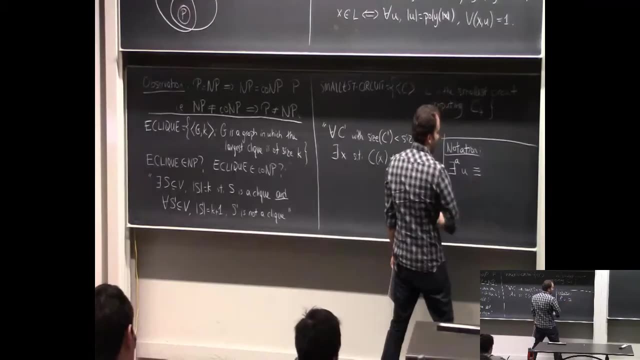 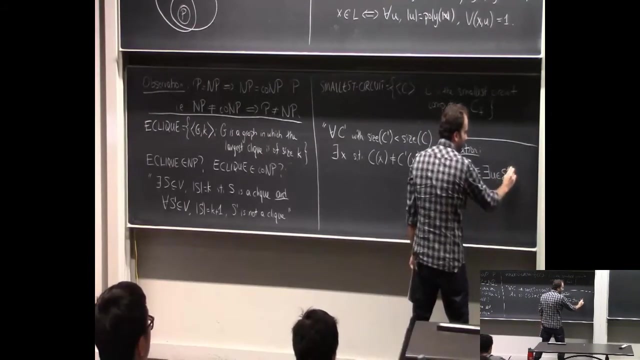 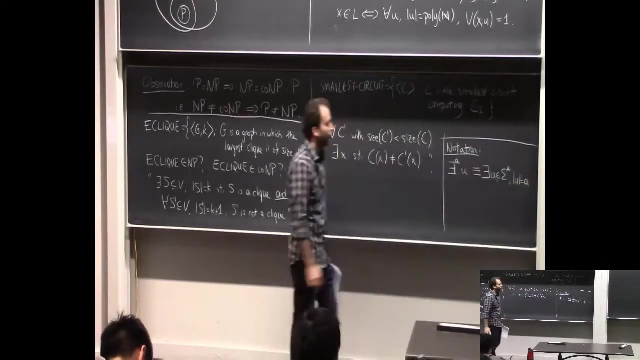 Notation. So I will write there exists, with like a superscript and then some variable, u. This is going to mean there exists u where you know where u is in sigma star and the size of u is exactly A. Okay, So when I use this notation, there exists a u, I mean there exists a u. 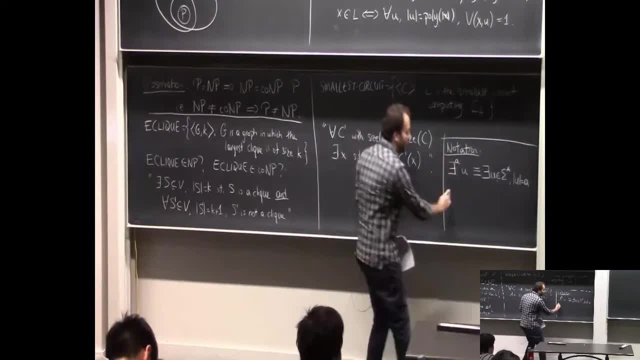 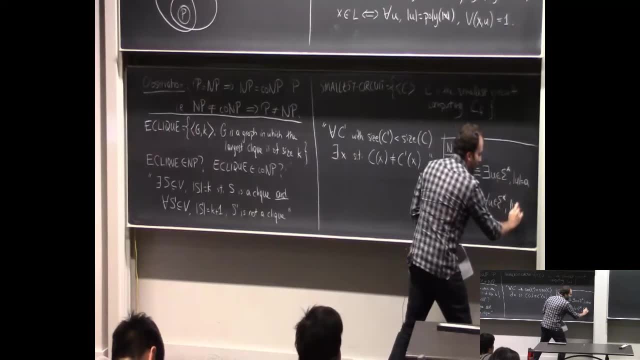 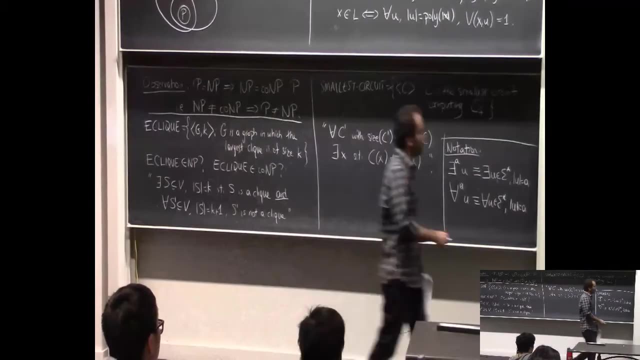 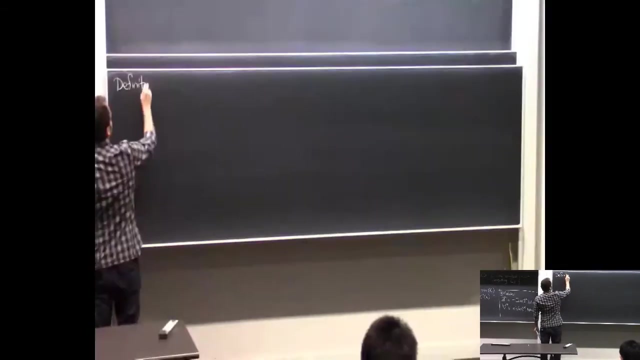 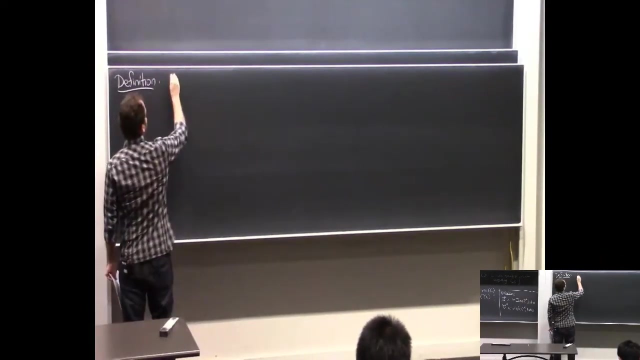 in sigma star, whose length is exactly A. Similarly, for all a u, this means: for all u in sigma star, with u equals A. Okay, So now let me define u, This complex, this complexity class that captures these problems. So we're going to say that L is in. 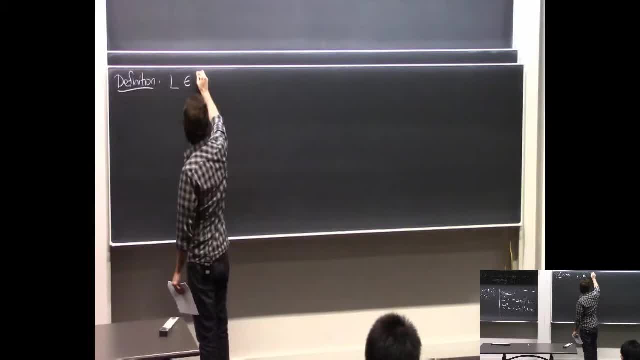 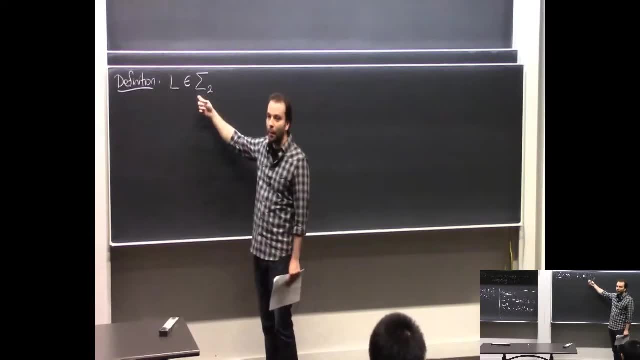 So he is an unfortunate class in notation. So this is going to be called sigma 2.. So this sigma is not the same as the alphabet sigma 3.. okay, but it's the way it's used. so unfortunately, I have to use Sigma. so 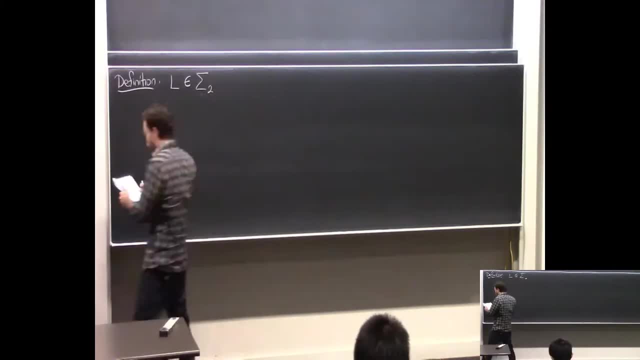 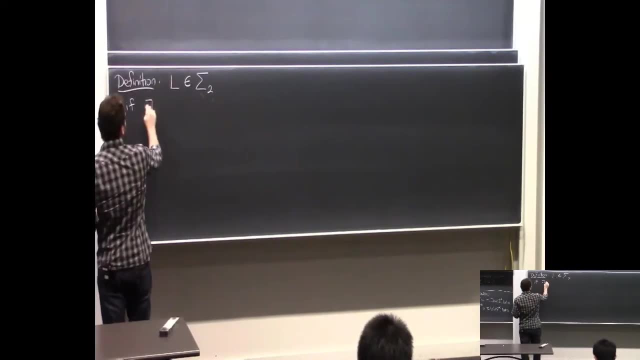 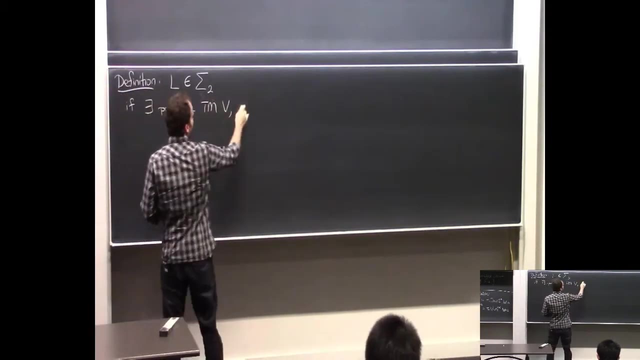 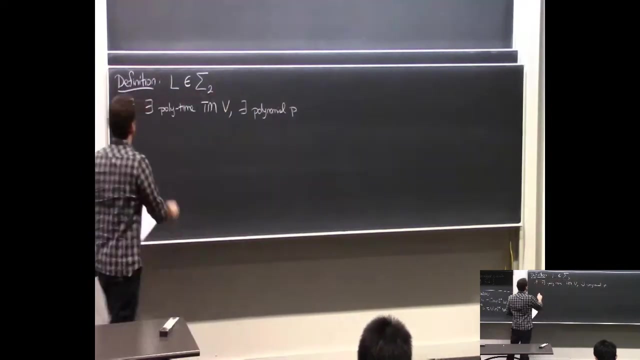 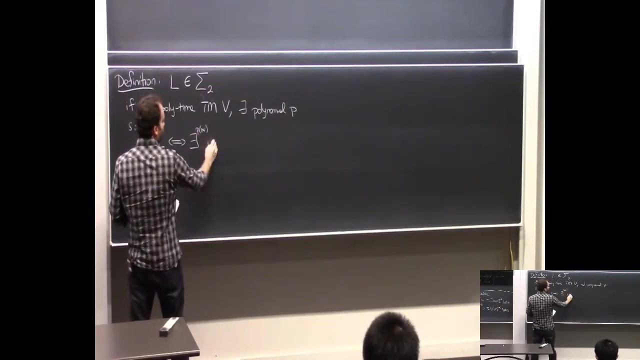 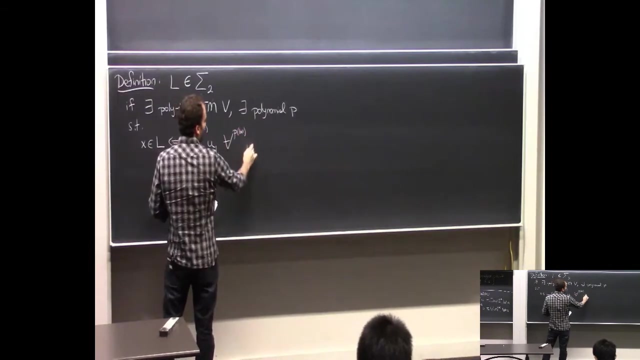 L is in Sigma 2, if there exists a polytime Turing machine, V, there exists a polynomial P, such that X is in the language. if, and only if there exists with the polynomial length u, u1, actually for all polynomial length, u2, V, V, V, V. 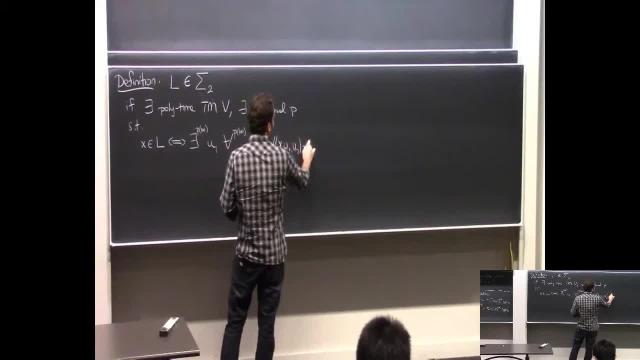 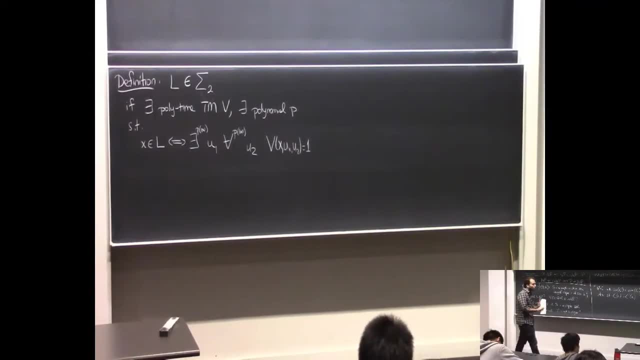 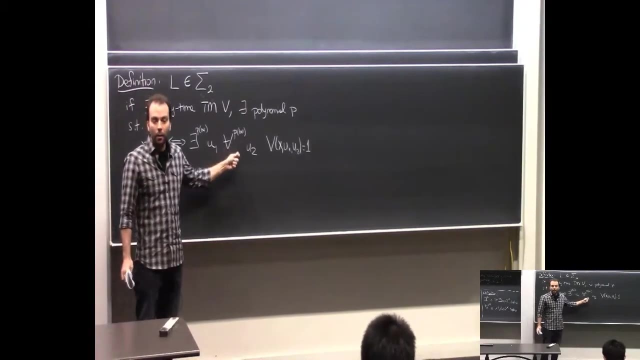 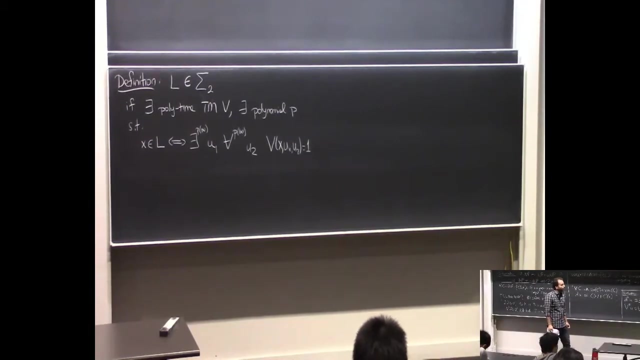 X, u1. u2 equals 1. okay, so I took the definition of MP, I added one more quantifier, I made it, I added a for all. okay, and actually I will stay like a color chalk here somewhere, not really okay, it doesn't matter. so I'll actually into this definition, add another. 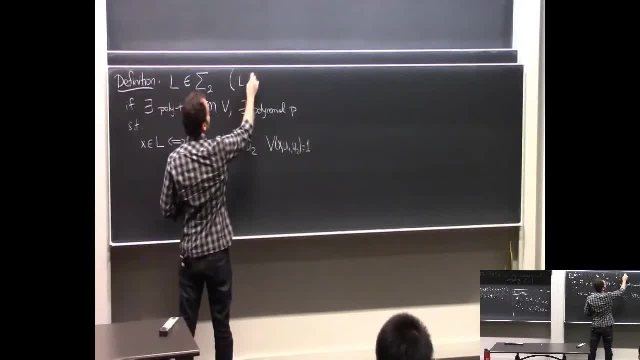 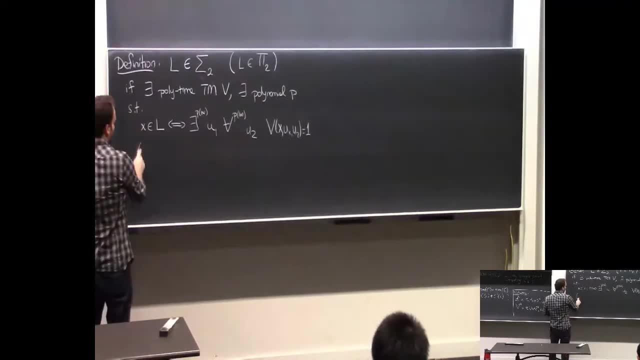 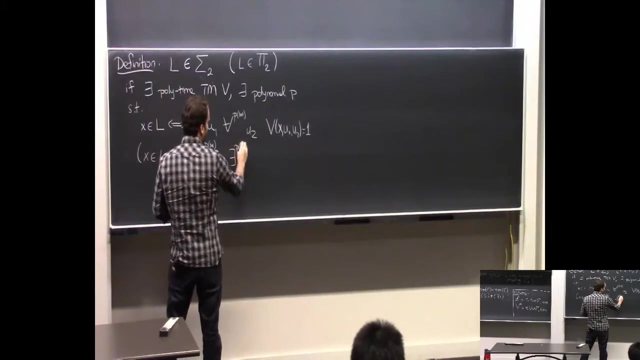 definition. so I'll put that is in parentheses. so I'll say that L is in PI to if, the same thing. but now the condition is that X is in L if and only F for all it. now it starts with the for all quantifier, For all u1,, there exists u2, and the rest is the same. 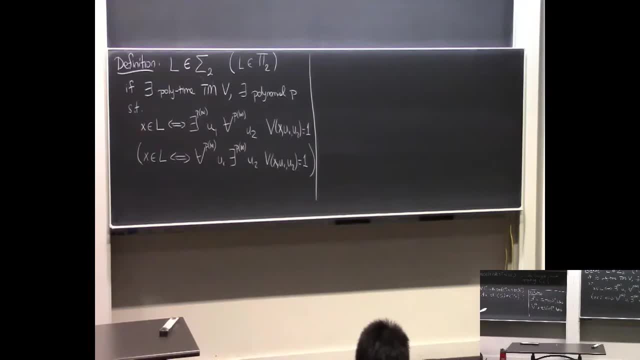 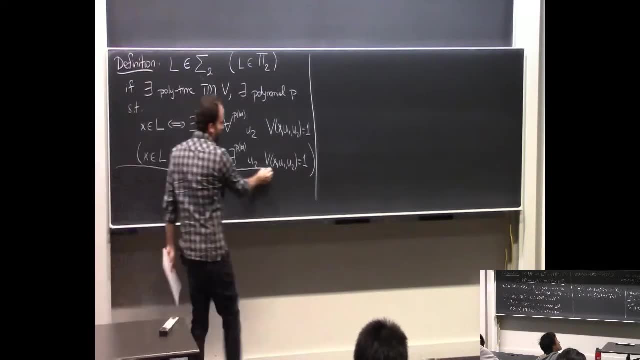 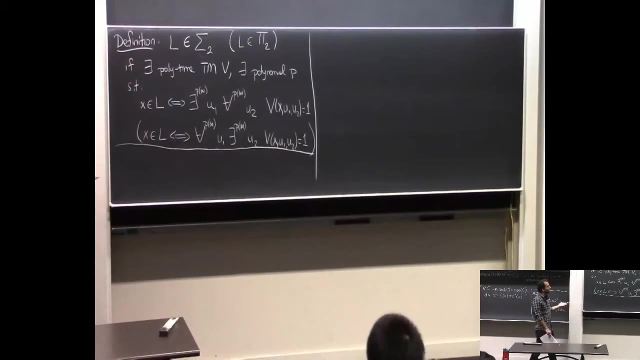 Okay, So the definition should be more or less clear. I mean, it's very similar, as you can see, to mp and co-mp. It's just one more quantifier. I'll make a little observation here. Observation pi 2 is actually co-sigma 2,. 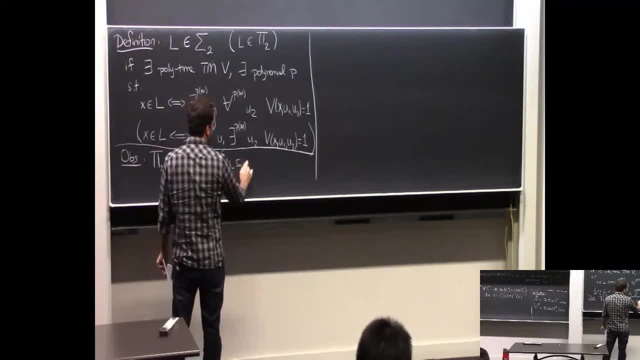 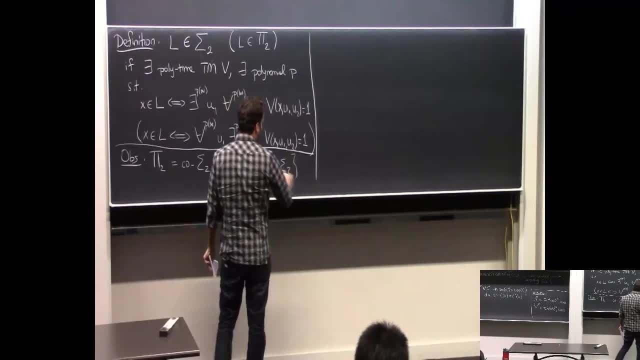 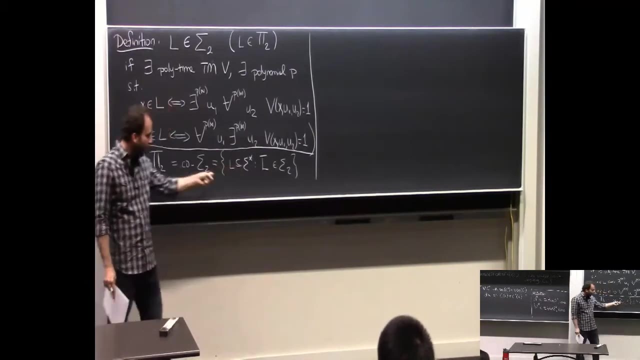 which we would define as all those, all those languages, such that the complement is in sigma 2.. Again, I apologize for the notation. Like this, sigma is not the same as the sigma, They're different, You might ask. why do you think you know there's a sigma here? 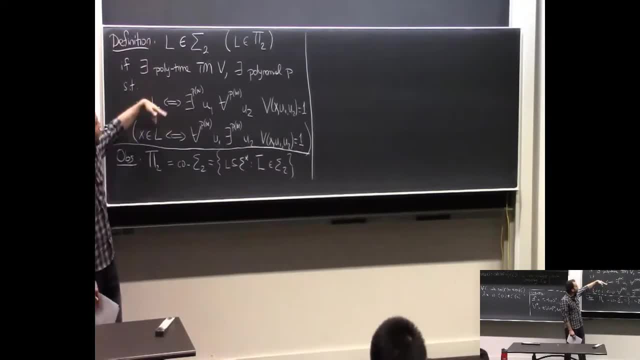 Like: why do we use this notation? So yeah, I mean you think of this as like: okay, it starts with a there exists. There exists is usually, you know, a sort of a you know, you know. 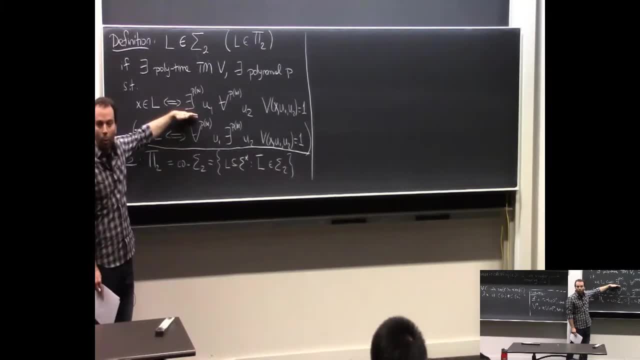 there exists, is usually associated with, or taking an or and or is usually associated with a sum. Okay, And then the other one, pi is like. well, this starts with for all. For all is associated with a product or ands. 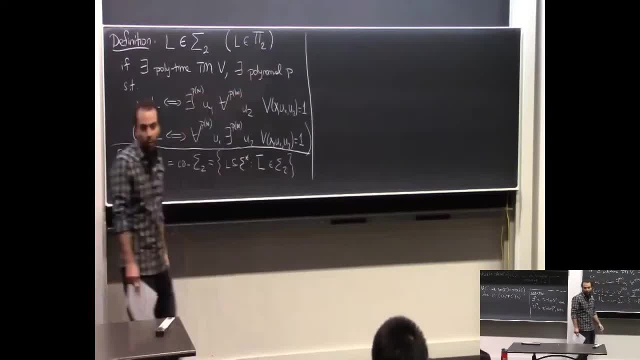 and this is a product, So that's the product there, product notation, So that's one way to remember which one is which You look at, which quantifier it starts with. There exists for all, And yeah, this is like an observation. 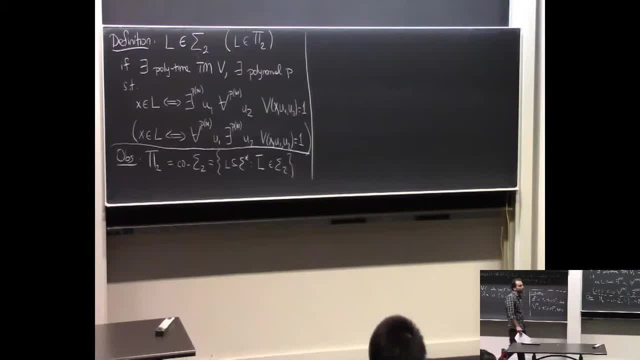 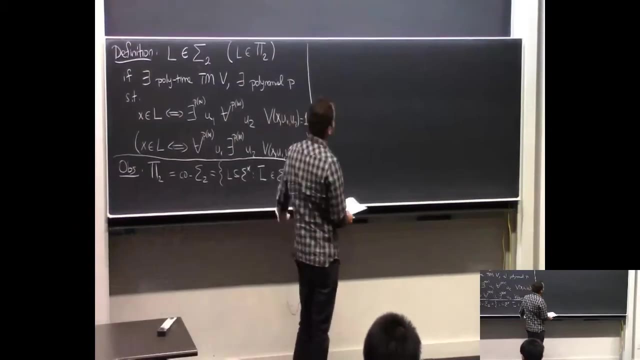 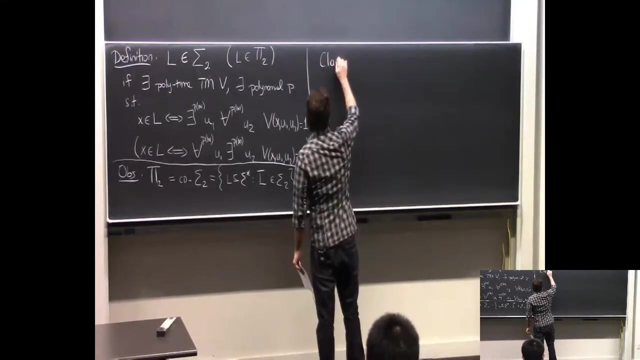 I mean you can. you should be able to see that I'm not going to waste too much time on this. But yeah, so pi 2 is co of sigma 2.. And now I claim: yeah, so claim, claim that this guy E clique. 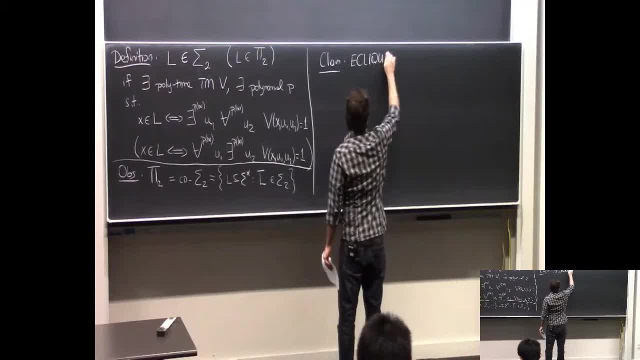 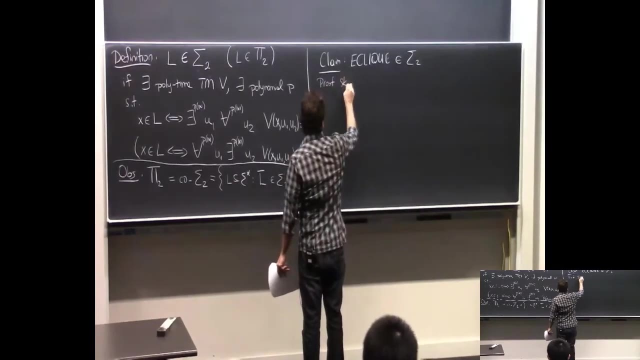 let's say, Is in sigma 2.. Okay, So let me give you the proof, idea here, Proof, you know, sketch if you want, or idea. So when you want to show E clique is in sigma 2, well, 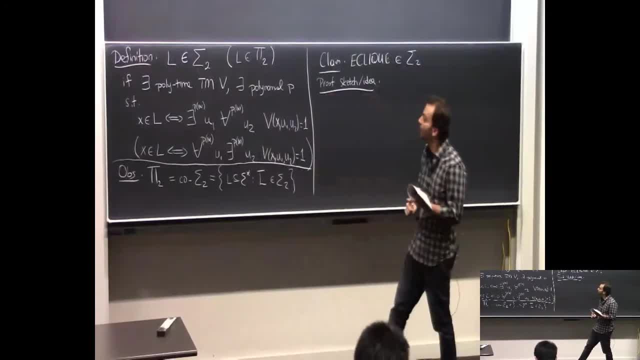 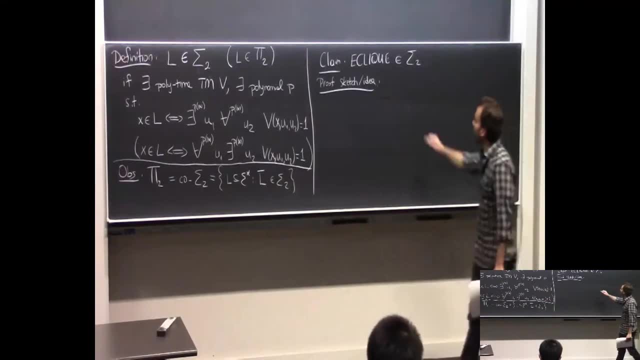 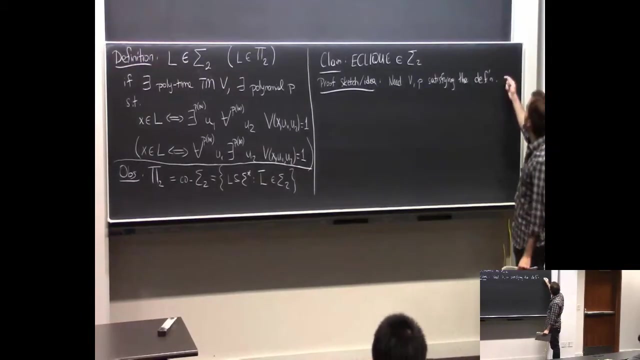 you go to your definition and say, okay, I need to come up with a verifier, V, polynomial P, such that this is satisfied. So need V and P satisfying the definition. Okay, So the P is going to be like: you can basically pick P. 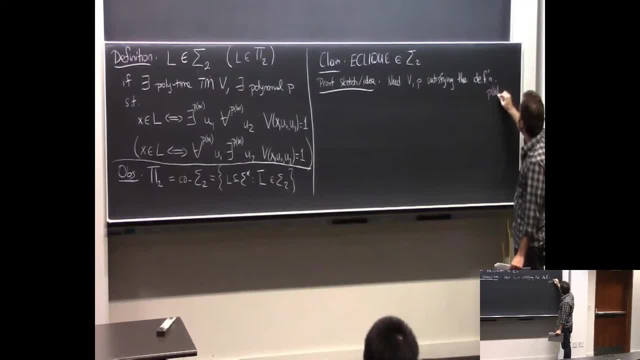 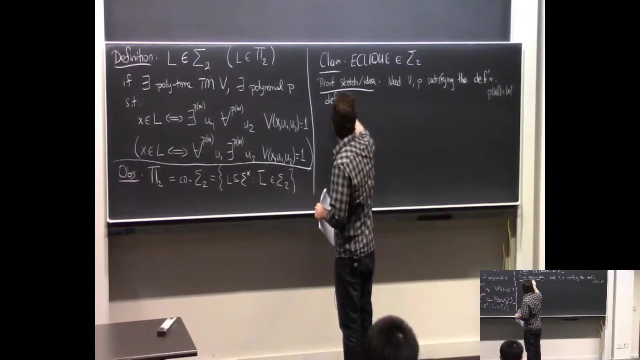 to be Like linear. That should do the trick. You don't need P to be too long And yeah, let me see if I can. yeah, let's, let me try to squeeze in the verifier here. So def. so this is the verifier V. It takes X, U1,, U2.. 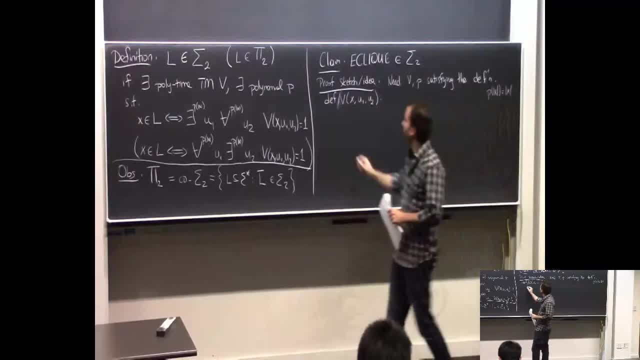 Okay, So this is the verifier V. It takes X, U1, U2.. Okay, So this is the verifier V. It takes X, U1, U2.. Okay, And step one is what? How do we, how do we do this kind of thing in a 251?? 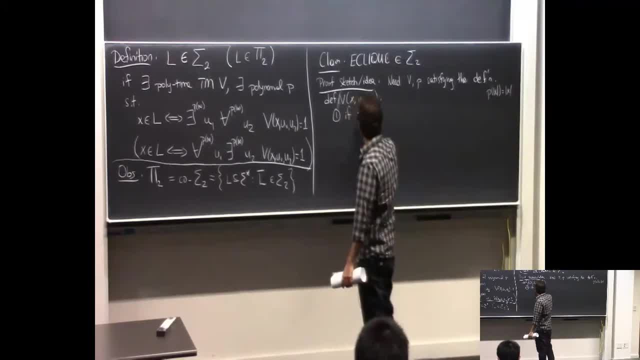 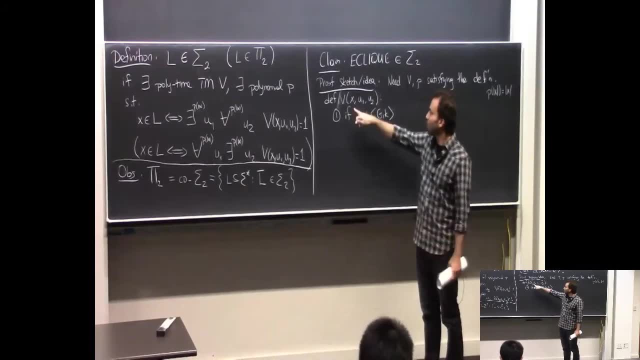 Check for a valid. So if X is not equal to GK, if X does not equal, So here X, U1,, U2, these are arbitrary strings. So if X is not equal to GK, if X does not equal, So here X, U1,, U2, these are arbitrary strings. 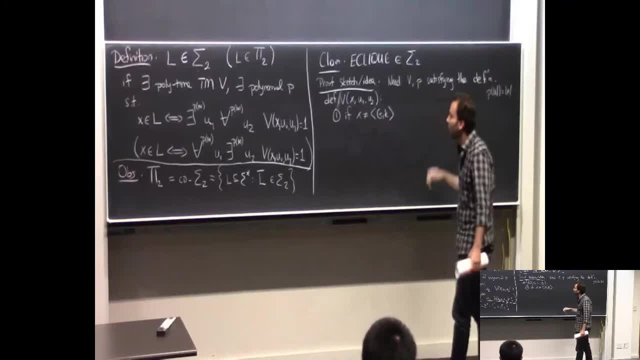 So if X is not equal to GK, if X does not equal, So here X, U1,, U2,, these are arbitrary strings. If X, first of all, is not like a valid encoding, then you're, you should just reject. 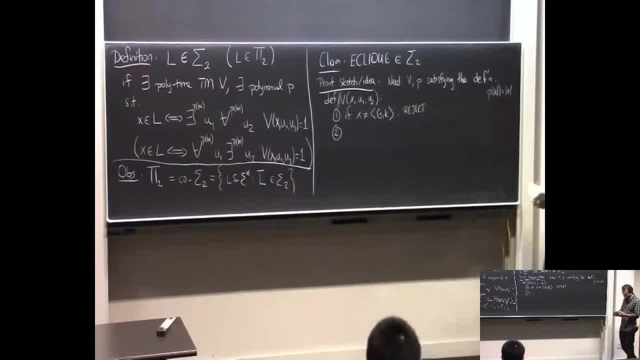 Okay, So then we have a valid encoding, a valid instance. Then what do I want? If so, I'll just say this, because you know, the first time you see it it may not be, it may not come natural to you. 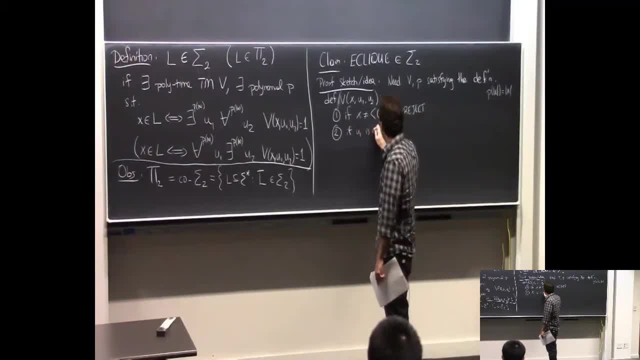 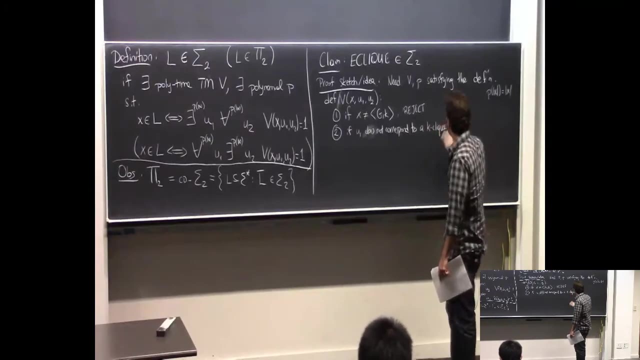 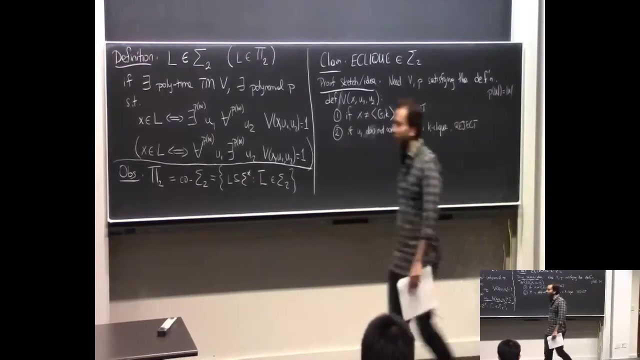 But yeah. so if U1 is not or does not correspond to a K-click in the graph G, then reject, Okay. So first, what I want is that you want to correspond to an actual K-click. So again, like you should, you should have this in mind. 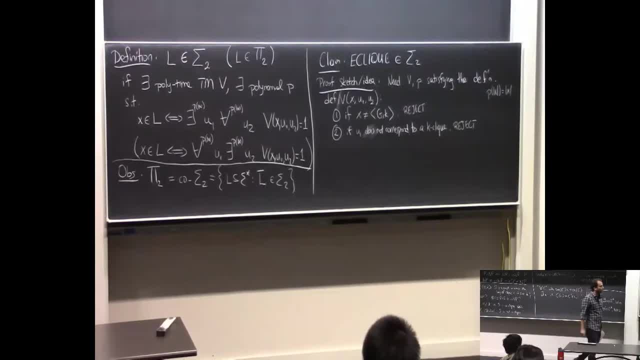 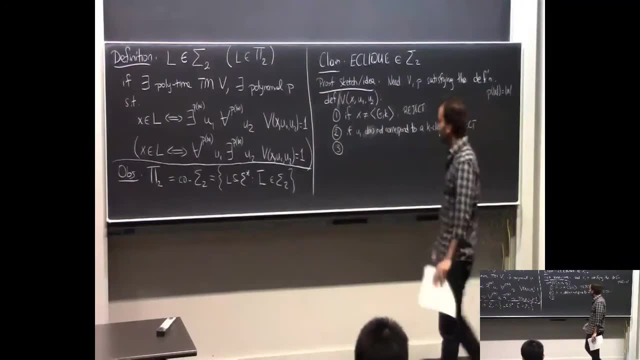 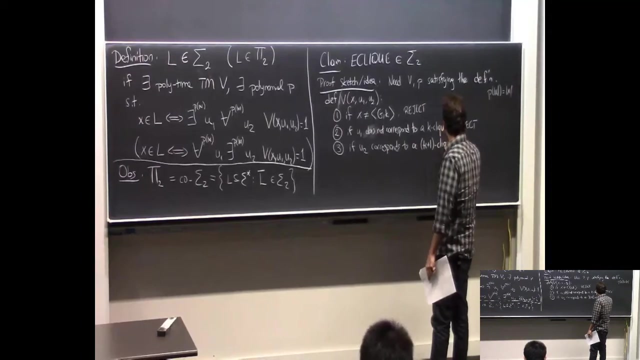 like this. This is trying, we're trying to mimic this idea here in our verifier number three: If U2 corresponds to corresponds to a K plus 1, click a click of size K plus 1, that's not a good sign. reject. 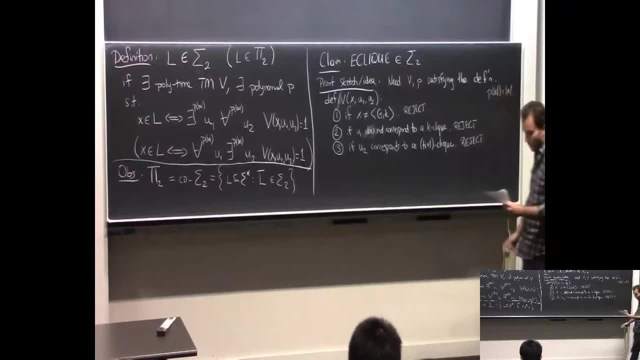 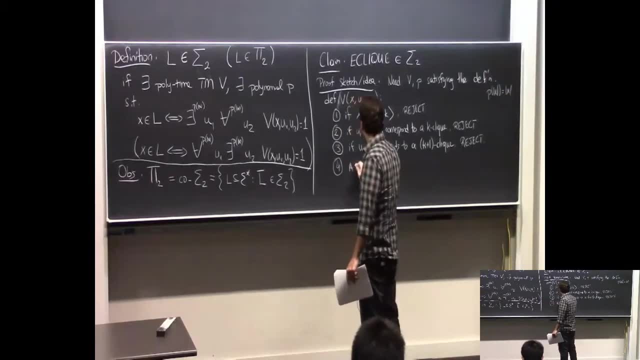 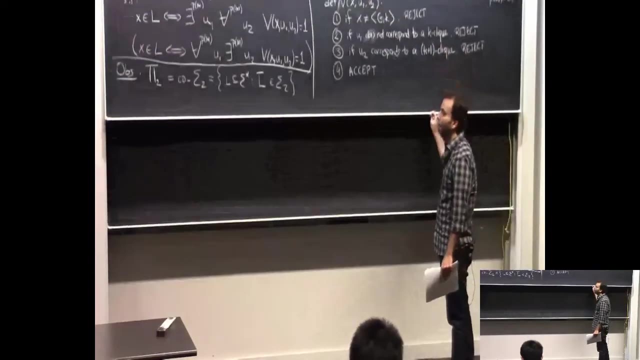 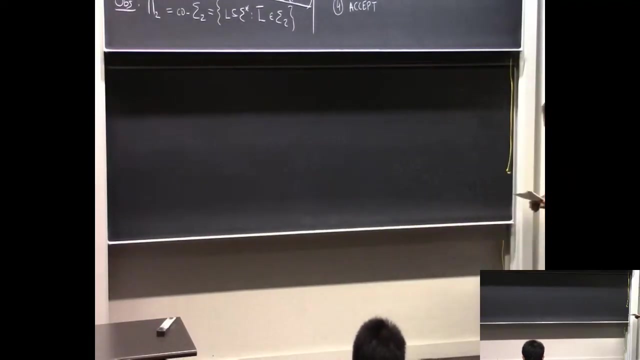 And otherwise you can accept. Okay, So now we can like check whether this V satisfies the K-click. Okay, So now we can like check whether this V satisfies the K-click. Now we can also check whether U2 satisfies our definition. 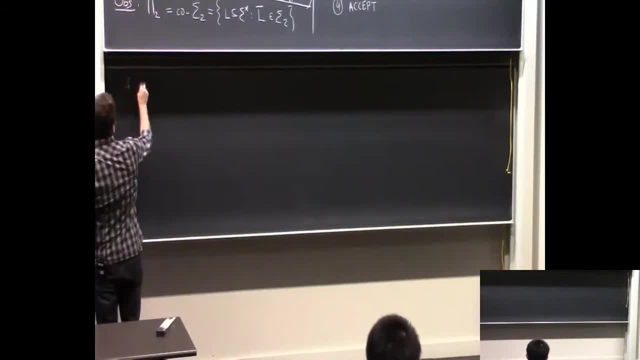 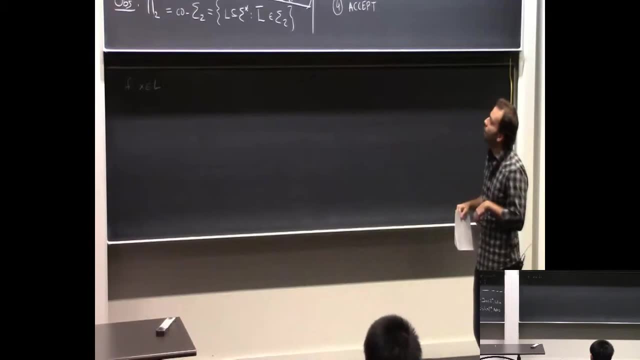 So if X is in L, when X is in L, so do we have that there exist U1, such that for all U2, V, X, U1, U2 accepts Well, what's going to be the U1?. 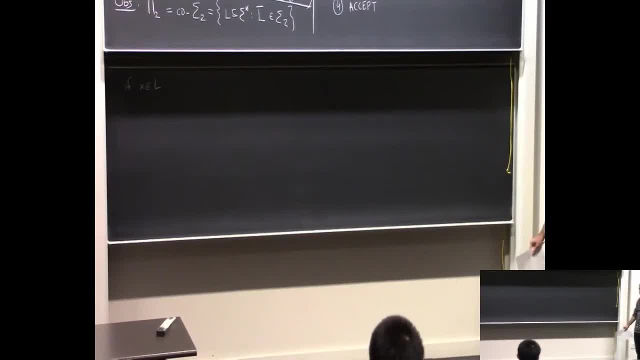 If X is in L, first of all there is a click of size K. The largest click of size, largest clique in the graph is of size K. So I can, I'm gonna- expect this U1 to be that correspond to that clique of size K, right? And so for the first step, 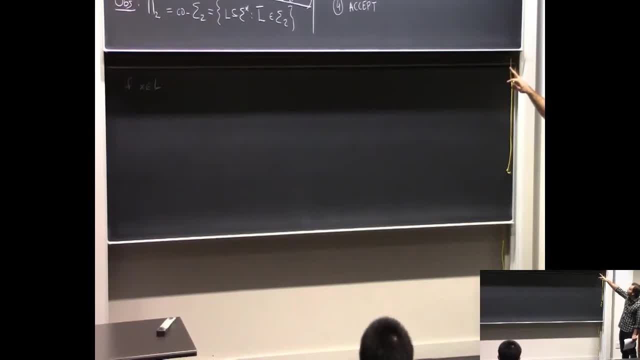 is good, like I'm not gonna reject there. Second step: U1, okay, so there will be a U1 where I won't reject in second step. It will make me happy with if you give me the K clique Three. if U2 corresponds to a K plus one clique, No matter what U2. 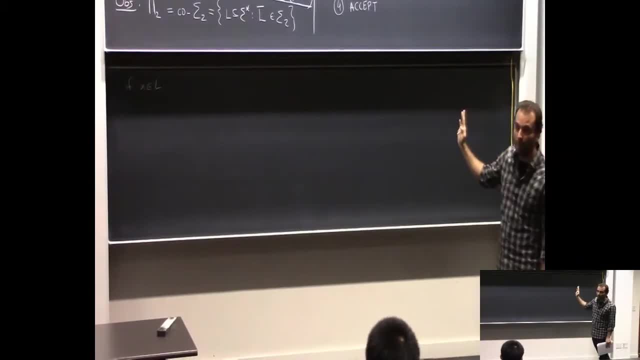 you give me. it cannot correspond to a K plus one clique in this graph, right? So I will never reject. there will never be a U2 that makes me reject. Okay, so that means that, for all U2, now, given that U1,, given that U1, for all U2, I. 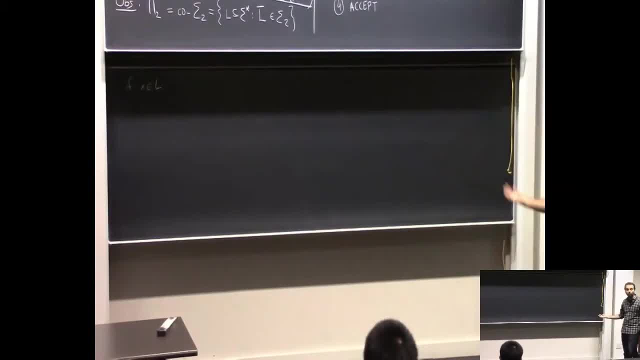 will accept, as I should. Okay, so it's, as I said, this kind of mind-bending. you have to play around with two quantifiers. You don't want to do that. when it gets to three quantifiers, We'll see. we'll see. 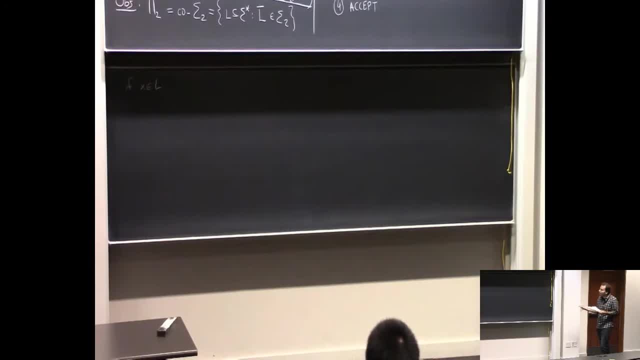 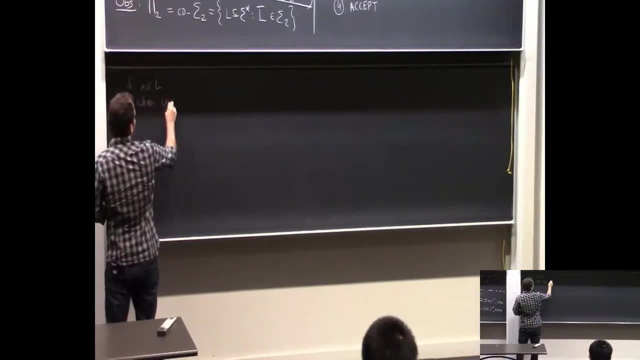 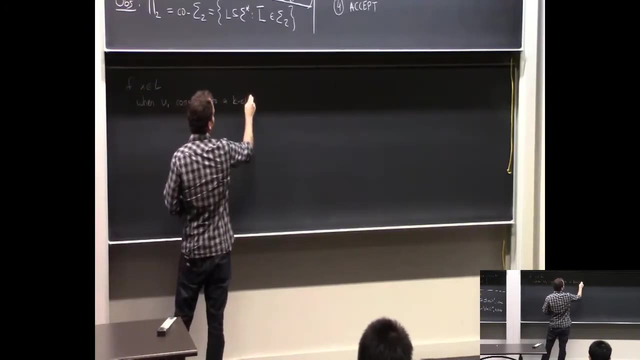 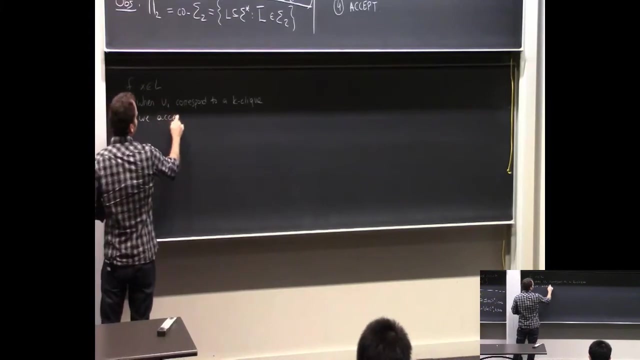 We'll see that too. but yeah, So that's like, if X is an L, I hopefully I can say like when, when U1 corresponds to a K clique, which which the graph does have, we accept, We accept no matter what. 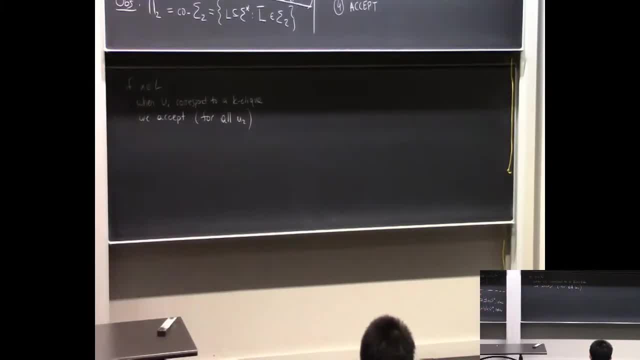 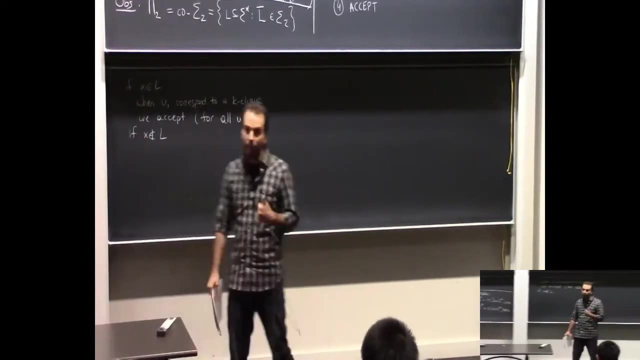 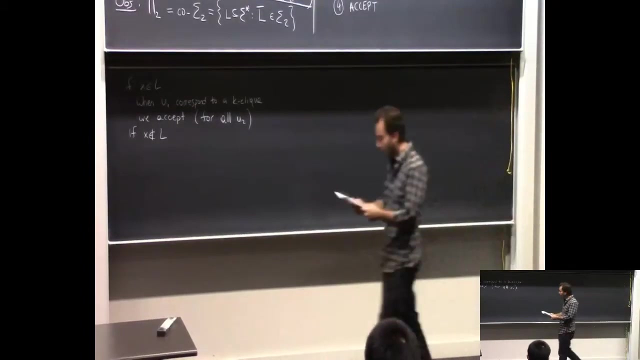 U2 is for all U2.. Now, how about if X is not in the language? Well, there are several ways that it cannot it's not in the language. One is like the trivial case where, like it doesn't even correspond to a valid encoding, Then we automatically reject. So let's say: 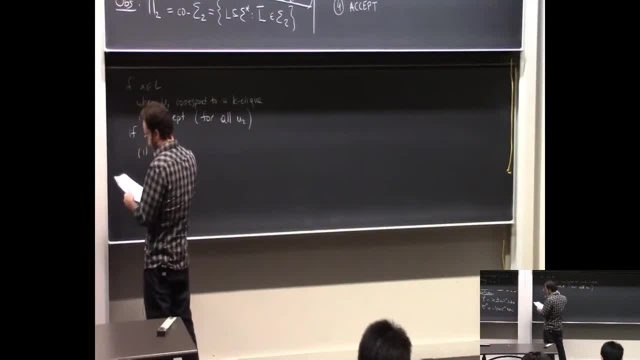 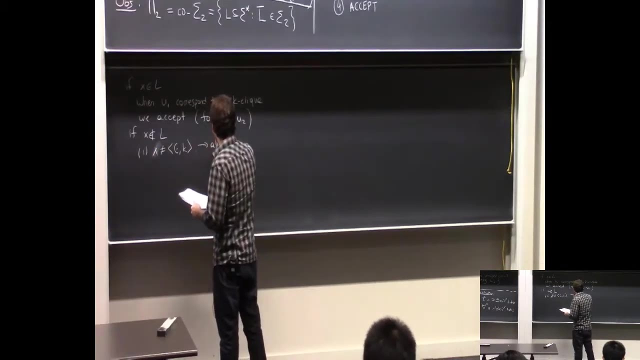 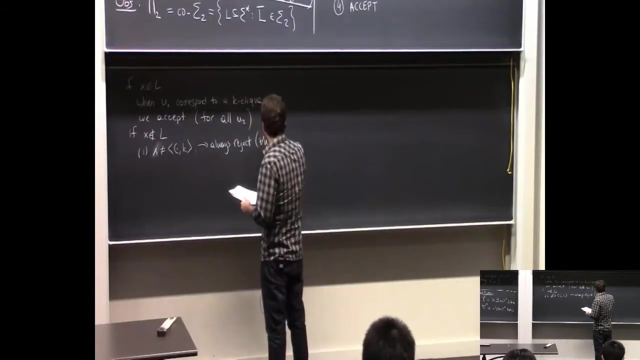 go case by one, case by case. So let me, I don't get it. I'm going to manipulateogaatch gave me an L, Let me duplicate and I'm going to satirize. So let me duplicate this and I'm going to litem latter point. okay, I'm going to. modify this to be U1, I'm going to try and lift this by 1.. I'm going to limit this by 1.. In this case, it could go wherever it could go wherever, So we're not going to predict this. So let's say, if the um, let's say X, is not equal to GK, and in this case always reject. this is for all U1, U2.. Okay, so if X is not in the language, if I tell him: ah, you can be careful. 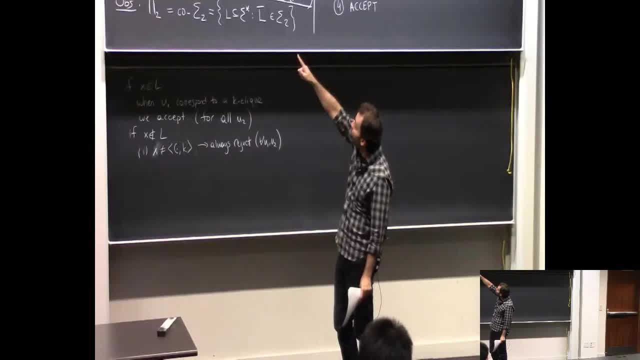 This is a string. I'm going to drop these arrow hairs, these arrow hairs in the middle. What I want is that for all u1, there exists some u2 that makes the verifier reject. In this case, I'm saying for all u1,. 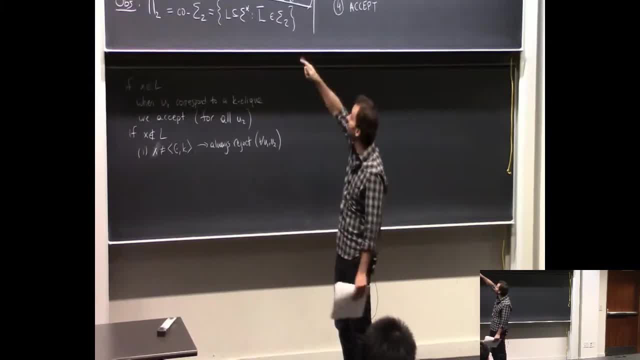 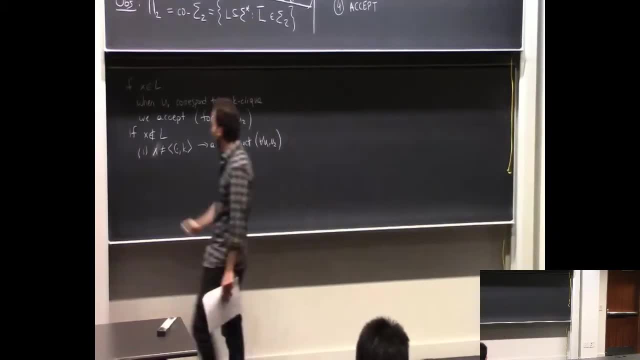 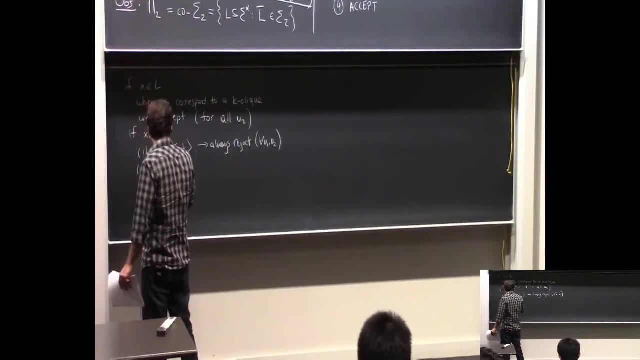 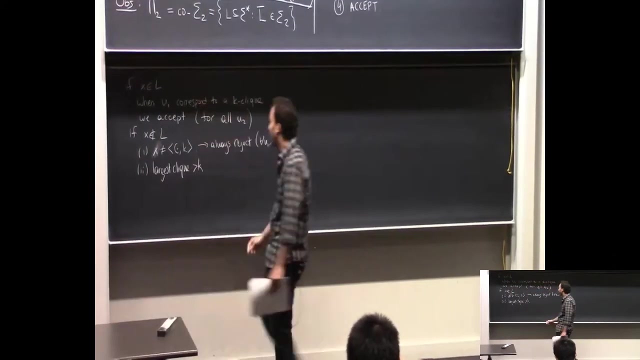 not only there exists a u2, but for all u2,. that's okay. It's more than I need. The verifier rejects. What about another case? So it could be the case that largest clique is at least k, or more than k, I should say. 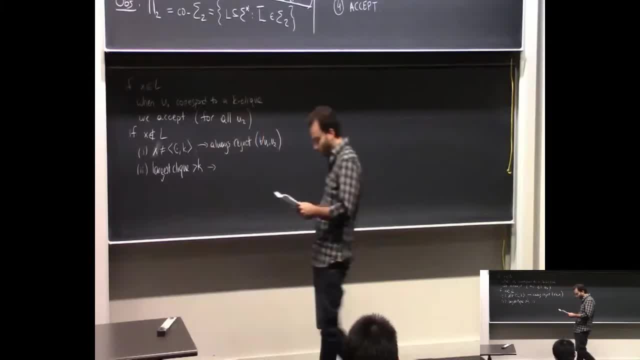 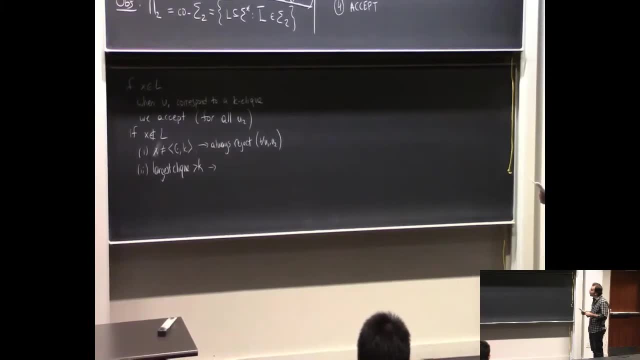 Then what Well if the largest clique is more than u1,? then what Well if the largest clique is more than u1,? then what Well if the largest clique is more than k? first of all, if u1 does not correspond to a k clique, we reject anyway. 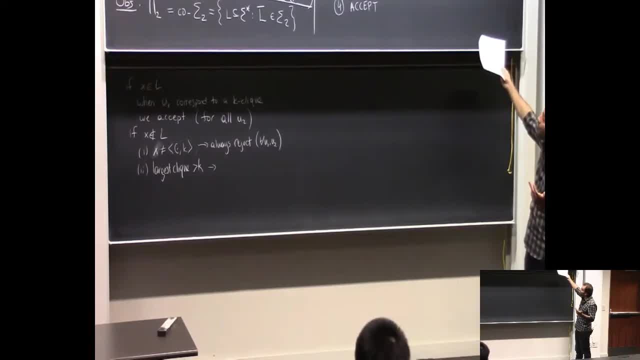 If u1 does correspond to a k clique, then there exists some u2 that makes there should exist some u2 that makes me reject, And that u2, of course, is going to be the string that corresponds to a k plus 1 clique. 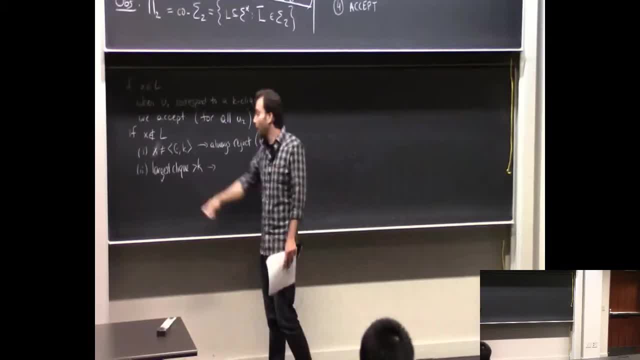 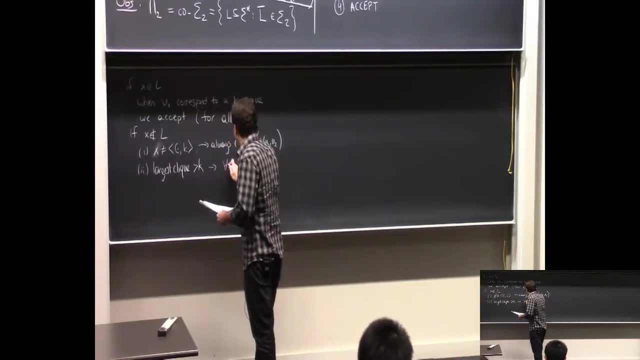 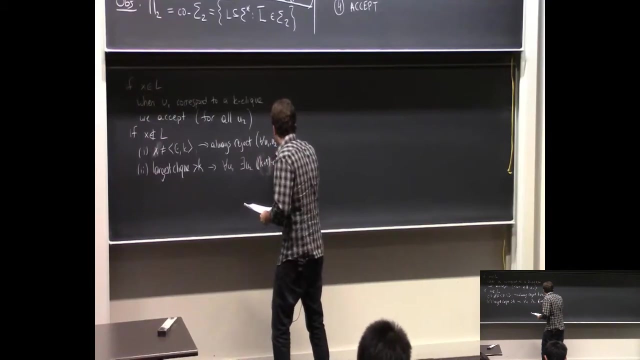 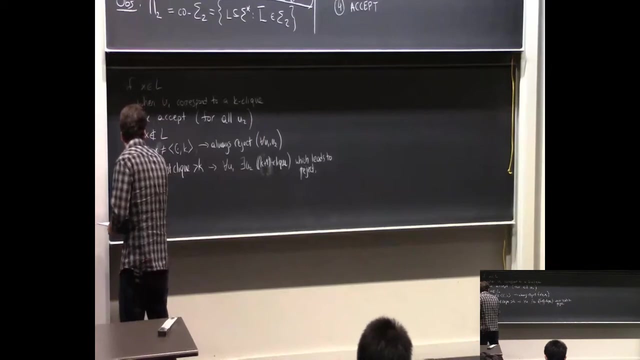 that does exist. by this assumption, right, I'll say that for all u1, there exists u2.. So this is a clique, This u2 is a clique. Let me say k plus 1 clique, Which leads to reject. Okay, And then the third case is: largest clique is less than k. 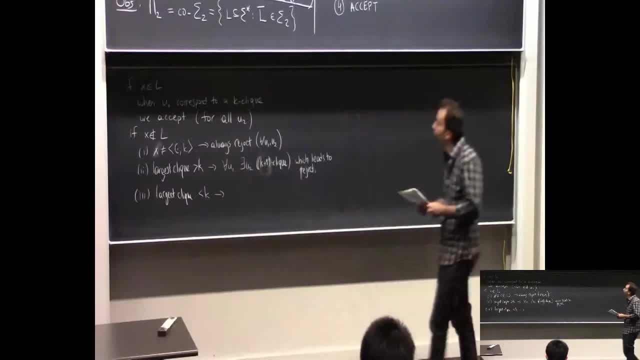 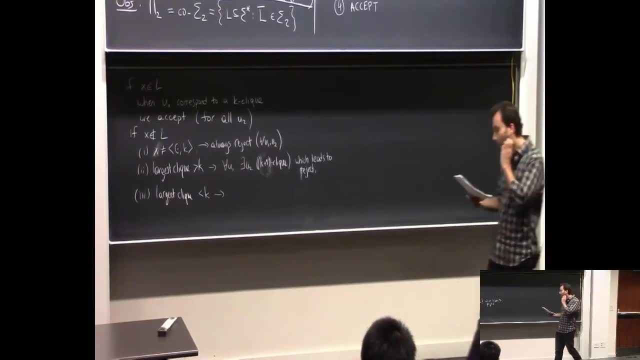 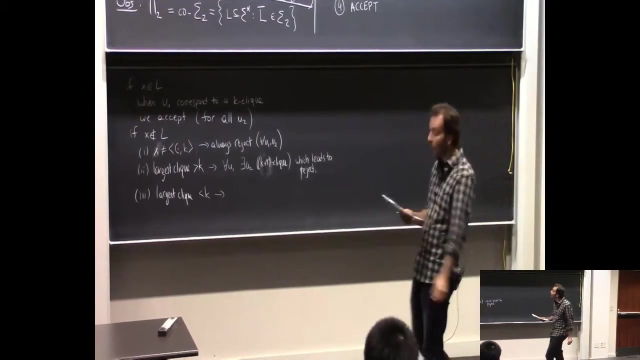 So then, what's the situation? Where do I reject Step two, And step two I'm going to reject, right? So u1 will never correspond to a k clique. It cannot correspond to a k clique. So for all u1, and then it doesn't matter what u2 is. 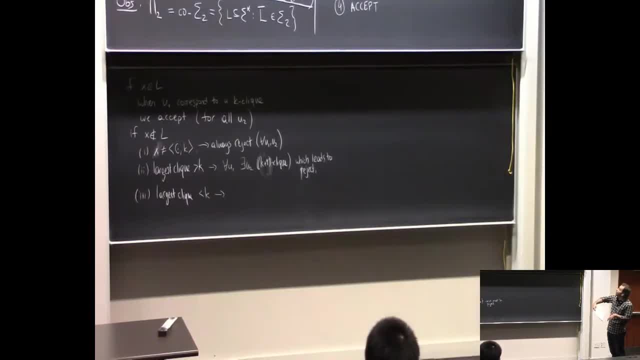 I'm not even checking what u2 is, So once I detect that u1 does not correspond to a k clique, I'm going to reject. If u1 does not correspond to a k clique, then for every u2,, whatever it is, I'm going to reject. 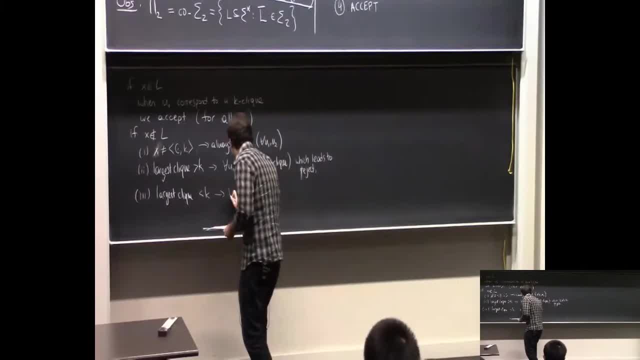 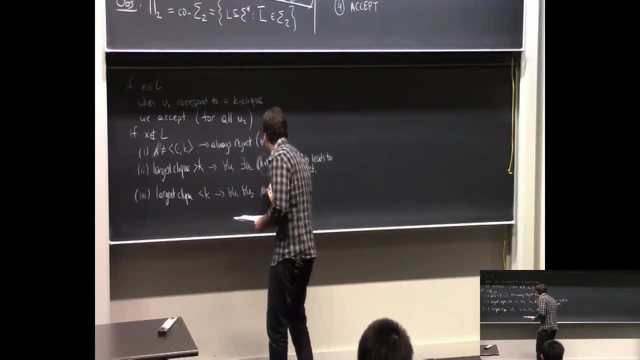 So here, for all u1 and for all u2, you reject, Verifier Rejects. So, as I said, you know by the, what the definition requires is like you want for all u1 that there is a k clique. 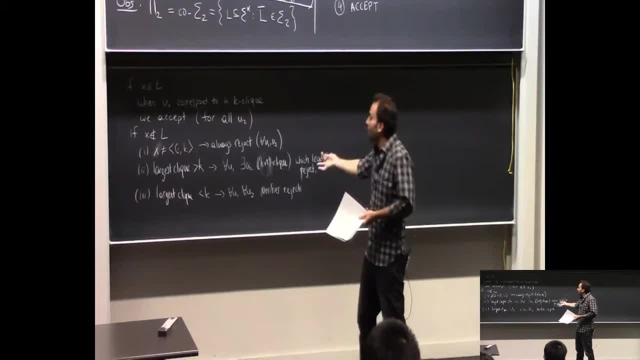 That there exists a u2, that it makes it reject. But sometimes it's like for all u1, for all u2, you reject, And that's fine. If you have for all u2, that implies there exists a u2.. 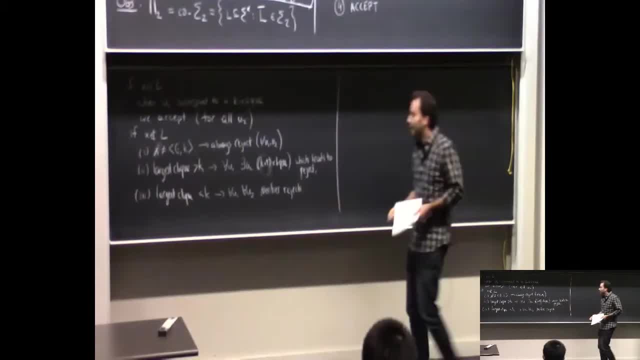 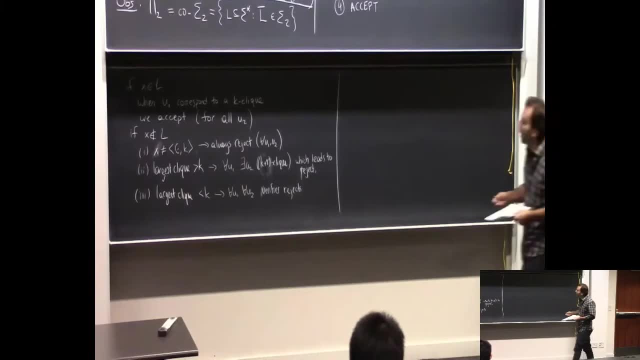 Okay, So that was just like to give you some. I mean, I did that in some level of detail to give you some intuition about how to think about these things. I'll also say I'm not going to prove this, but this is an exercise for you. 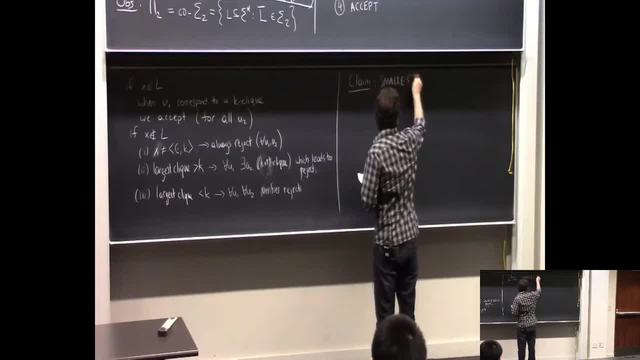 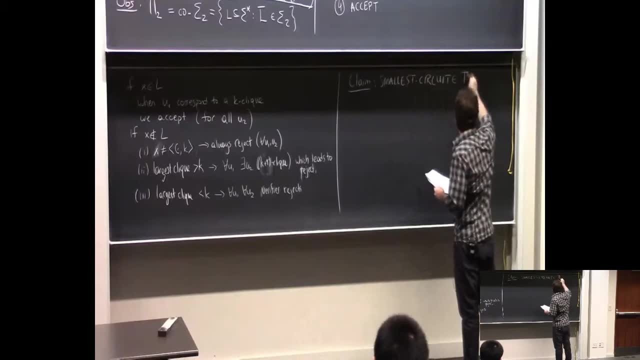 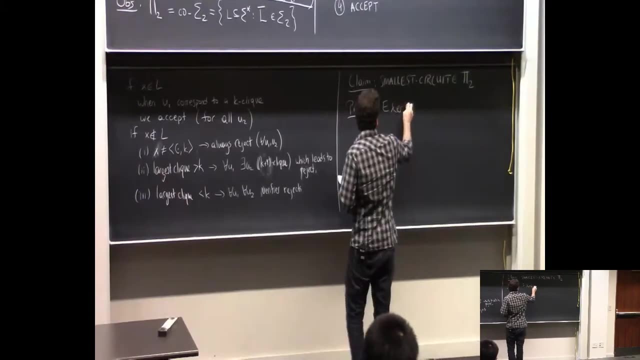 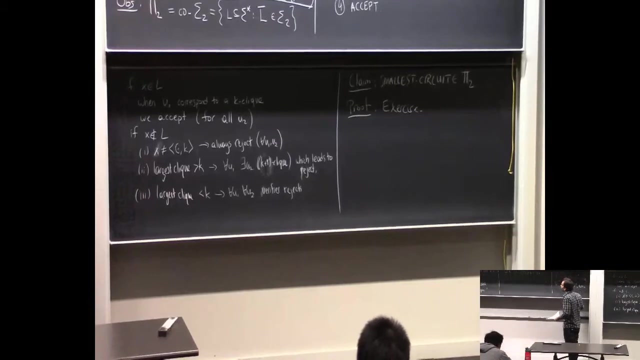 Smallest circuit Is in pi 2, okay, And the proof is exercise. Or maybe it's show up in the homework, I don't know. Okay, So let me come back here. If you have any questions, Let me know. 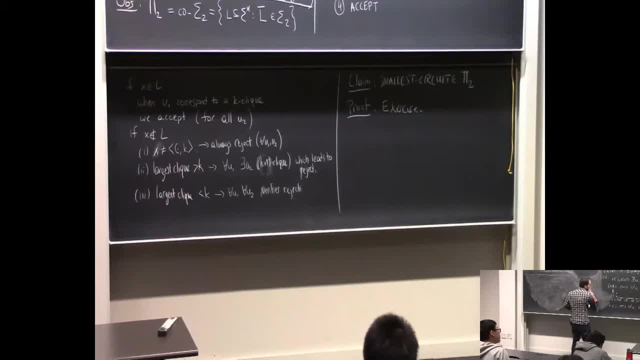 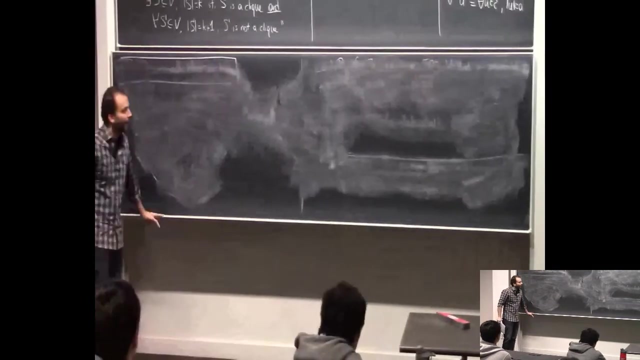 Okay. so now, obviously we're not going to just stop at two quantifiers, right, We're just going to keep going, All right. so let me give you some notation. 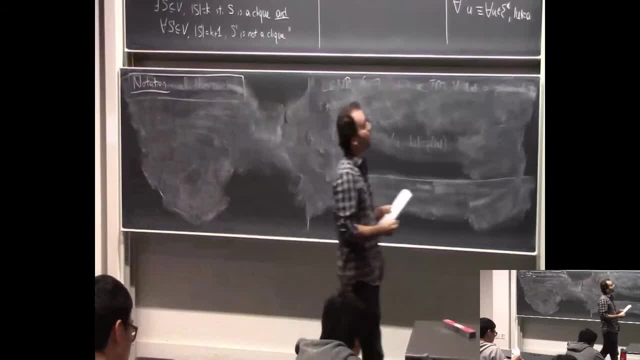 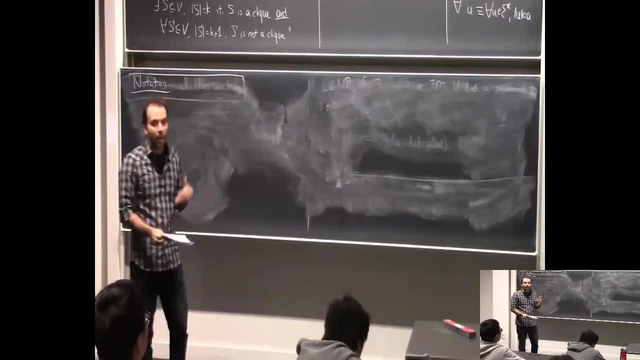 So, as you can imagine, I can take this definition and I can say, oh, L is in sigma 3.. If there exists a polynomial time-turning machine, V, there exists a polynomial P. So I said X is in L if, and only if, there exists U1, for all U2, there exists U3,, such that VX, U1, U2, U3 is 1.. 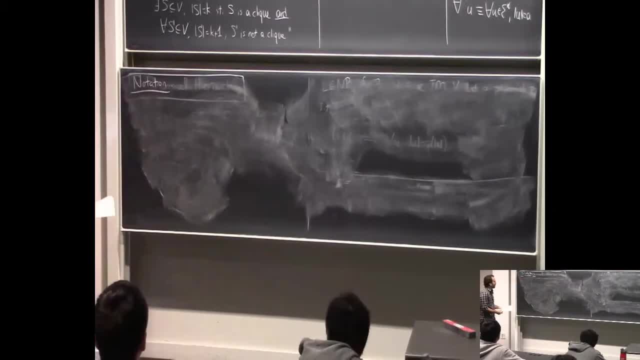 So I can just add another quantifier to this. So I'm not going to write that definition down, but instead let me just give you the notation here. So first of all, sigma 0, pi 0. So this index I refers to. 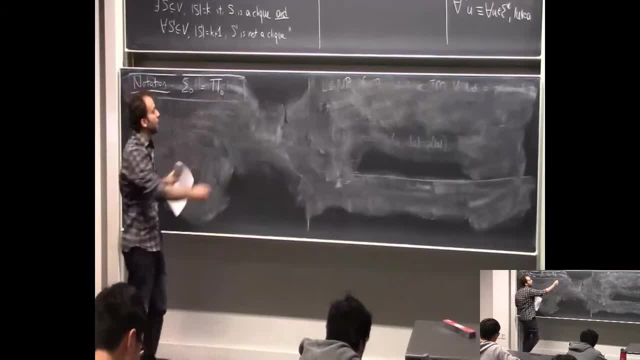 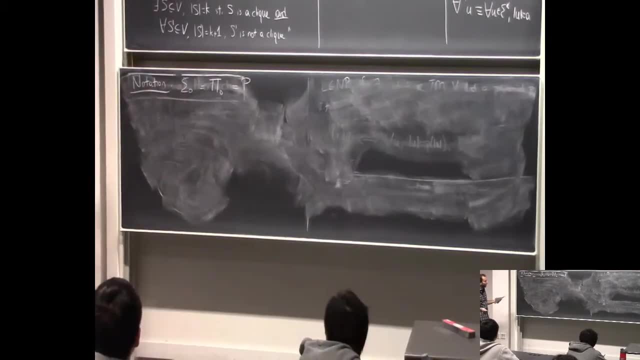 The number of quantifiers. okay, So this is just going to be good old polynomial time: P. Okay. now, if you don't have any quantifiers, it's polynomial, it's P. Now, sigma 1 actually corresponds to MP. 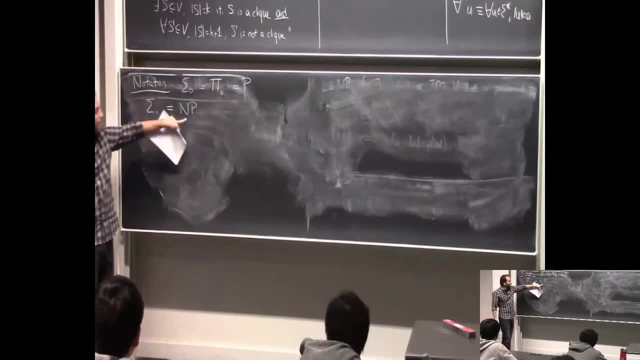 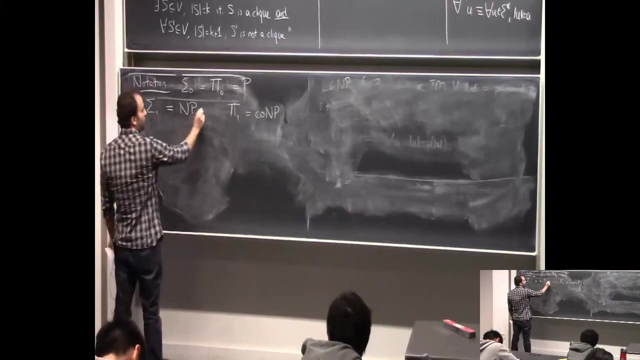 Okay, one quantifier. there exists quantifier. This is MP, And pi 1 corresponds to co-MP. Okay, one for all quantifier, And actually I'm even going to write this as So this is like a notation that I'm introducing now. 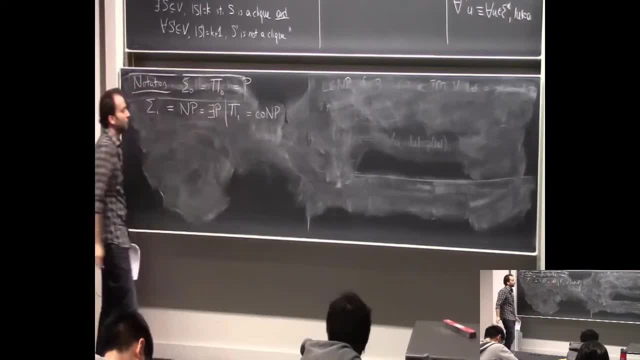 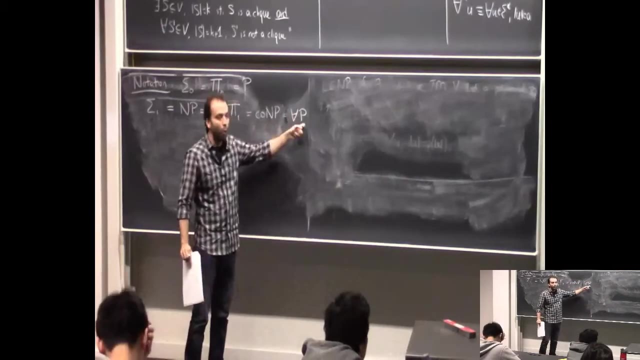 I'm going to write this as there exists P, Okay, and I'm going to write this co-MP as for all P. Okay, so I have these quantifiers and at the end, I have a polynomial time machine. Okay, so I have the quantifiers and then your polynomial time verifier. 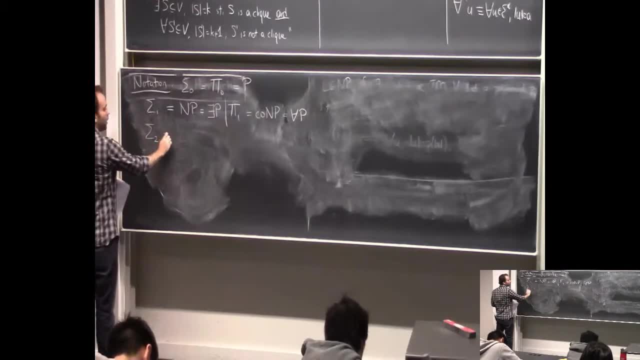 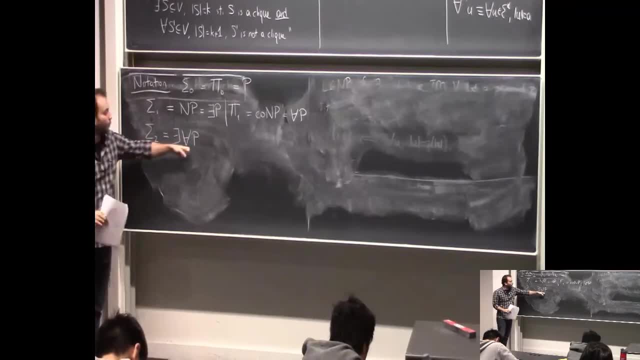 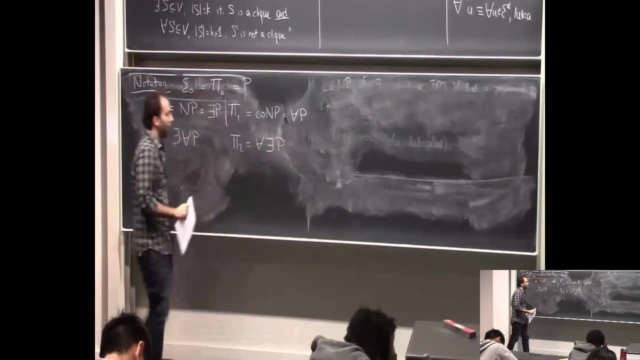 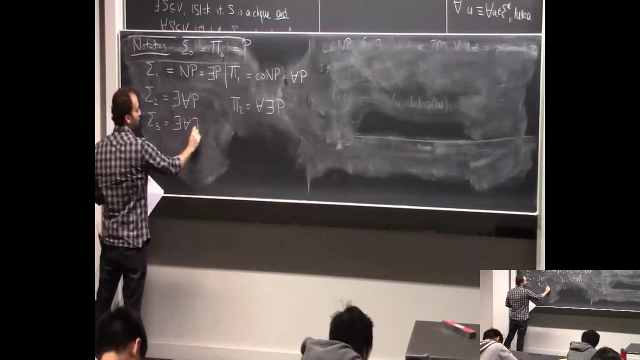 Okay, so this is a good way to remember it. There exists for all P, and then pi 2 is for all. there exists P, And then keep going. There exists for all, there exists P, pi 3 for all. 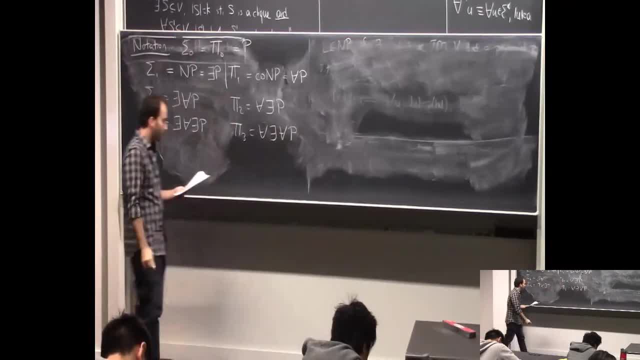 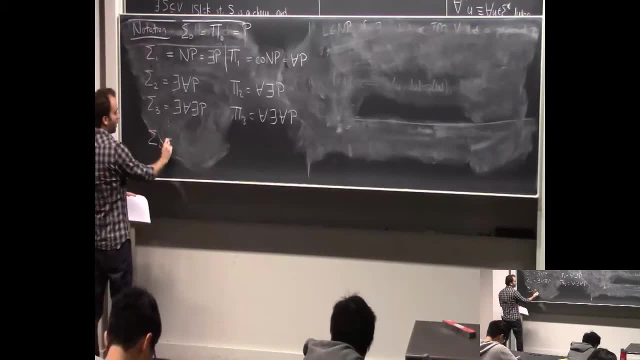 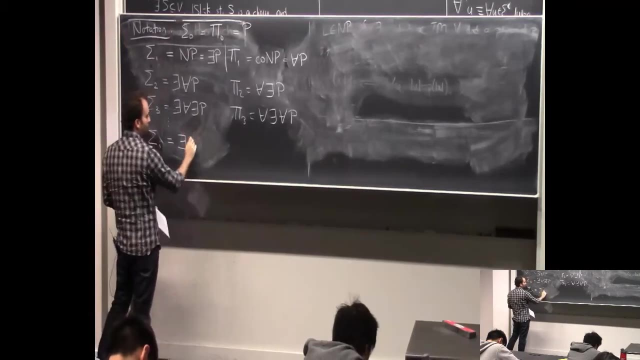 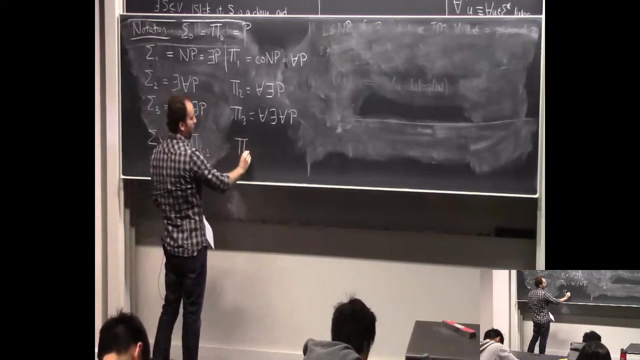 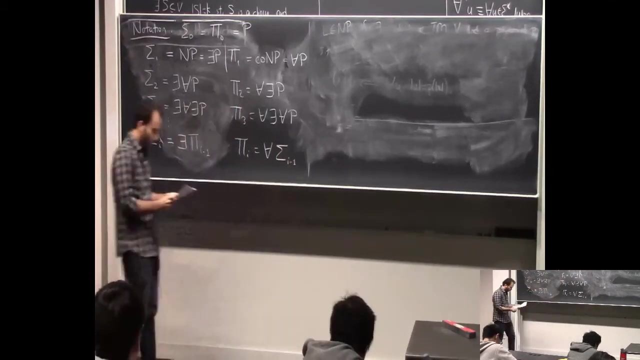 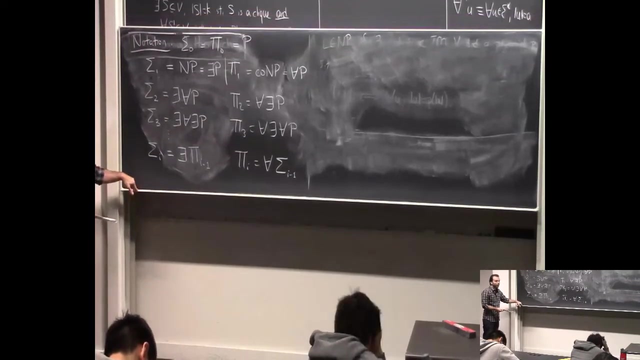 there exists for all p and you go like this: in general you can say: like Sigma i is equal to, there exists Sigma, not Sigma pi. pi i minus 1 and in general pi i is for all and then Sigma i minus 1. okay, so for each fixed I we can define these complexity classes. just again an. 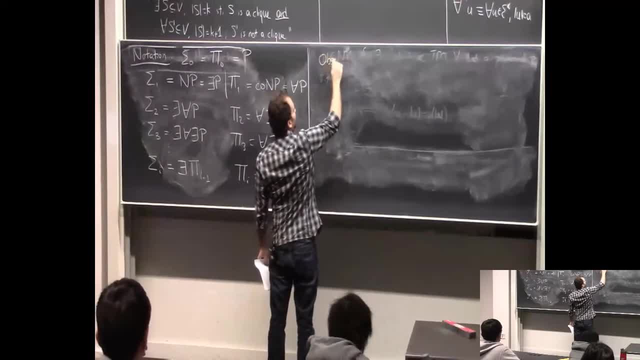 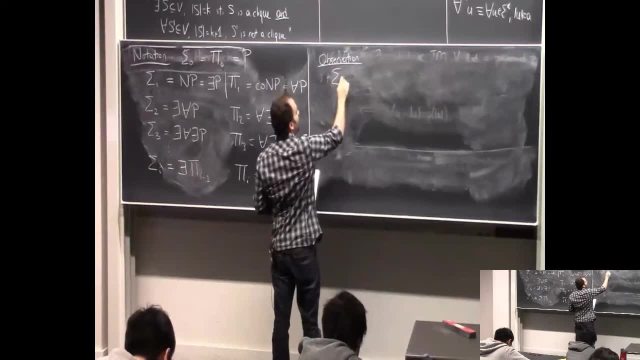 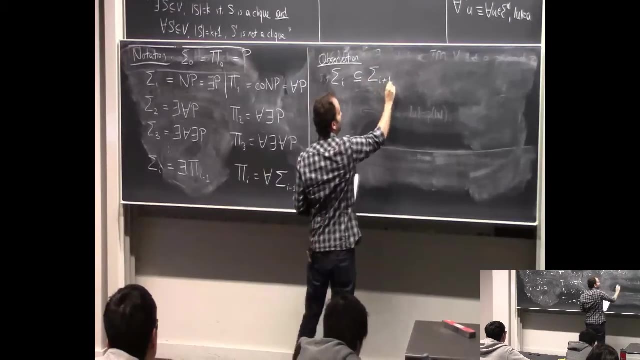 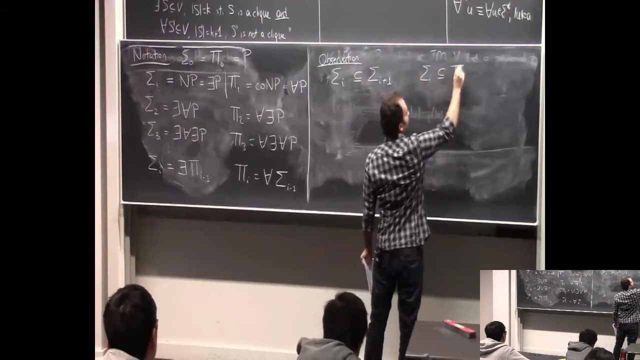 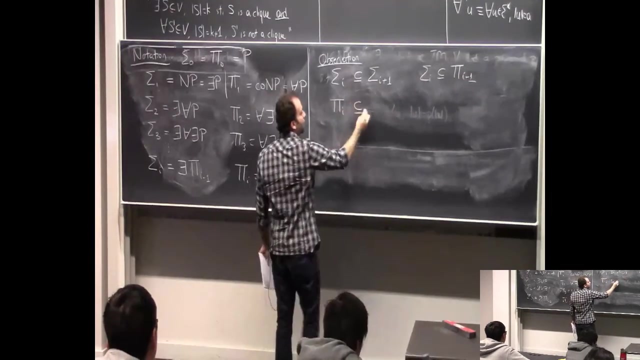 observation. so this is the observation- is that Sigma is always contained in- well, first of all sigma i plus 1, but it's also always contained in pi i plus 1.. And similarly we have pi i is contained in pi i plus 1. 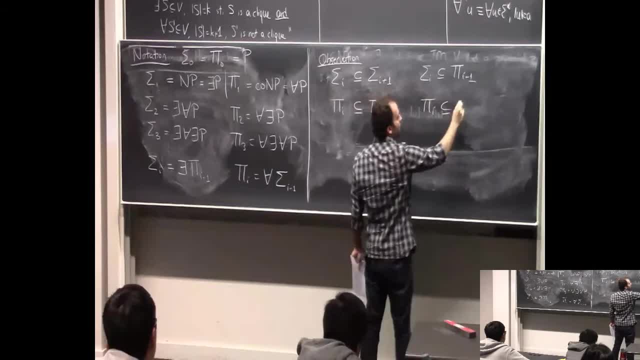 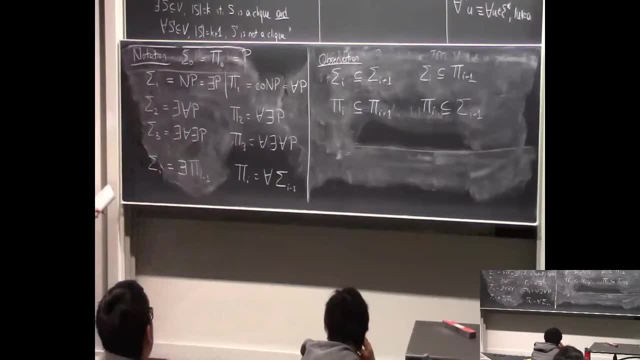 and pi i is contained in sigma i plus 1.. So why is this the case? So let's say, like you take sigma 3. Sigma, let me. let me put. no, let me take sigma 2.. So sigma 2: 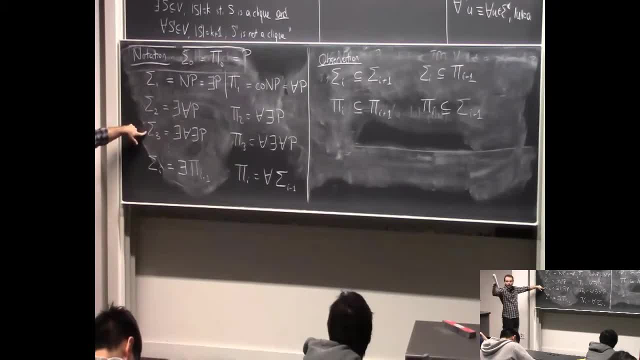 is contained in sigma 3.. Yeah, So is there a reason why, like when we go from sigma 2 to sigma 3, why do we have to put just one? like there exists, like, why is there a reason why we can't like change? 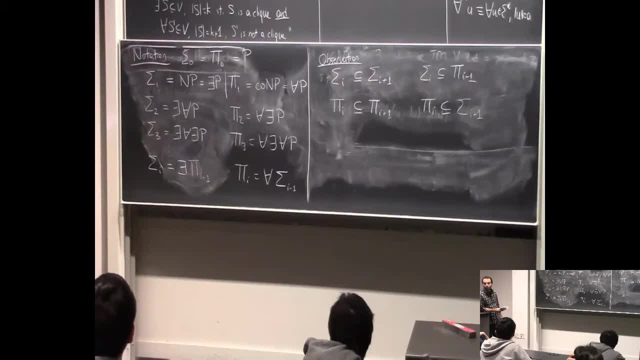 the ordering, or does it have to be like? Oh yeah, the changing ordering can. yeah, Yeah, it has to be alternating. So yeah, here's one thing I can tell you is that if you have two there exists in a row, you can collapse them into one there exists, Okay. so if you 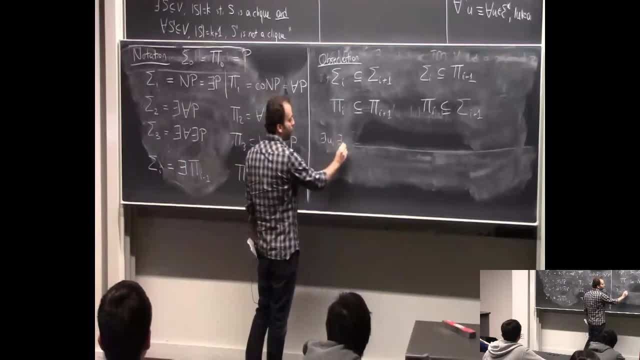 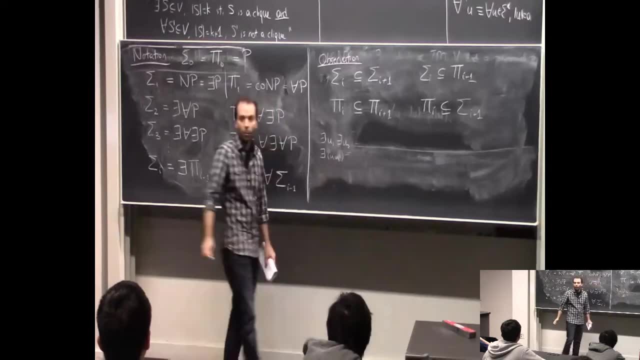 had like there exists u1 and there exists u2,. okay, so just take this as like there exists. well, just combine them. Combine them together: u1, u2, and that will be your new u. You will call that u. 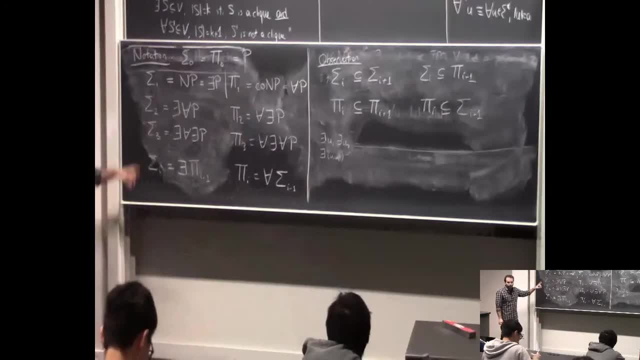 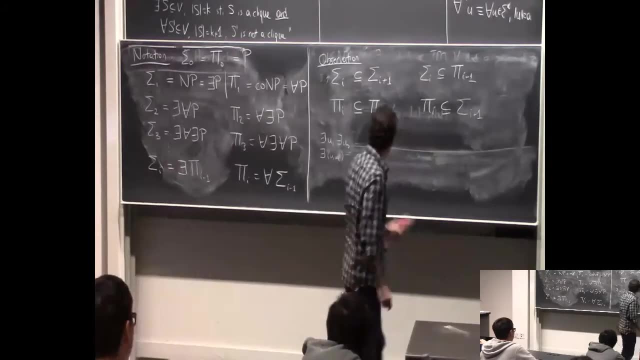 Okay, so you can just turn anything into this. Yeah, so I tell it will always be alternating, You can make it. yeah, Good question. Okay, So now yeah, and then here, like, if you say like sigma 2 is contained in sigma 3, why? 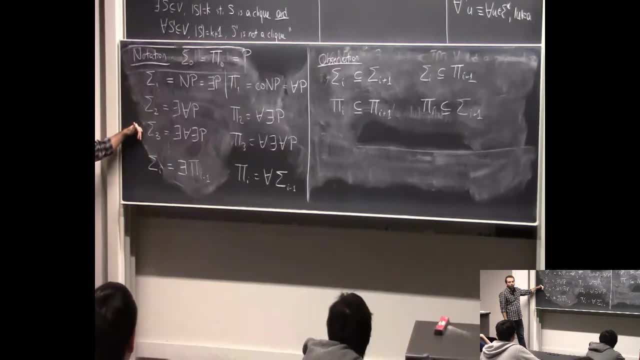 is that the case? Like, adding more quantifiers gives you more power, It cannot restrict you. It can give you more things to do. You can always ignore one of the quantifiers. You can say, oh, that's a dummy quantifier. It's there, but it's dummy, I'm not going to even look at it, kind of. 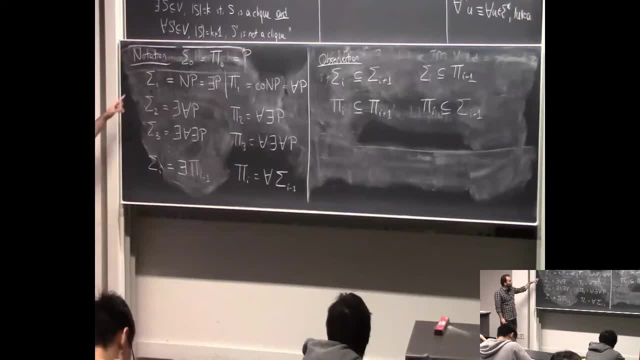 thing. Okay, so that's kind of the intuition, So that allows you to say, like well, you know, here I have three quantifiers, but here you know, if I just go from here to here and forget about this one, it's like pi 2.. If I forget about that one, it's like sigma. 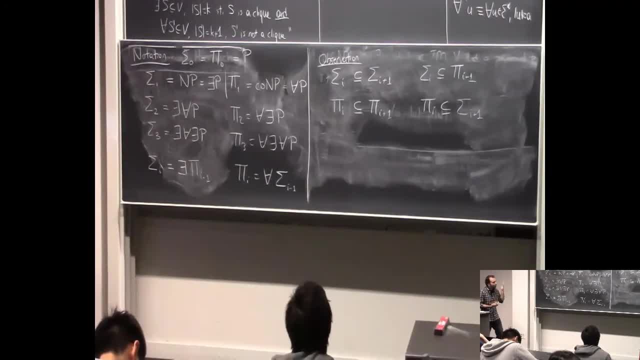 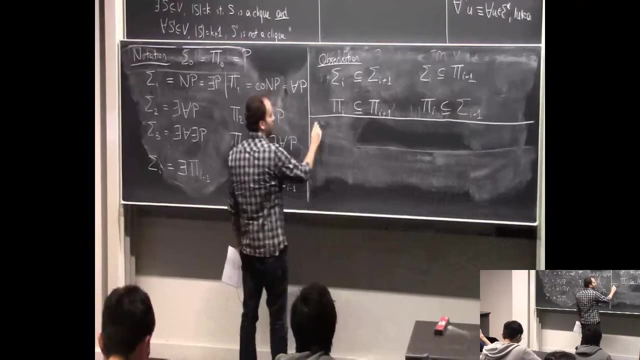 2, and so on. Okay, Um, so you have these inclusions. So having more quantifiers only gives you more power. And now the um, basically the title of the lecture- is the polynomial hierarchy, right, Okay? 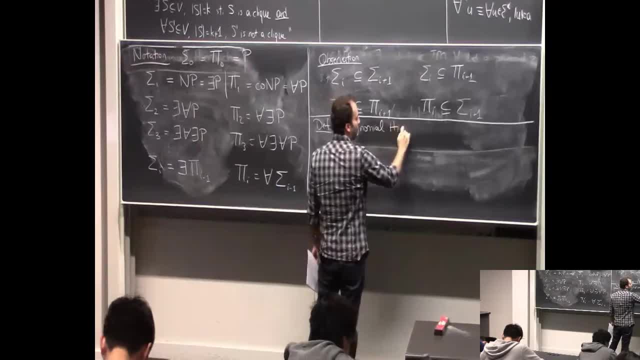 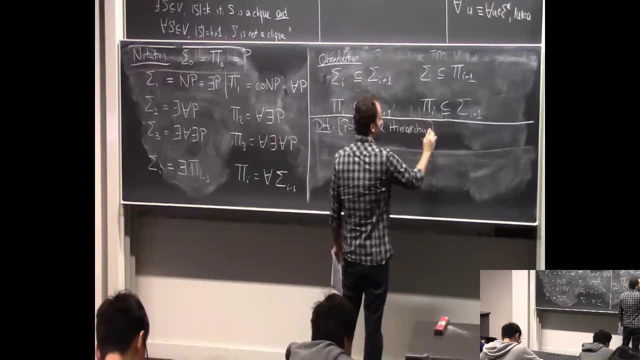 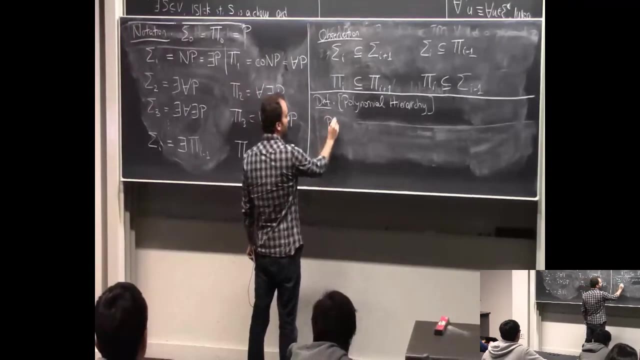 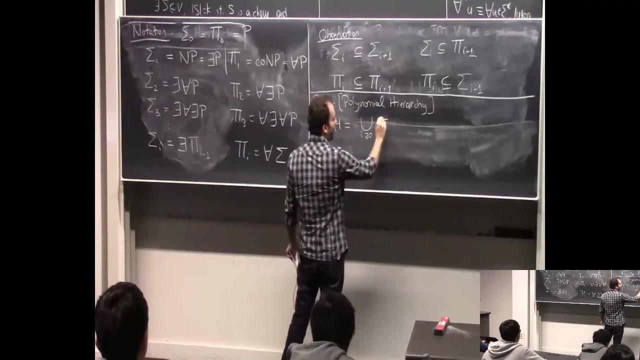 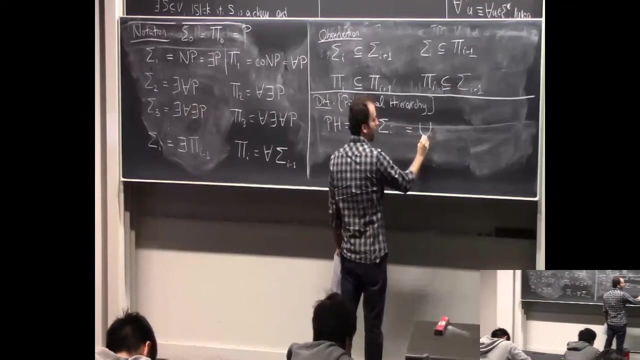 this is okay. so this is going to be the complexity class that we call pH polynomial hierarchy, which is the union over all I of. you can take it as Sigma I, but that's going to be equal to the union over all I, Phi, I and the reason. 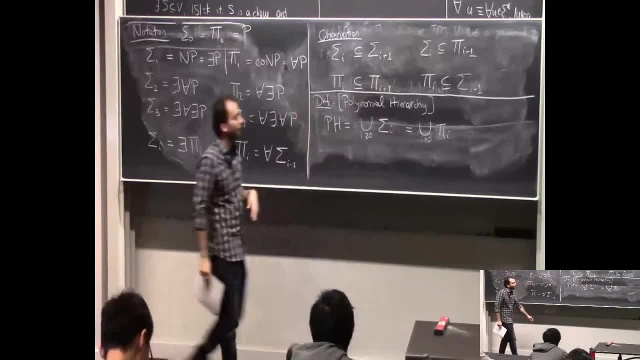 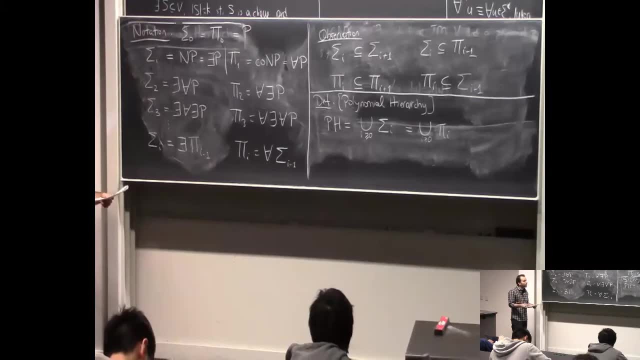 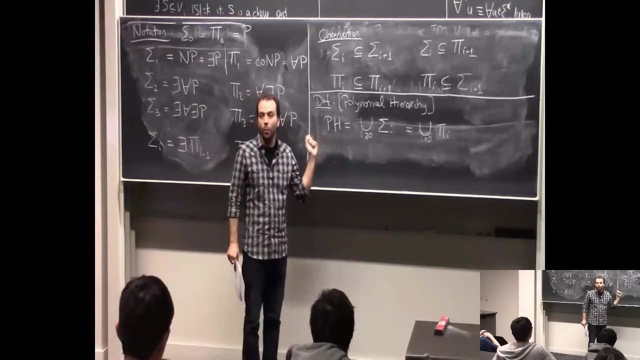 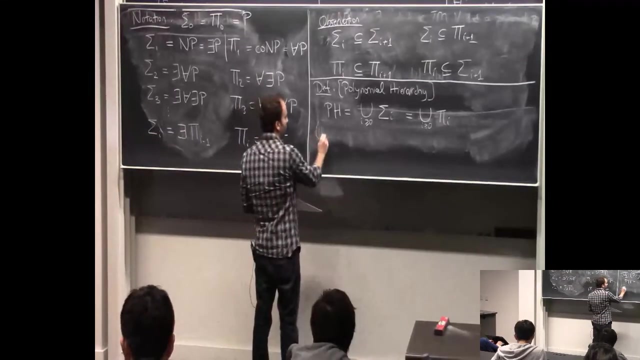 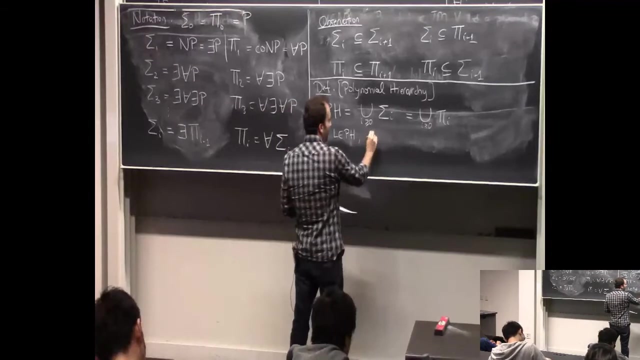 for this equality is because of this observation. so basically, intuitively, a language is in pH. okay, if you can describe it with some constant number of quantifiers, so let me write that down. so if L isn't pH, then then L is in, let's say, Sigma I. 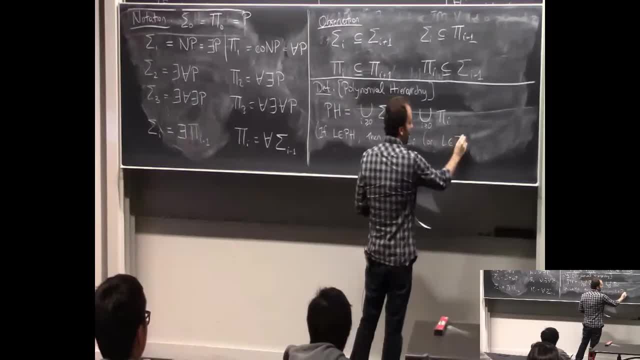 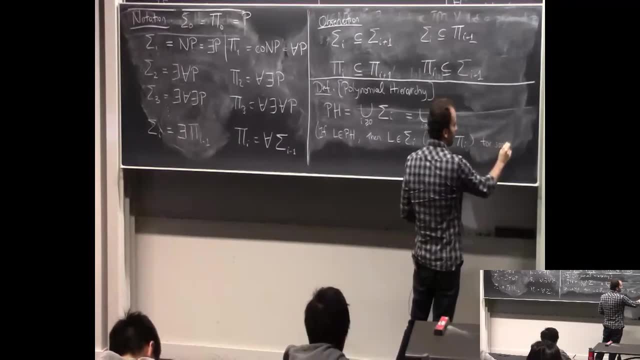 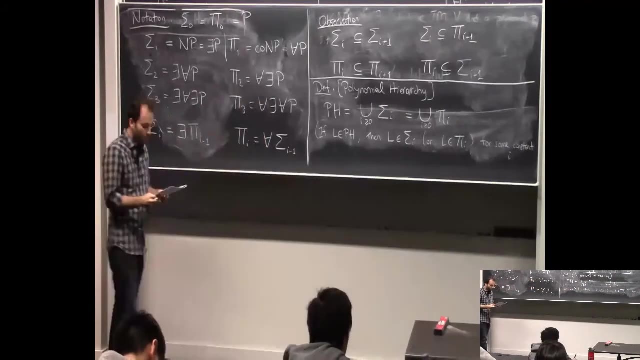 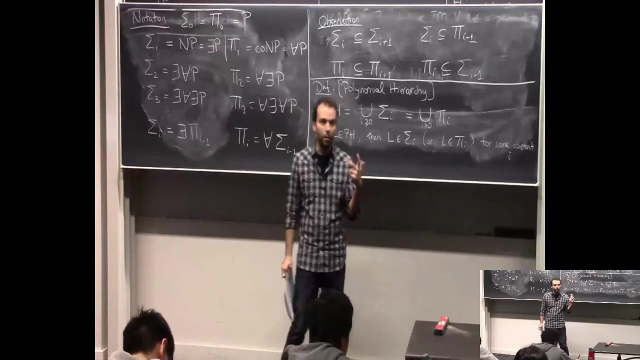 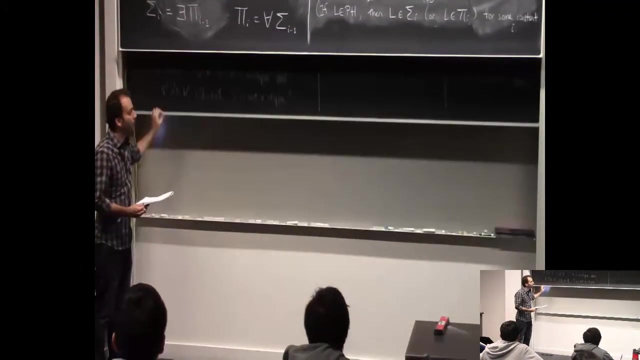 or L is in Pi, I that's can also write this way for some, for some constant, I okay, but the number of quantifiers, maybe I should highlight, cannot depend on the input length. okay, it's always some fixed constant, you can put it in, okay. and then now, with this definition and this observation, we have a nice 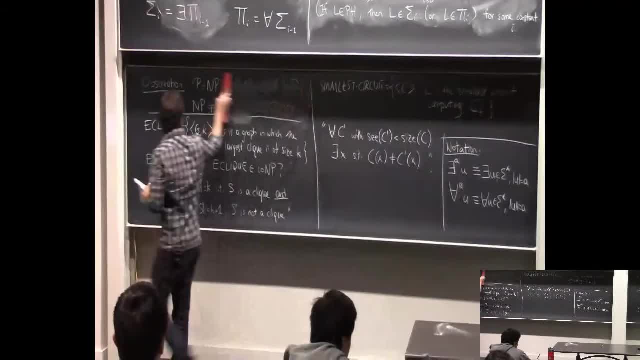 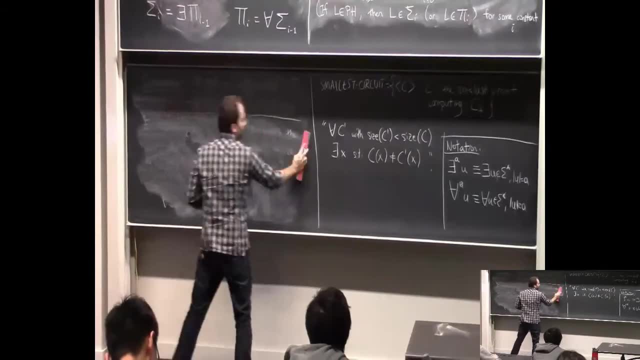 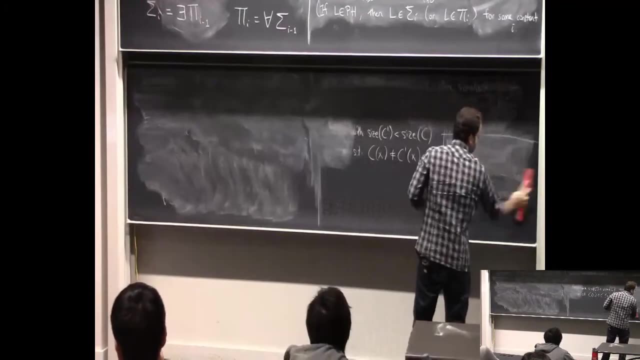 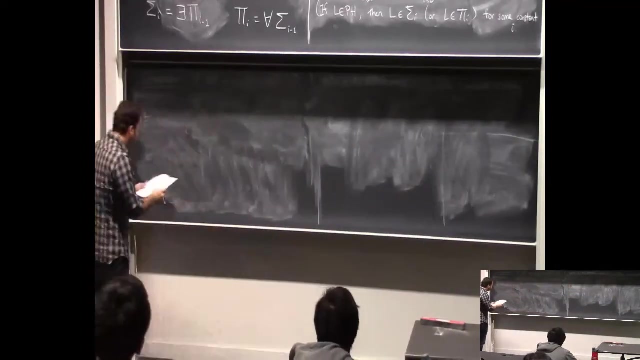 picture coming up, so just a moment. so the picture is this. so we have, we have P P L. we have to find that P L P E- OK, okay, very well, in Np is contained in CoNp. Np is sigma 1.. CoNp is pi 1.. Sigma 1 is contained in. 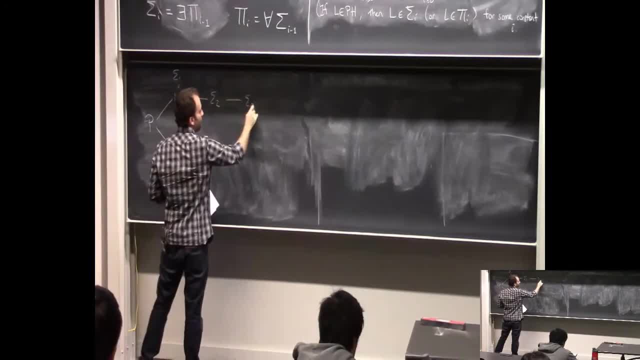 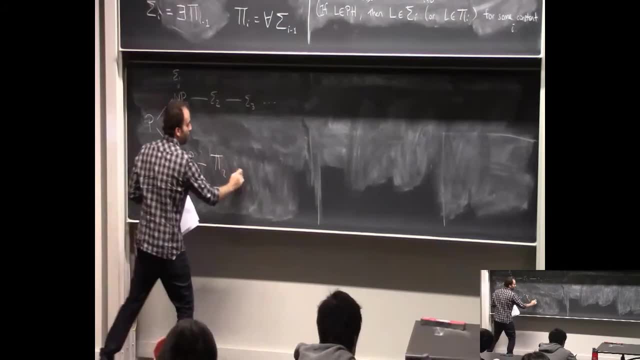 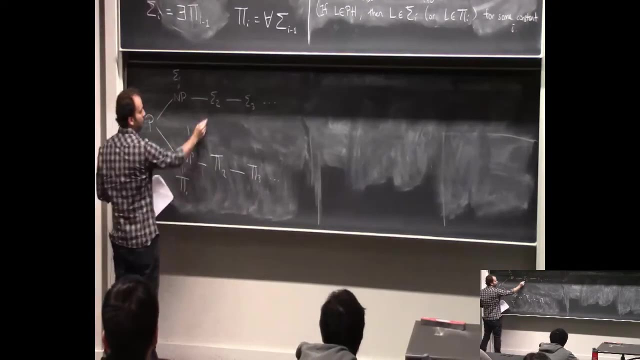 sigma 2, contained in sigma 3, and so on. Pi 1 is contained in pi 2, contained in pi 3, and so on. Furthermore, pi 1 is contained in sigma 2, and sigma 1 is. 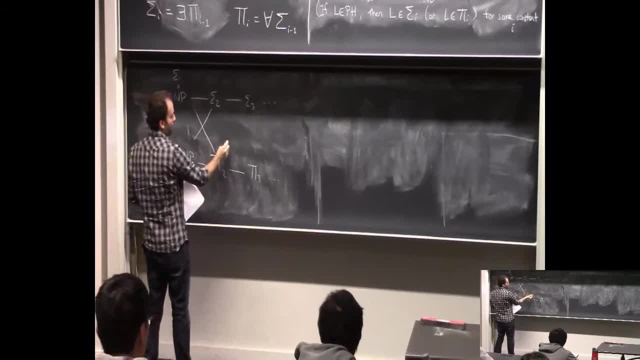 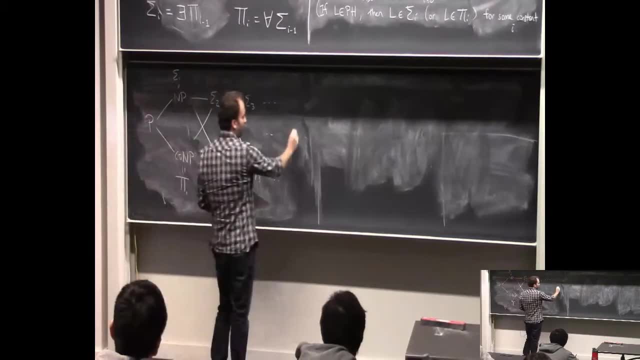 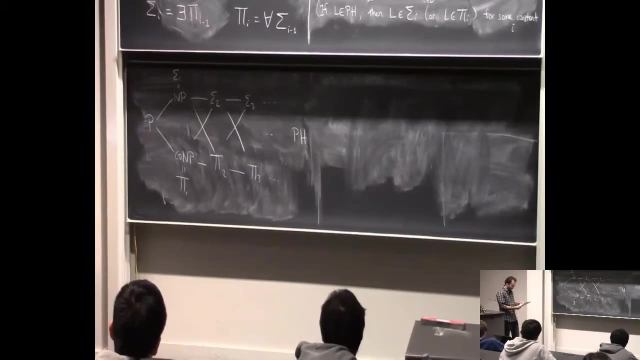 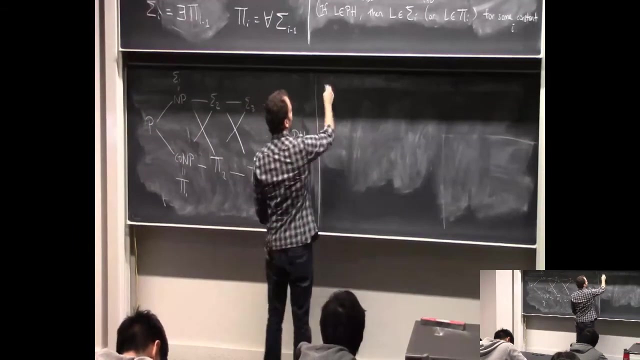 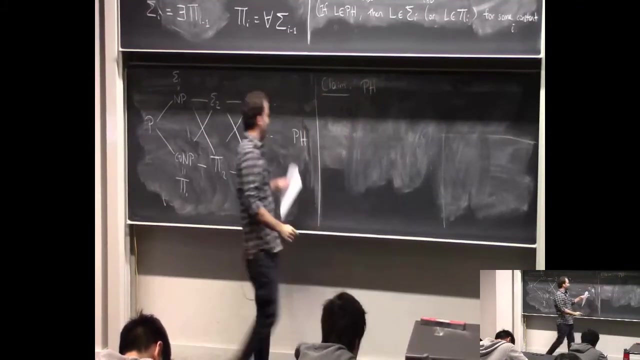 contained in pi 2, and similarly here and so on, And at the end we have pH polynomial hierarchy, the union of all of these guys, And here is a not a difficult claim, so let me put it as a claim. You might ask now: okay, 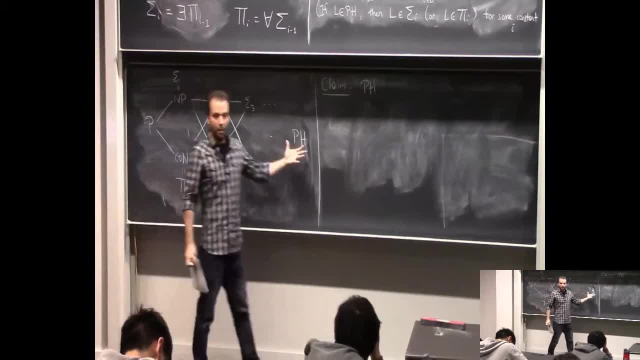 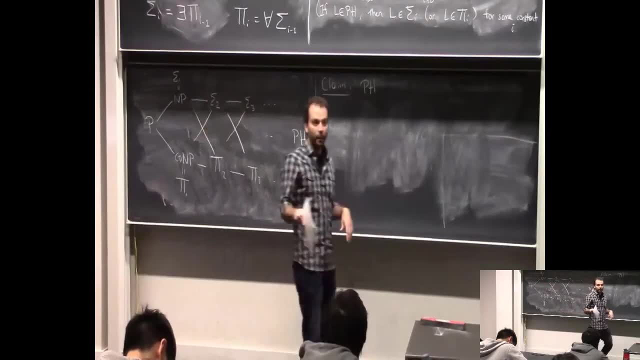 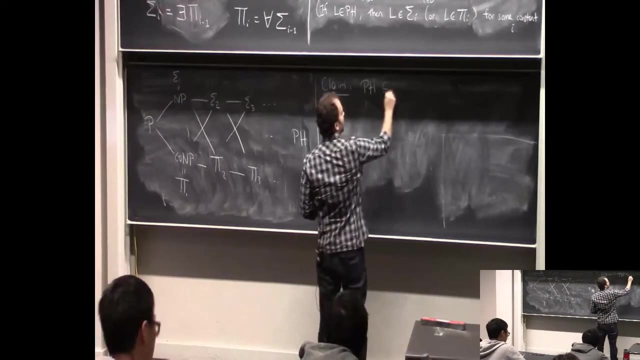 what's an upper bound on pH? Is there an upper bound on pH? What's a natural upper bound on pH? What do you think it is? Anyone have a guess? P-space, P-space, Absolutely. So why is it contained in p-space? Yeah, 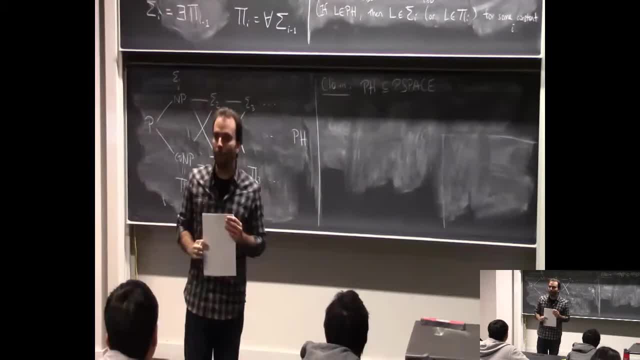 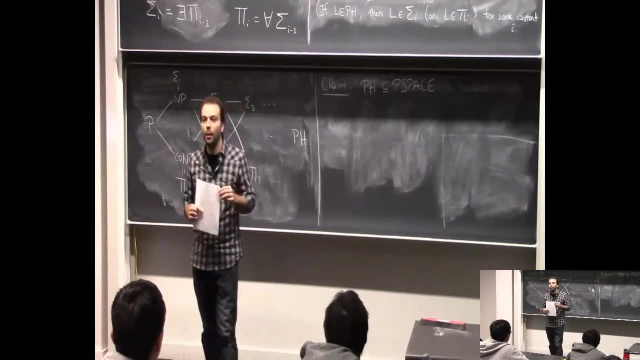 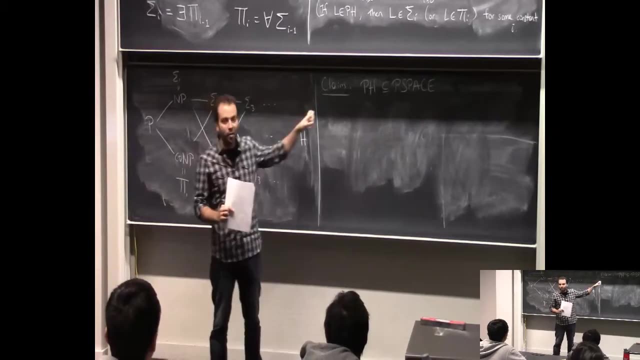 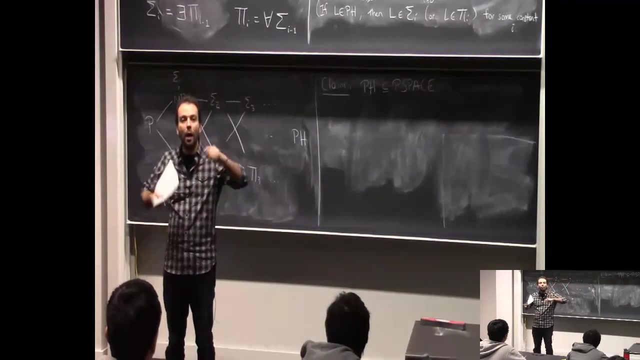 There's one language that it's like the: you can sap, but you can have quantifiers. See, you're talking about the true quantified Boolean formulas, Right? So that's complete for p-space, and that should give you an idea why this is contained in, because there you have like N quantification and how do you show that it's in p-space? 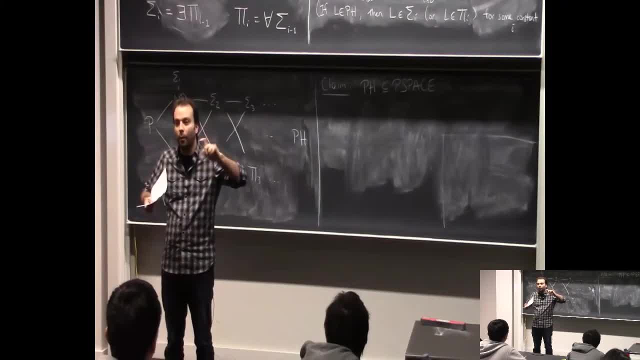 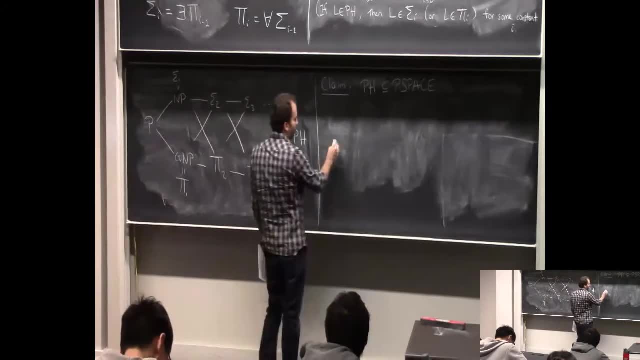 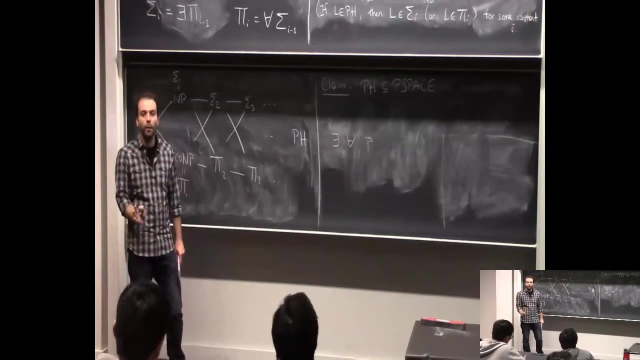 Well, by using the, So you can like, reuse the space for the quantifiers. So, for example, let's take something like: if I said: like there exists for all, and then you have a polynomial machine, just this one. How do you show that this is in p-space? 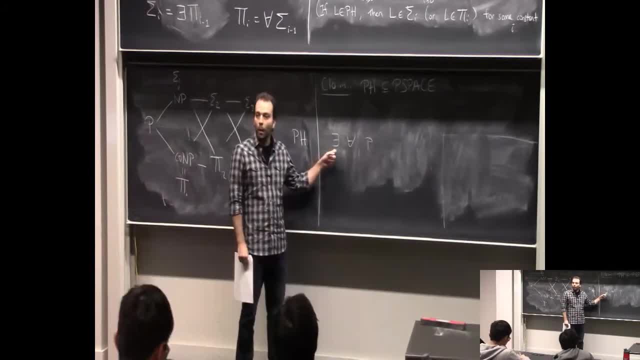 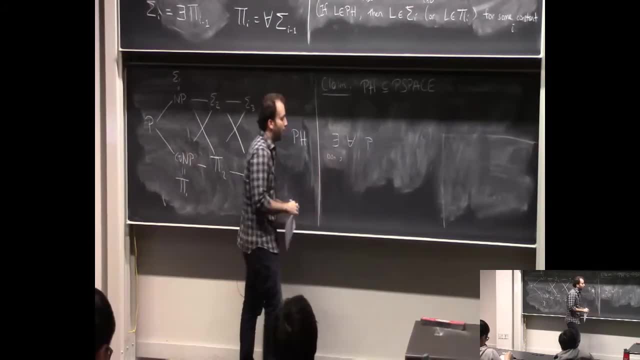 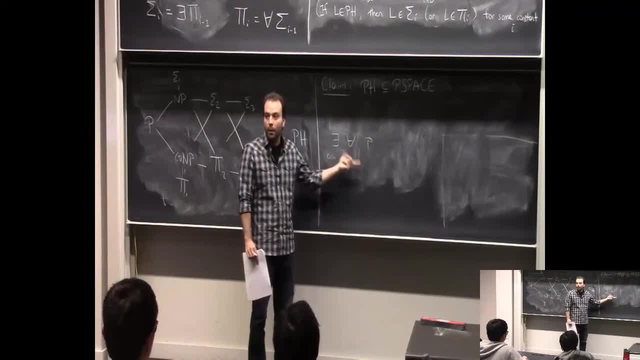 but when they, when you're doing that, going through, you can always reuse that space that you're using, right? so I just need, like, a space allocated for the first variable as another space allocated for the second variable and, as I'm going through each of these possibilities, I just reuse that space. so 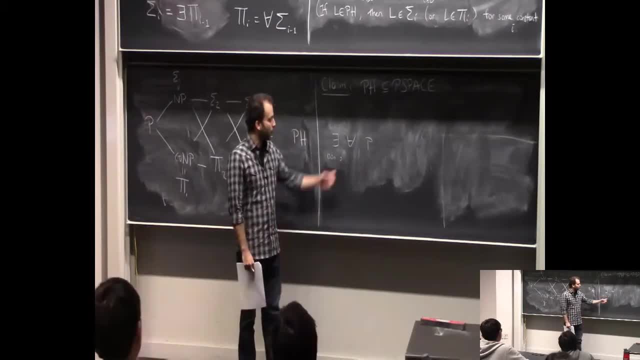 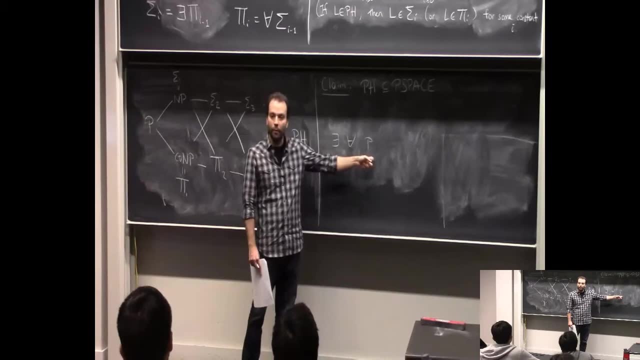 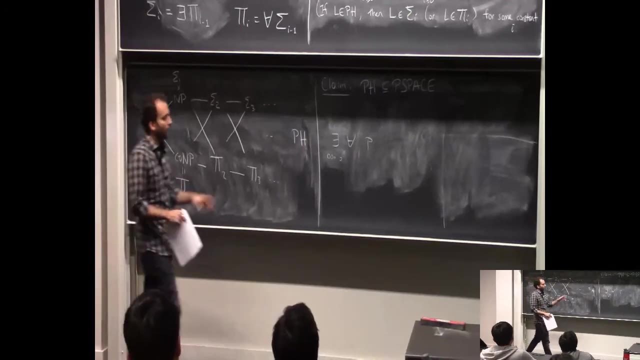 I'm not using more and more space, so you try a possibility there, then you go back here, increment this and then try every possibility there, and so on, so forth. every time you're running your verifier V and checking whether you know you're getting the answers you expect and, of course, if you have constant number of. 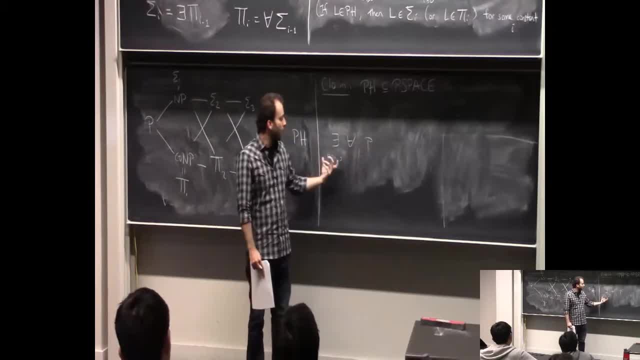 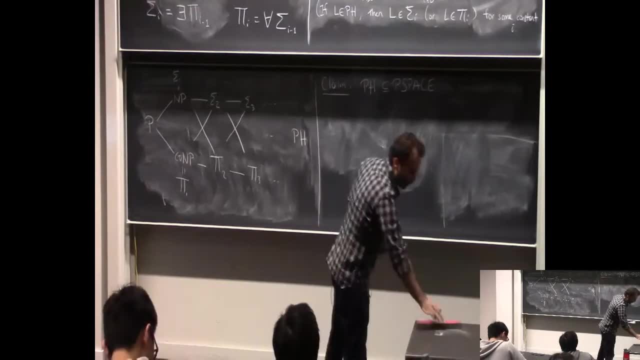 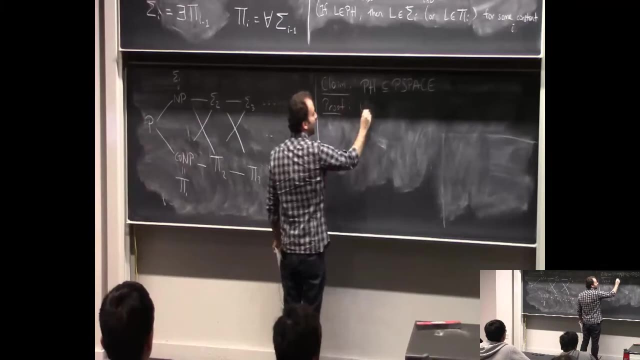 quantifiers, then it's fine, right, so you have constant times polynomial space that you're using. so that's kind of like the idea. so well, if you, you, if you're, if you have nothing to do, I guess you can write it out, but it's not. 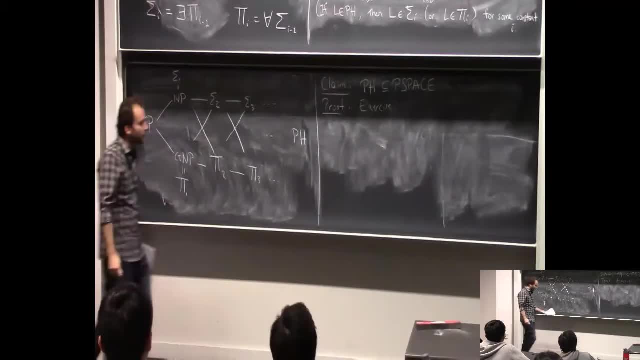 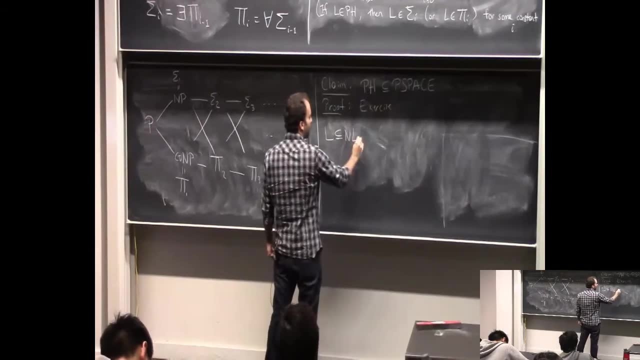 going to be an interesting proof, it's. I mean, I just I just told you what it is okay, so now, okay, let me give you the complexity chain that you might have seen before. L is contained in NL and L is contained in P, P is contained in NP. 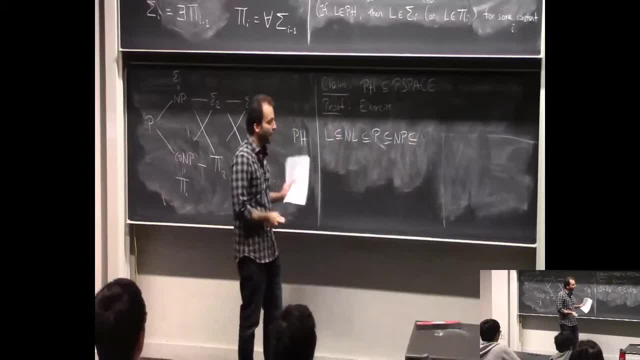 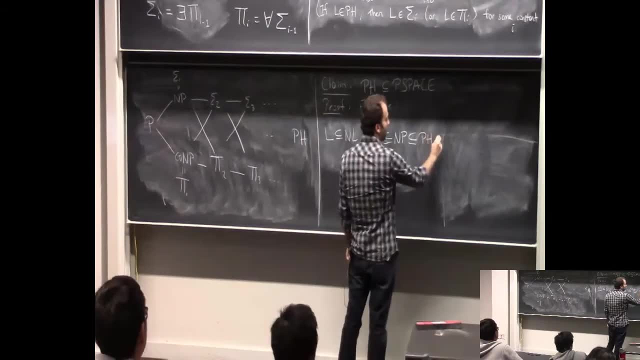 and then here I can like add all the infinitely many guys and sigma i's and pi i's, but let me just put this in here and I'm going to put this in here and I'm going to put pi i's and pi sh is contained in P space, e space is. 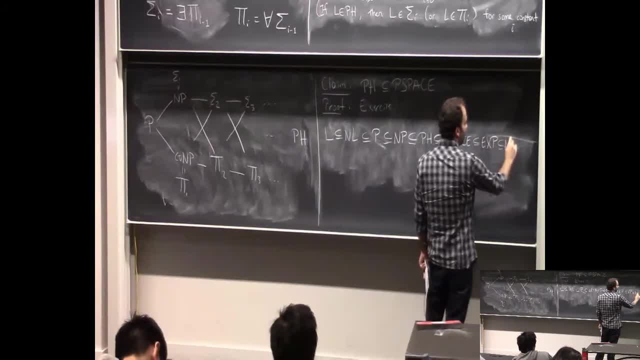 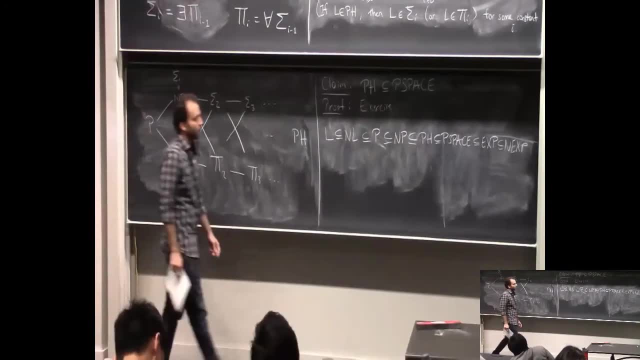 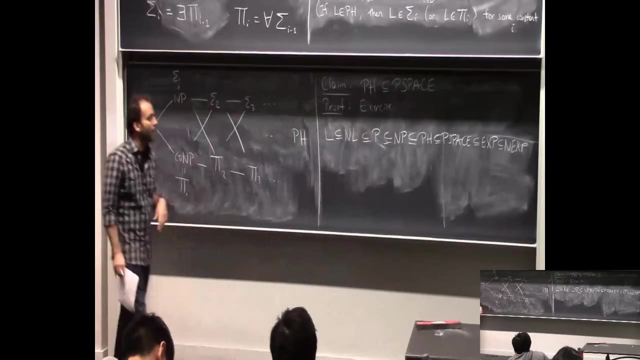 contained in X. X is contained in non-deterministic exponential time, and so on. it goes on. okay, so this, we have put something not between MP and P space. not only that, we put infinitely many actually complex the classes between and MP and P space. okay, So now let's come back here. 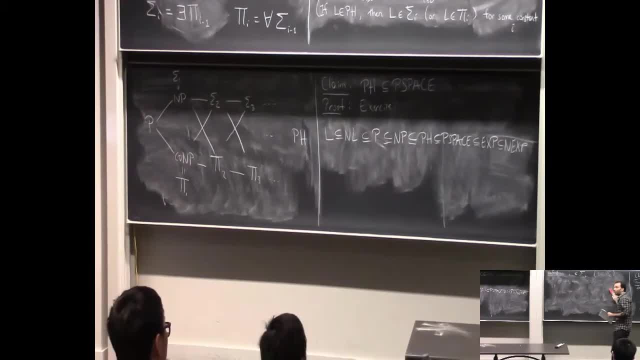 So how many people here believe P is different from MP? You weren't expecting this question. How many believe it's equal? Anyone believe they're equal? No one. So here's, I'm going to now give you, show you, a result that kind of you can take it. 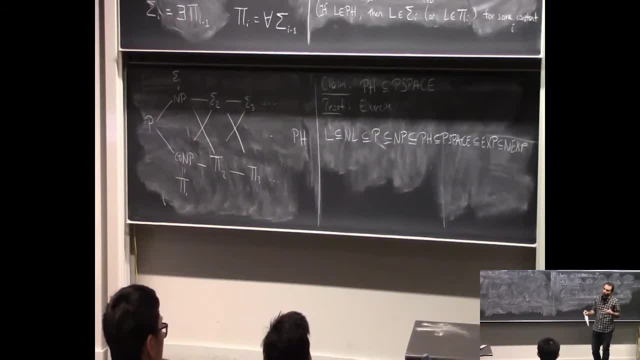 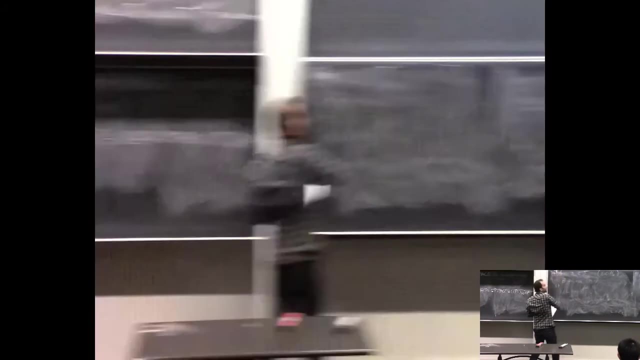 as maybe more evidence towards you know it's believing P is different from MP, if you will okay. So yeah, here we go. So the theorem is: and yeah, I don't have half an hour left. 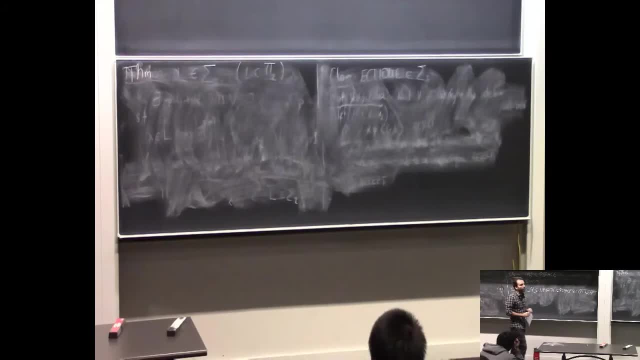 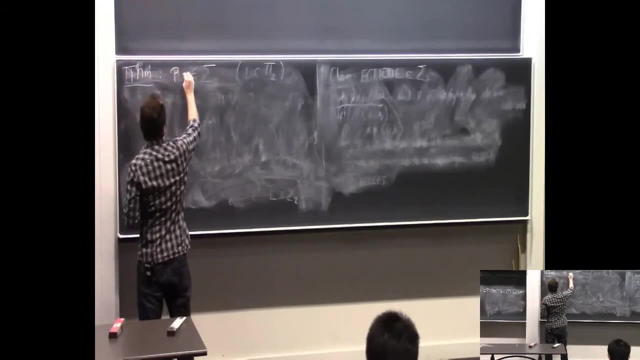 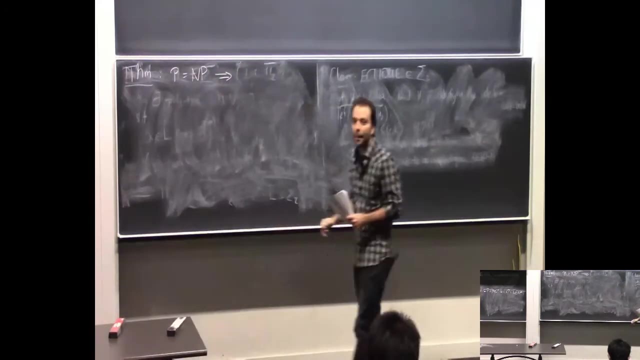 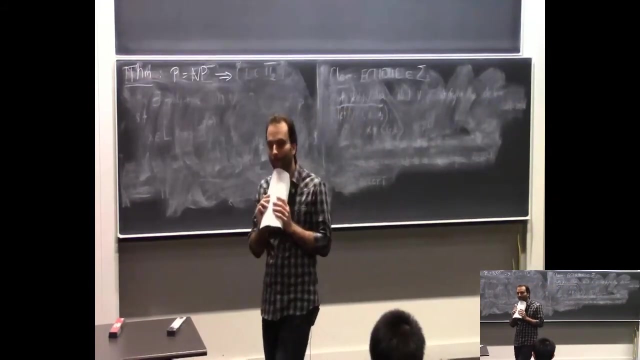 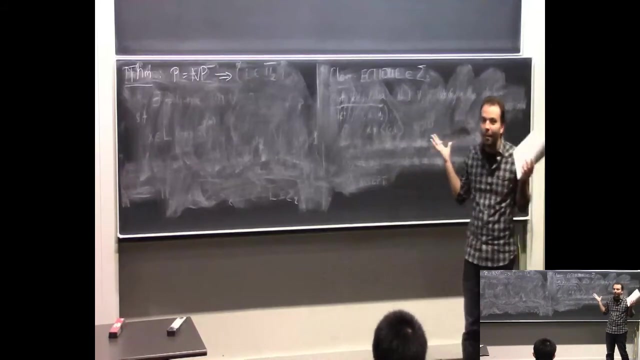 Yeah, I'll probably give you like the sketch of the proof, without doing it very formally, But okay, so the theorem is: P equals MP implies. anyone can guess what it implies: P equals MP. it's something related to polynomial hierarchy, obviously. 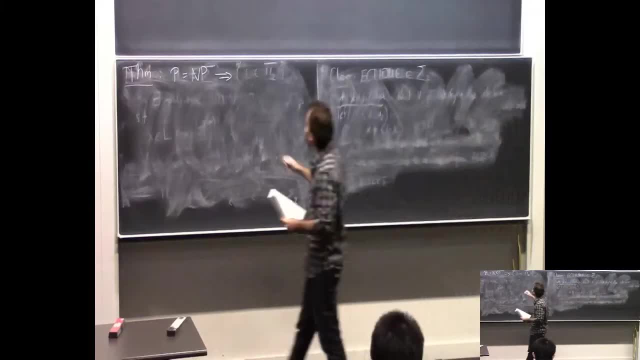 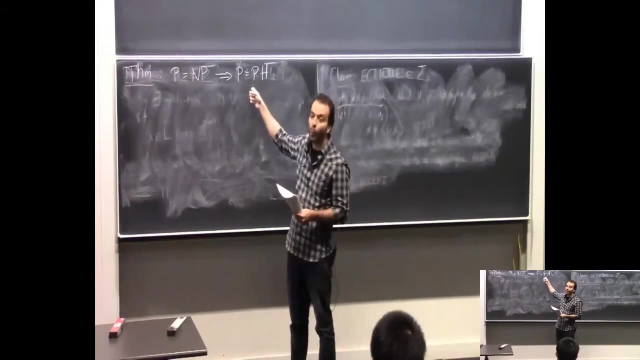 Yeah, Yes, exactly, P equals PH. Okay, So, if you can show, P is equal to MP, the polynomial hierarchy- and I mean the way people like to phrase this- is that the polynomial hierarchy collapses to P. okay. 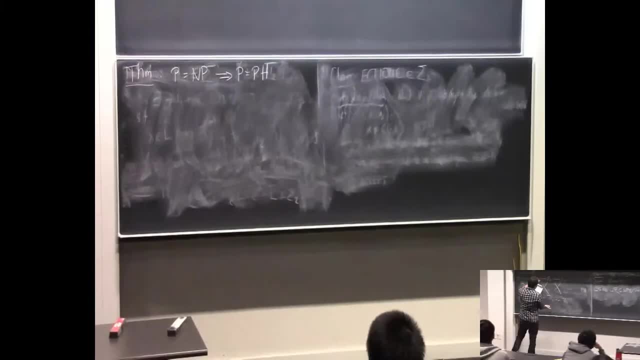 People like to usually draw this picture. I'll draw it this way. People like to draw it like this way, where, like, the hierarchy goes up and then you're saying, oh, everything crumbles down to P if P equals MP. 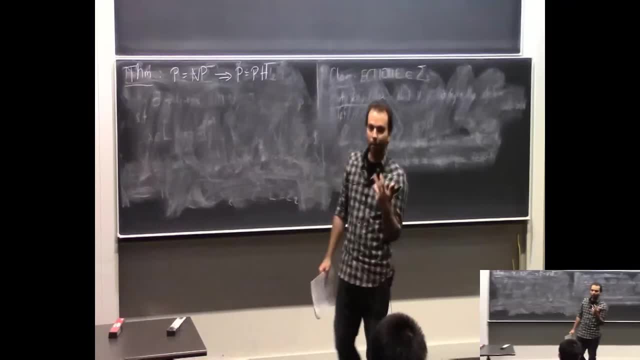 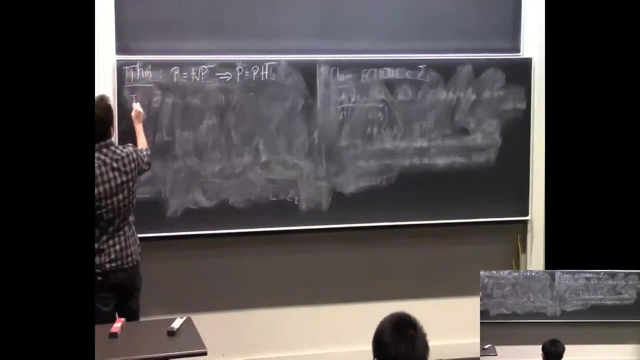 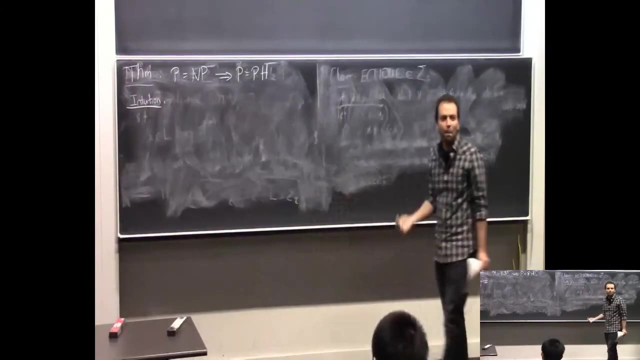 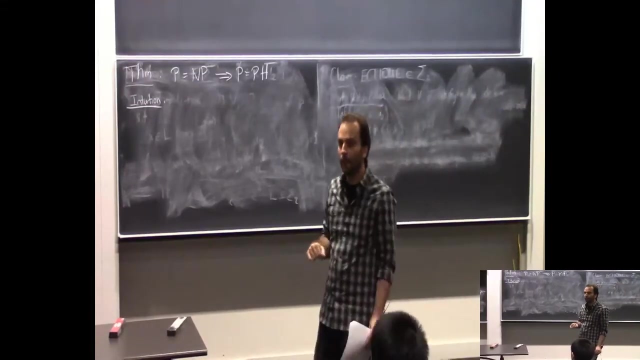 So what was the intuition? Do you? why do you think this is true? I'm going to give you the intuition. What does P equals MP mean? in some sense, P equals, there exists P. yeah, Sigma 2 is equal to pi 2.. 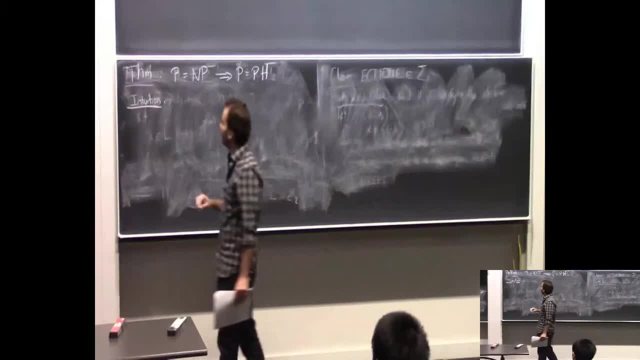 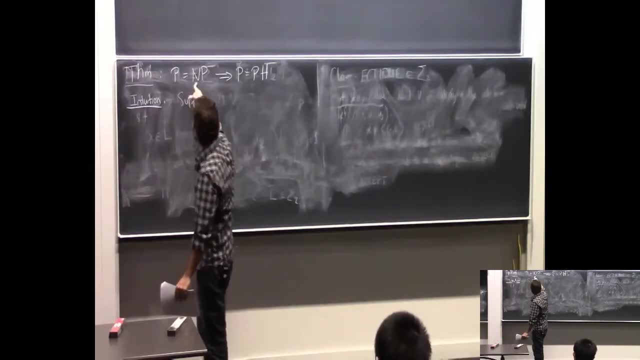 Right, but why? Sigma 1 is equal to pi 1.. Right, So that's right, So suppose. so the point is that MP is there, exists P, and you're saying there exists, P is equal to P. So you're kind of saying: 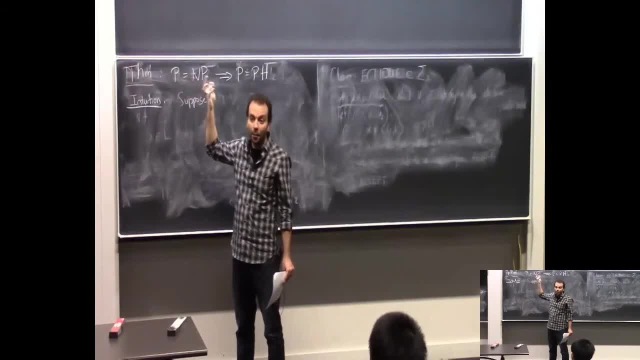 you know what I can just get rid of, that there exists quantify in some sense, okay. And the second thing is: if P equals MP, then that equals co-MP. right, That's what we saw somewhere. I think I wrote that if P equals MP, then MP equals co-MP. 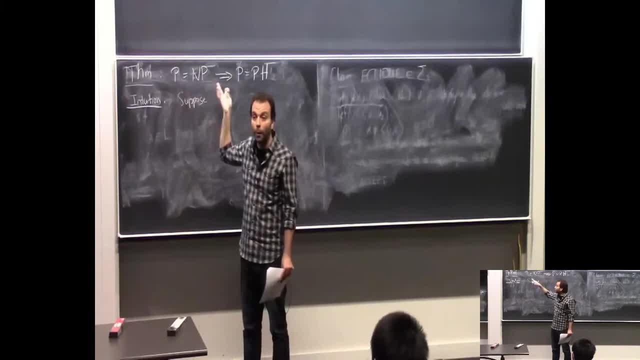 So then you're saying P equals co-MP and co-MP is for all P. Then you're saying P is equal to for all P. So now you're also telling me: I can also get rid of this- for all quantifier too. 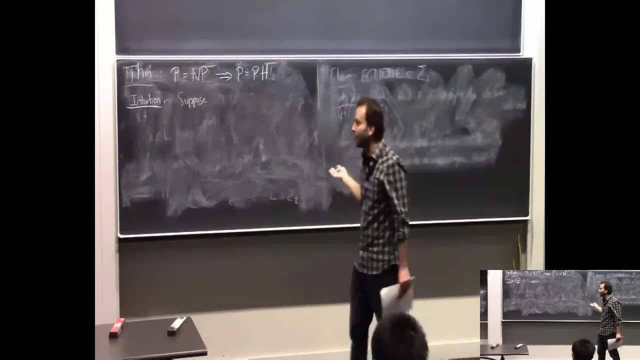 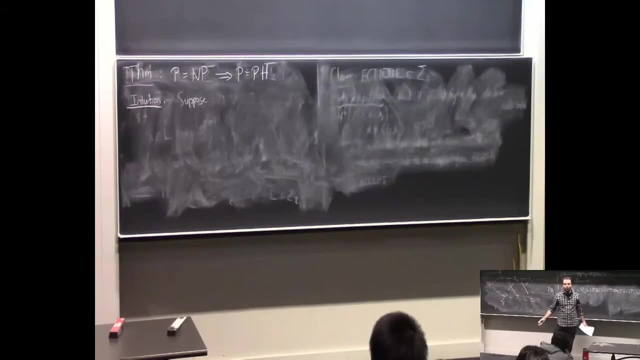 So I can get rid of the exist quantifier. it's going to get rid of for all quantifier, So I just keep getting rid of them. So wherever you are, you can just keep getting rid of them and go down to P. That's the intuition. 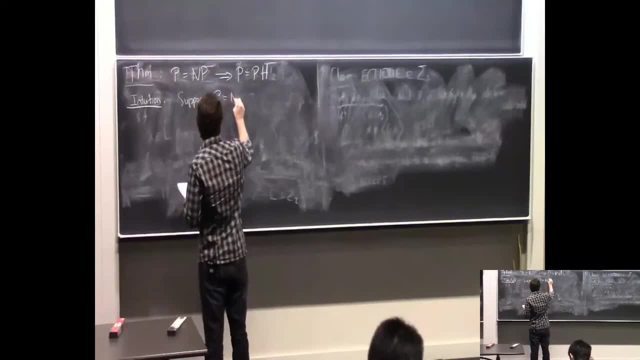 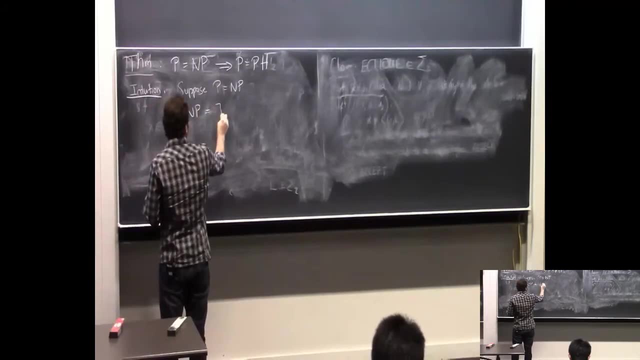 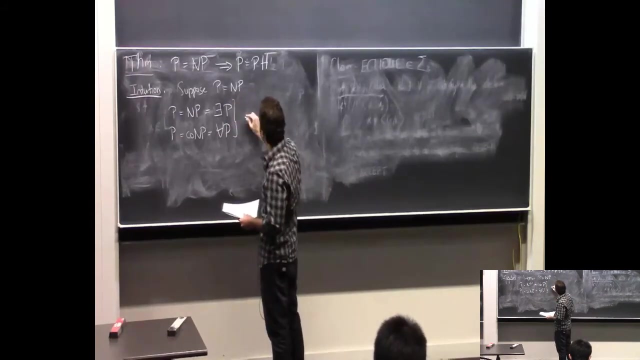 Okay, so suppose I mean, let me write this down: Suppose P equals MP, Then We know that P equals MP, which we characterize as there exists P, and then also P equals co-MP, which is for all P. So here the implication is that we can get rid of there exists and 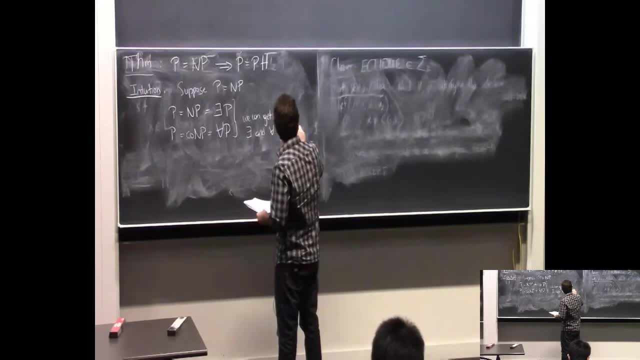 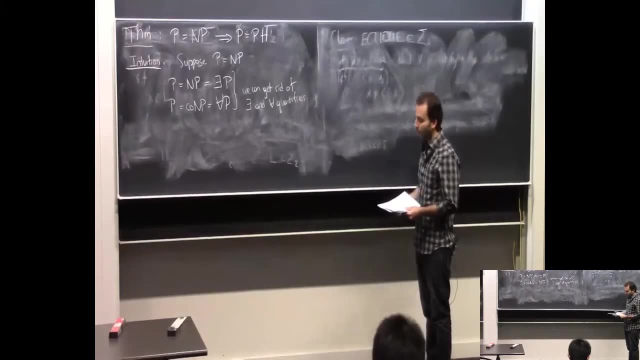 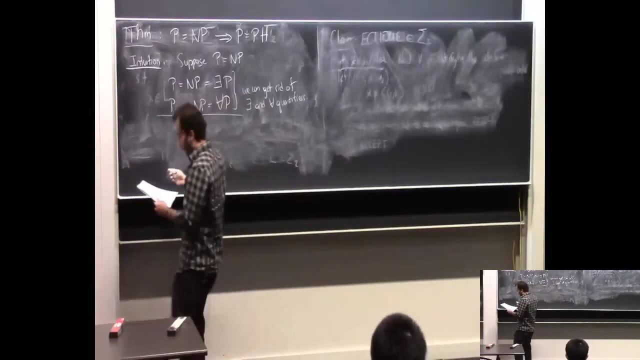 for all. So we want to get rid of the exist quantifiers. Okay, look, this is not a proof, This is just like the idea, But it's a very accurate intuition, So okay, so if you have now, let's say there exists. so let's take, like, sigma 2.. 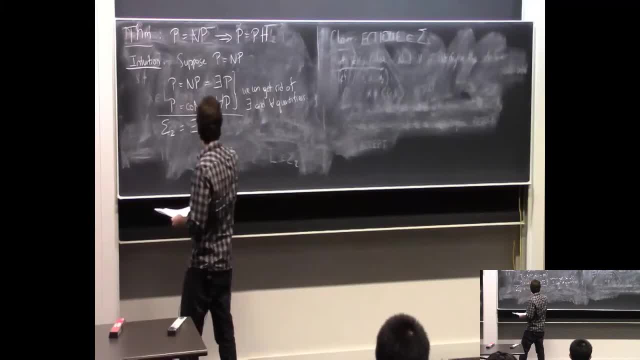 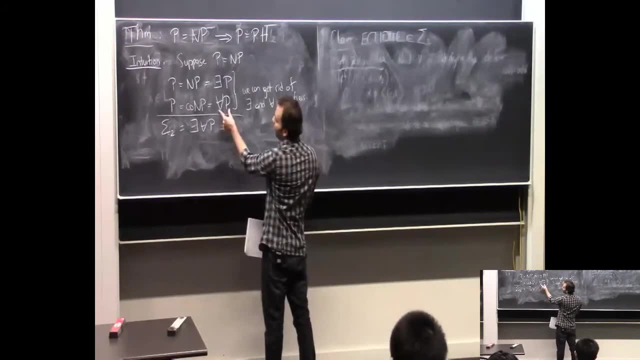 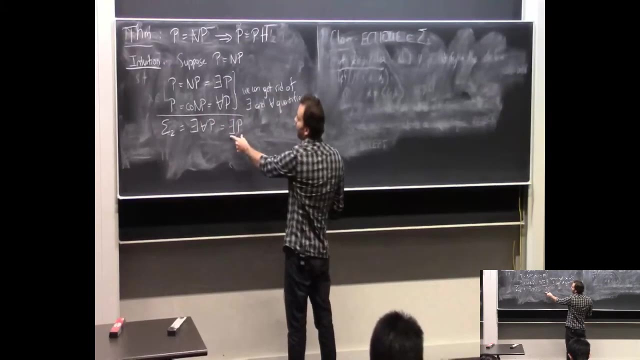 Sigma 2 is: there exists for all P, So there exists for all P. but now I know for all P is P. So this is like there exists P then And there exists P is NP, which is P. And if I look at similarly for pi 2, this is for. 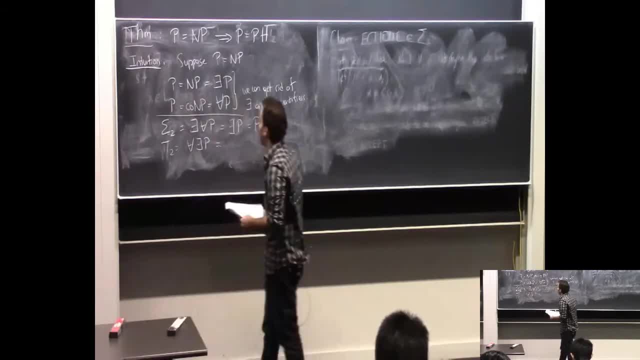 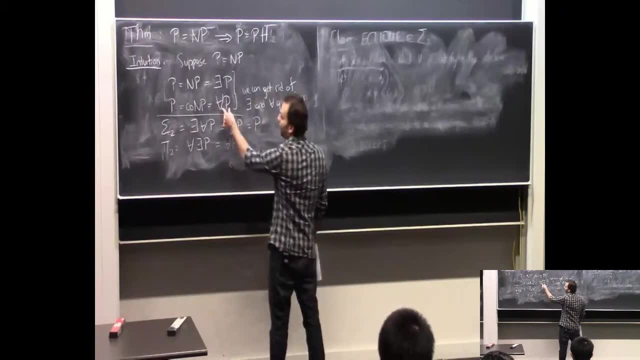 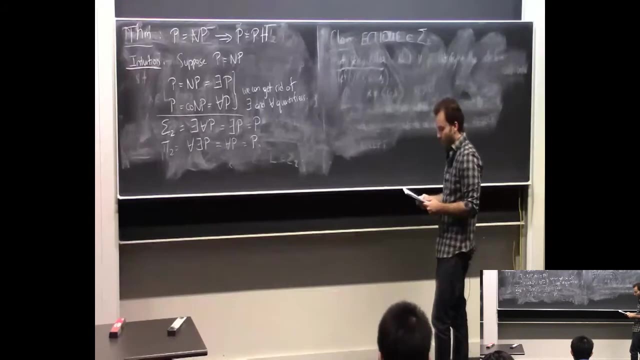 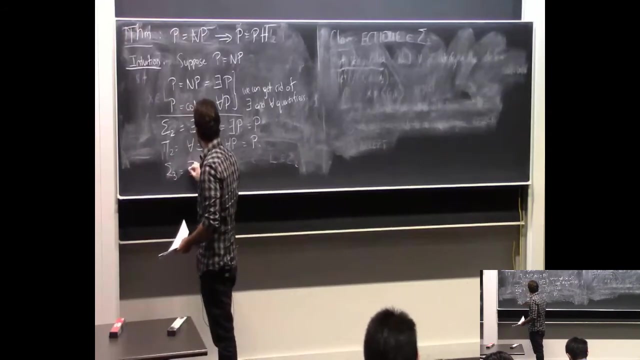 all there exists P, but there exists P is P. So this is like for all P, but then for all P is P. And yeah, I mean, let me do maybe one more. Sigma 3 is there exists. for all there exists P. 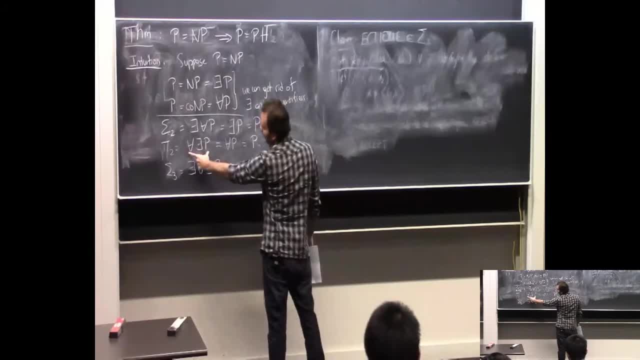 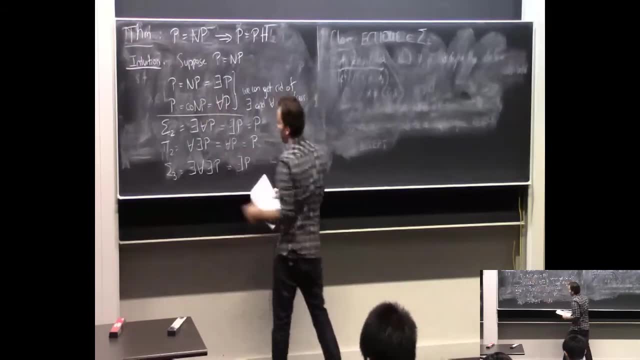 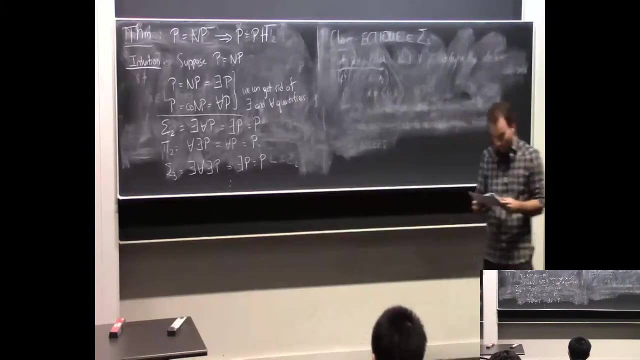 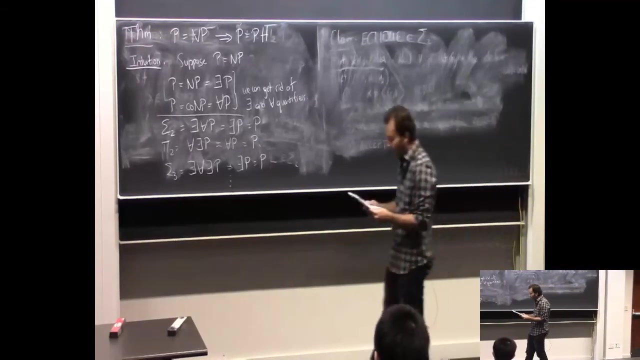 But now I've shown you that That, for all, there exists P is P, So that makes this: there exists P, There exists P is P, And so on. Yeah, I'm not going to have time to prove this formally, So yeah, so to prove this formally, you can basically do an induction proof induction. 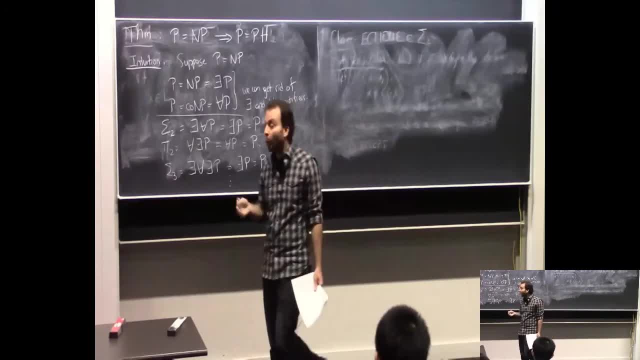 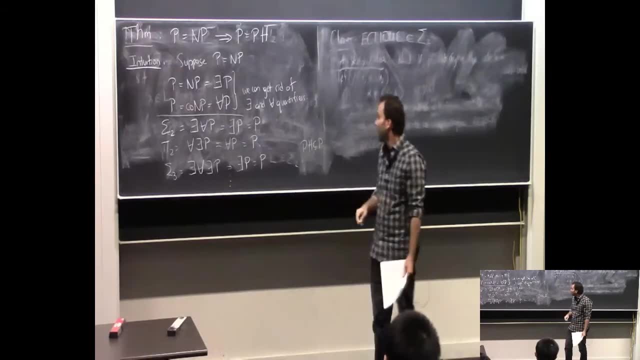 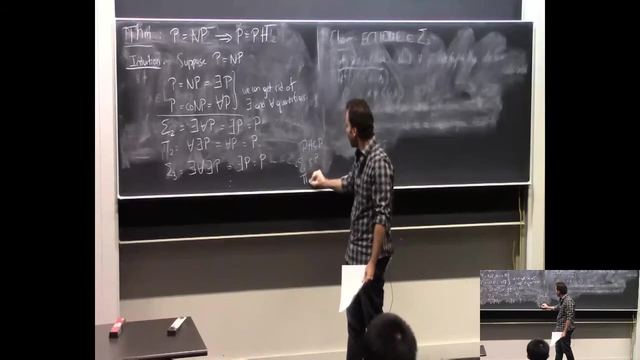 on the i. Okay, So you want to show basically that pH. you want to show pH is in P. So for each i, you want to show that sigma i is in P and pi i is in P, And then you show it by induction. 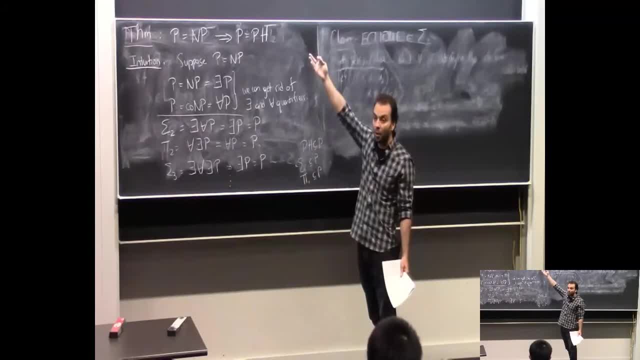 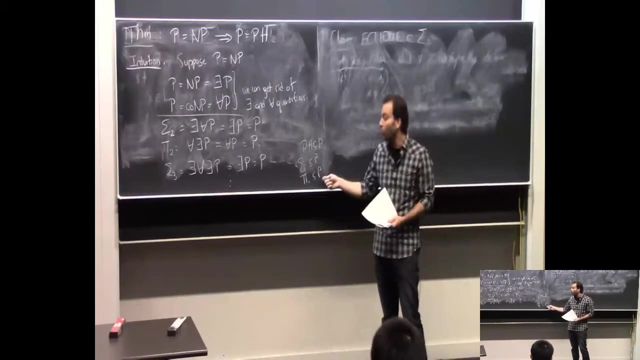 on i. The base case corresponds to basically, the assumption that P equals NP. That's yeah, that's pi 1 and sigma 1.. And then now, assuming that sigma i minus 1 is in P and pi i minus 1 is in P, you can: 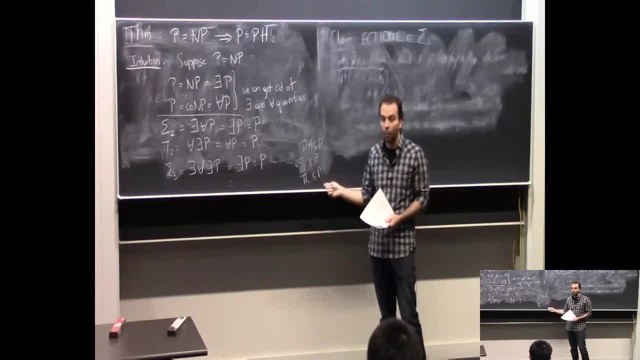 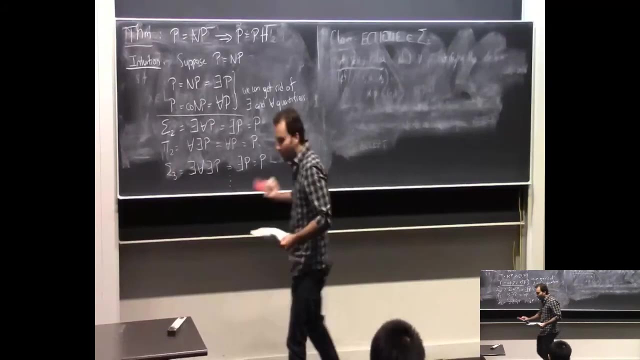 show that sigma i is going to be in P and pi i is going to be in P. I think you can believe that So, and you know, there's a way to formally do this Good. Moving on, Here's another related 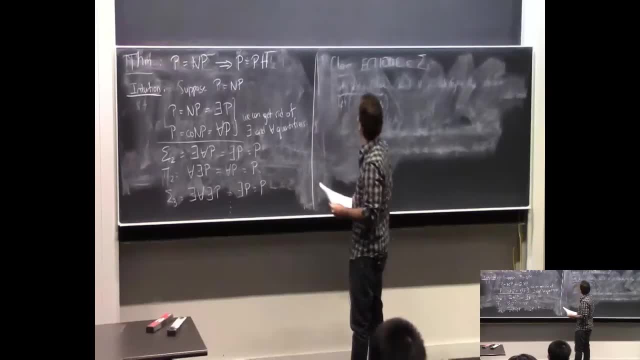 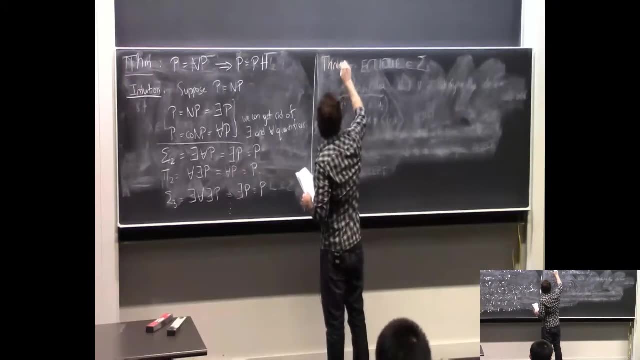 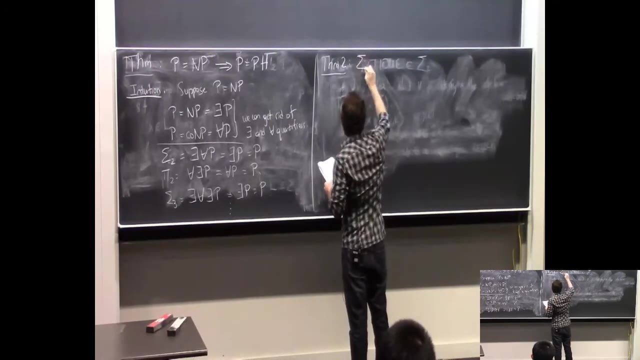 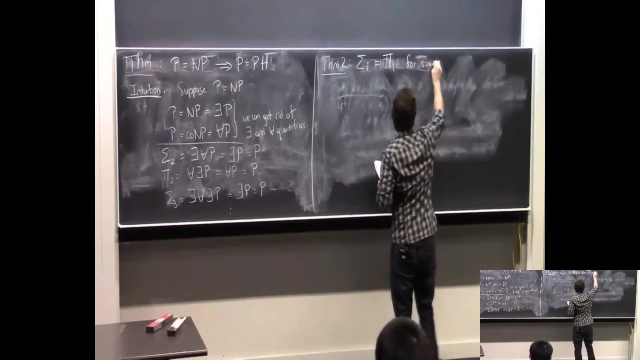 Okay, Okay, So you can use your theory. this is theorem. This is theorem. theorem two with a similar proof. So this is like: if sigma i equals pi i, for some i, then what do you think happens? So what's the? what you will do? 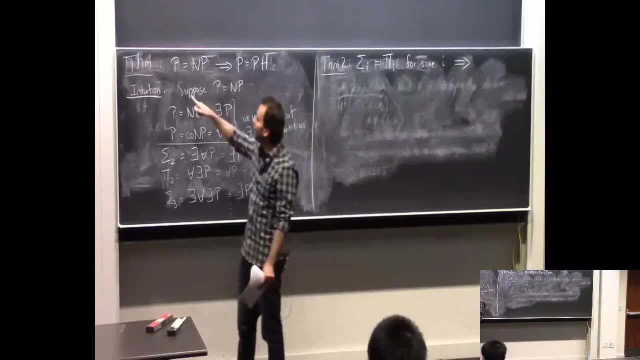 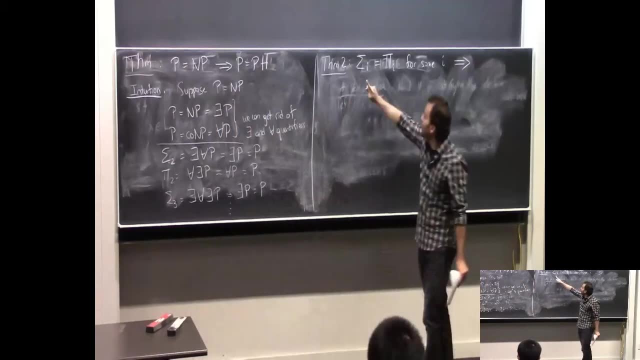 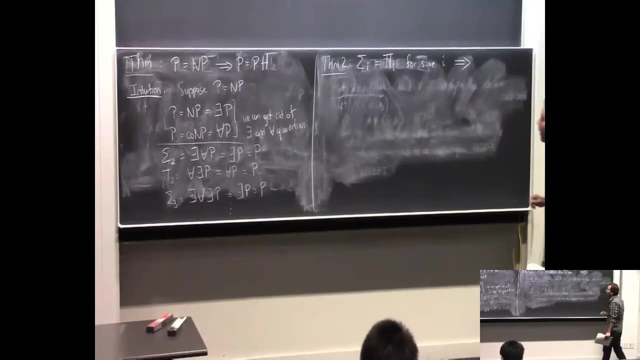 You can show it. okay, here we were like: okay, this is like. Sigma 0 equals Sigma 1. this is now Sigma I equals PI. I like, if you take I to be one, for example, a special case of this would be, let's say, MP equals Co MP. what do you think would happen in that case if MP equals? 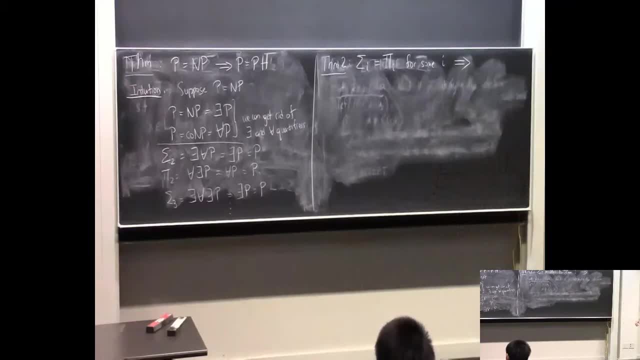 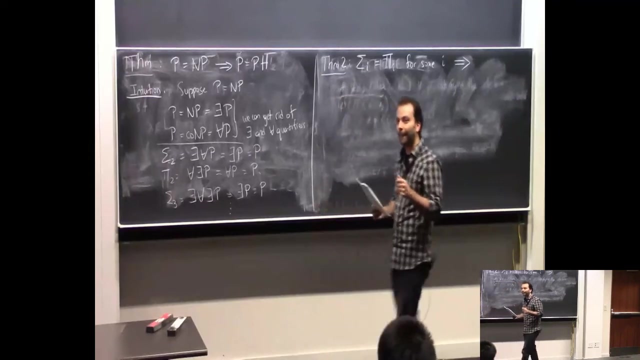 Co MP. any guesses what might be the answer? yeah, to equal to. so everything. everything pH becomes- and pH already contains everything below. everything collapses to Sigma. if it was MP equals Co MP, everything collapses to MP, which is equal quant. yeah, so again, this is like saying people like to say: 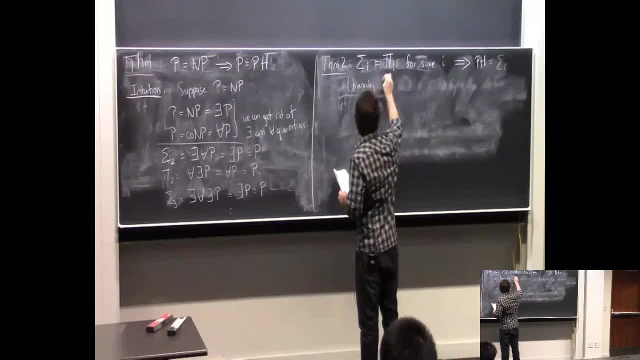 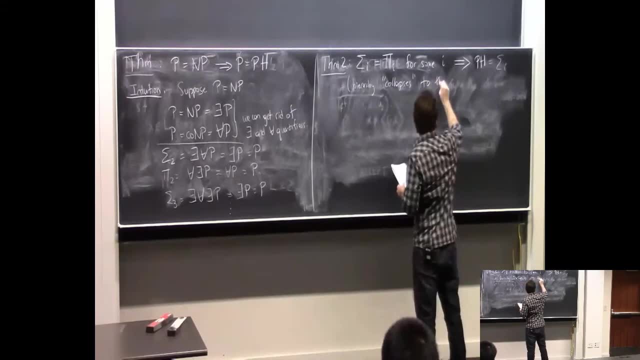 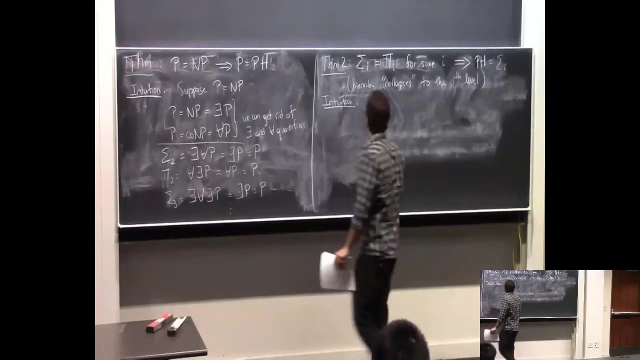 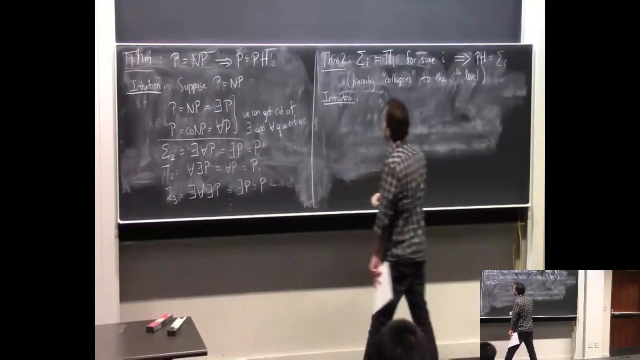 the hierarchy collapses to the ith level. okay, so again I can give you do intuition which is going to be similar. so here let me demonstrate it with: MP equals quantity, but it's the same idea. so suppose, and P equals coin P, then I want to show that pH equals MP. so this, what does this? 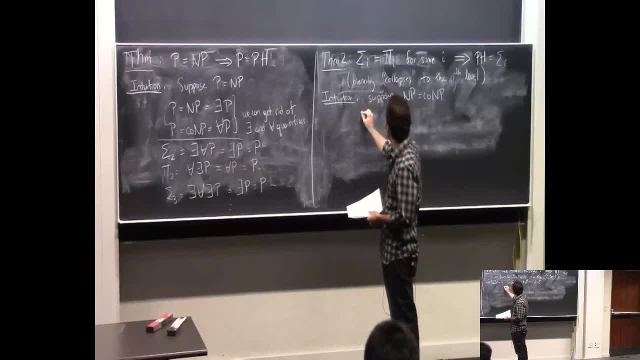 mean again, like when you write it in this way, you know, things become clear. so you know that there exists P equals for all P. so if they exist, P is for all P. then if I now look at there exists for all P, then what can I say? well, this for. 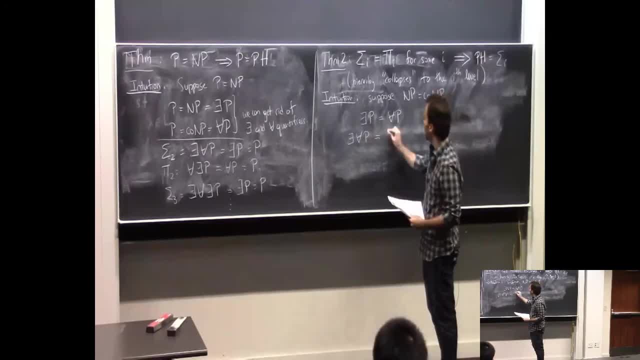 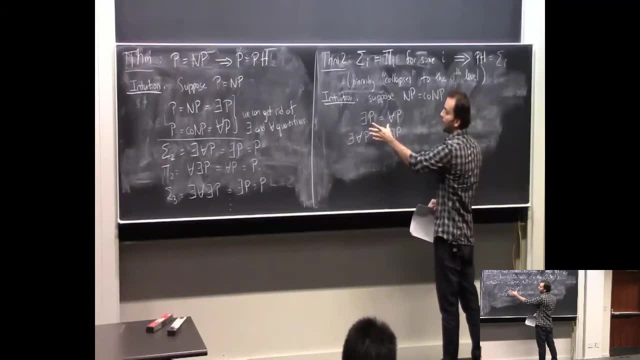 all P is there exists P. so now I have there exists, there exists P. okay, so I was able to switch. so this allows me basically, as you can see, switch a there exists quantifier to a for all quantifier in some sense. so I, when I have there exists for all P, now I have there exists. 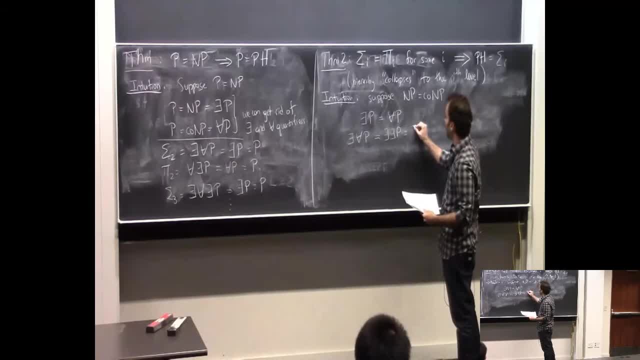 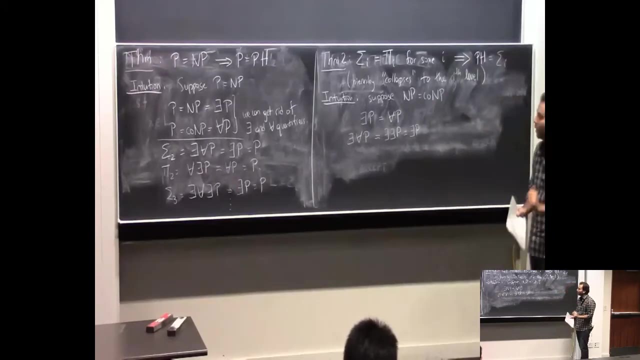 there exists P, and now this is equal to there exists P because, as I mentioned, based on your question, right, if you have two, there exists in a row you. there is this, you one. there exists you two. you can combine them into one. there exists quantification for one variable and similarly, for all, there exists P. if I 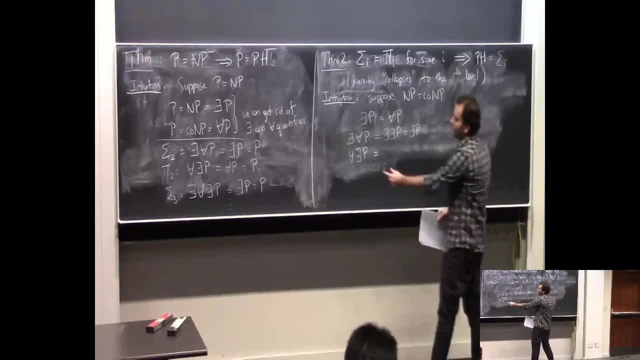 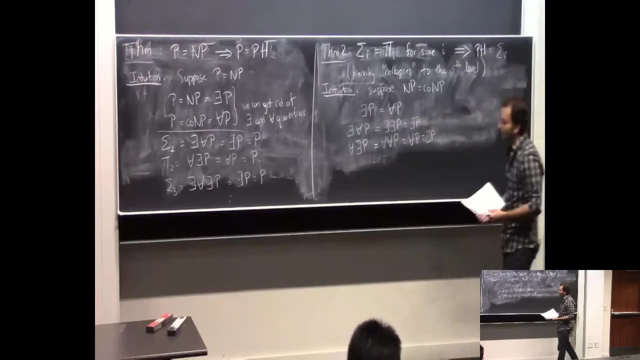 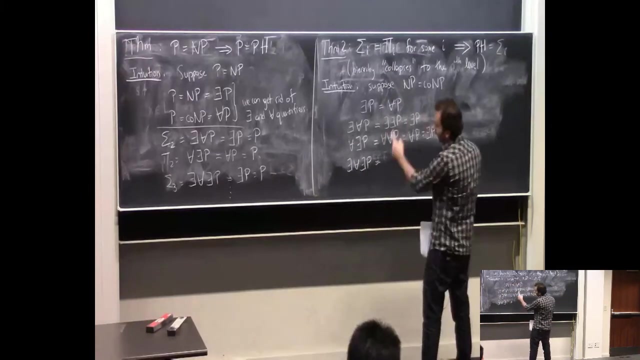 look at this. well, there exists P, is for all P. so this allows me to say this is for all, for all P, which is for all P. okay, which actually is, there exists P. and you know, let me do one more: there exists for all, there exists P. well, now, I know from the previous part that for all there exists. 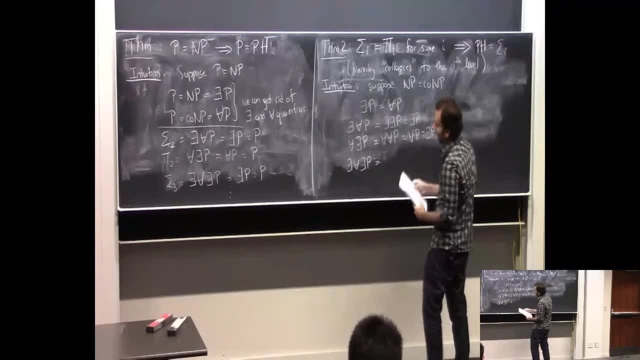 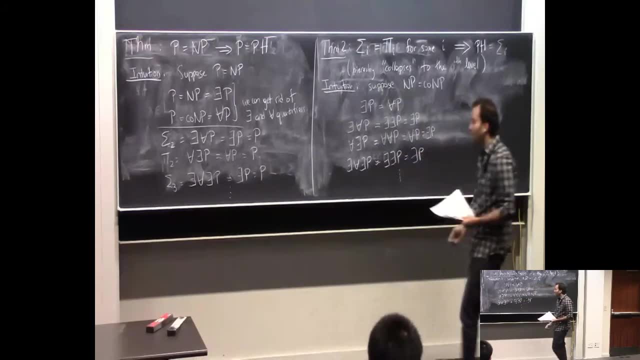 P is equal to there exists P, so this is there exists. there exists P, which is there exists P, and so on. okay, so no matter what I level I go in, I can collapse it to there exists P, which is MP. this is because I started from: MP equals co MP. 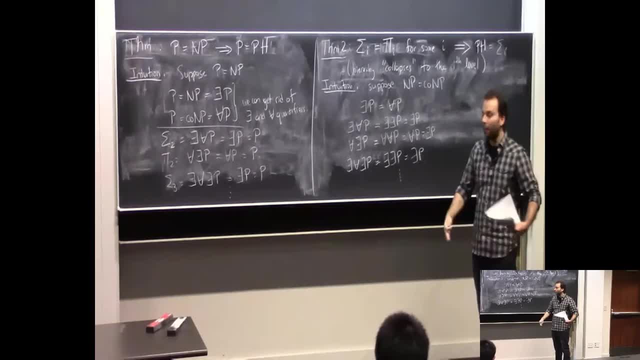 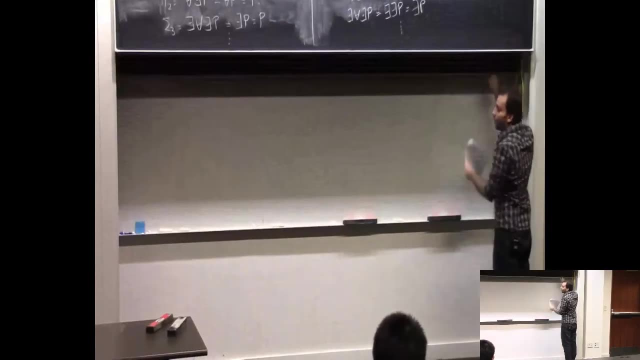 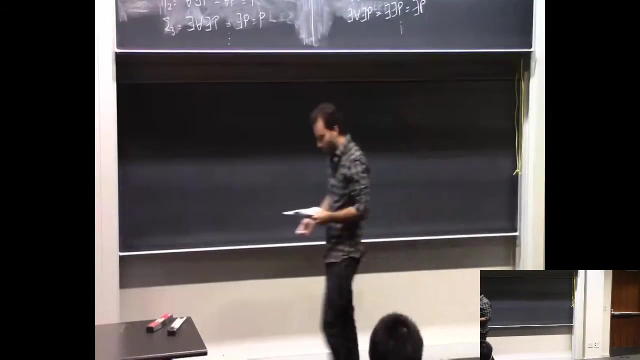 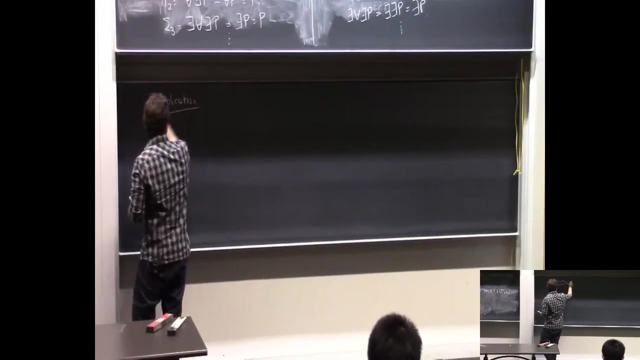 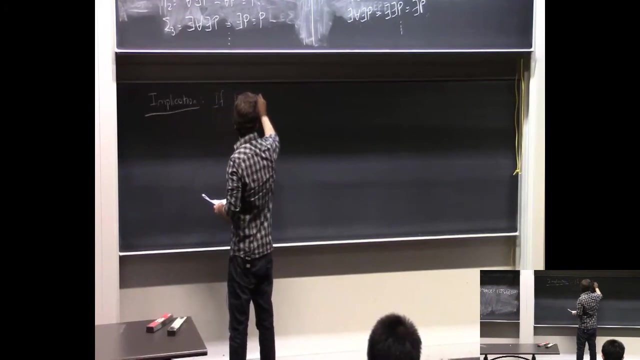 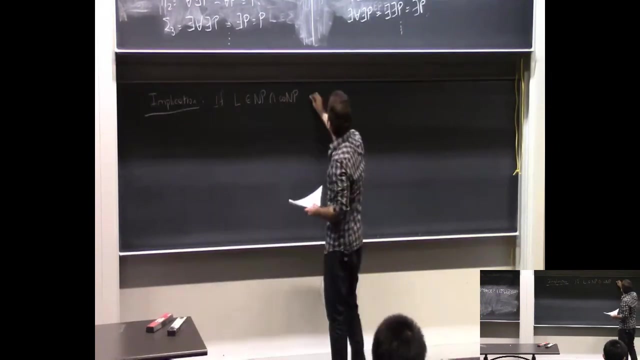 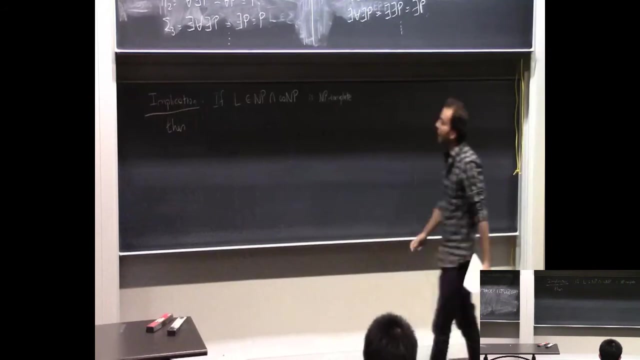 if I start at a deeper level, we can do the same thing and collapse it to that level. so is an implication of this: if L is n, if L in MP intersection coin P is NP complete, then so if you have a language in MP intersection, climb P, that's MP complete. 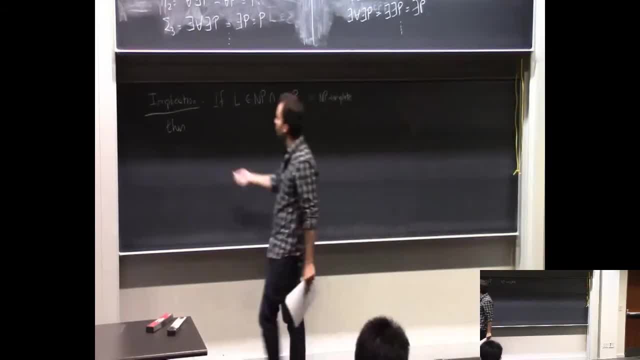 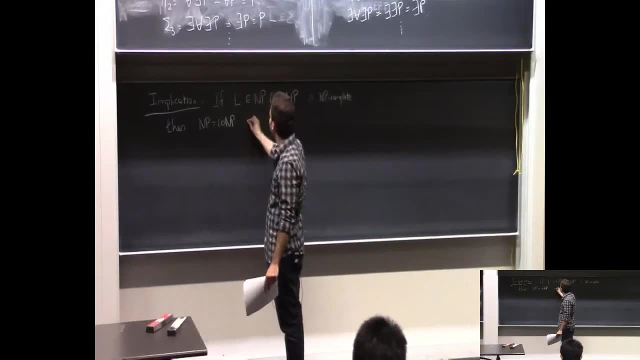 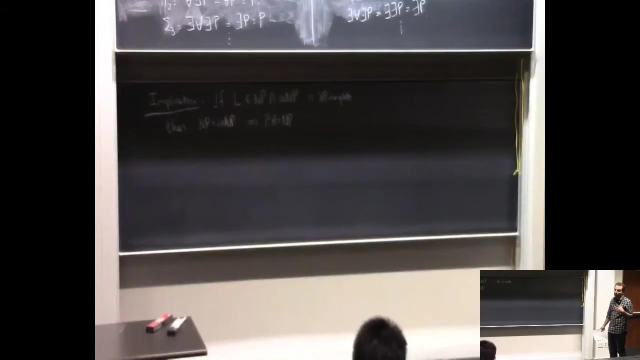 then you can actually show that MP has to be equal to Co MP, which then implies, as we just saw, and pH equal. okay, so then, if you don't believe- and most people do not believe, so maybe I should make a comment about that- what experts believe about the polynomial hierarchy. so people believe that each of these levels are: 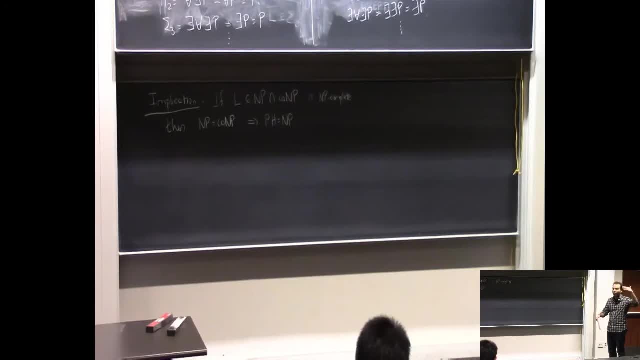 distinct, like you have different complexity classes, larger and larger complexity classes, and that the polynomial hierarchy is not expected to collapse and and you can see like here, you can take this as evidence that we don't expect a language in MP intersection climb P to be MP complete. okay, because if that 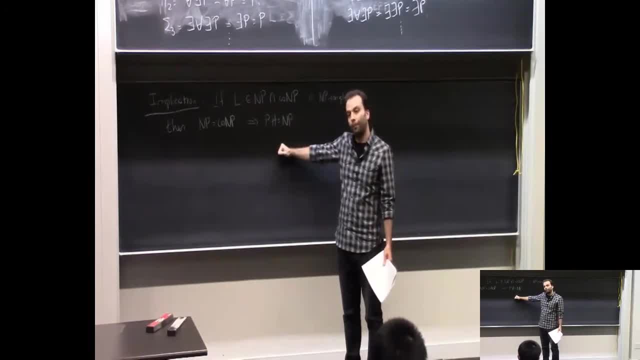 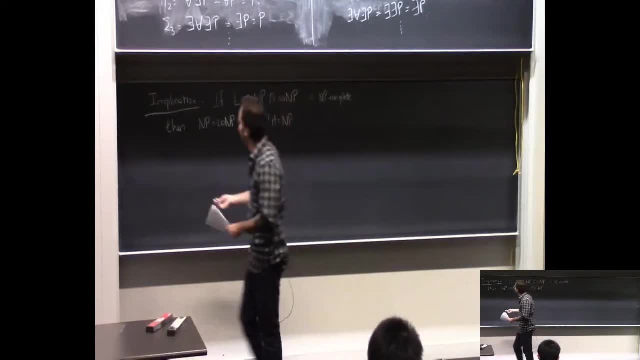 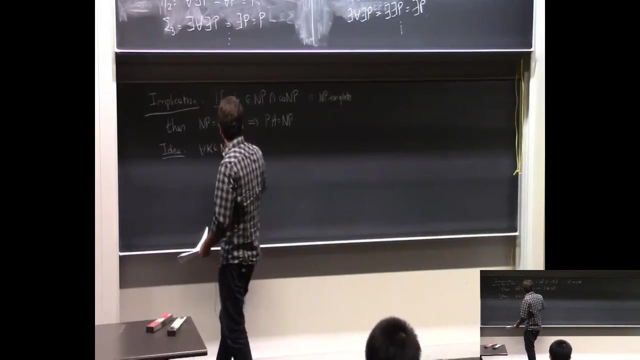 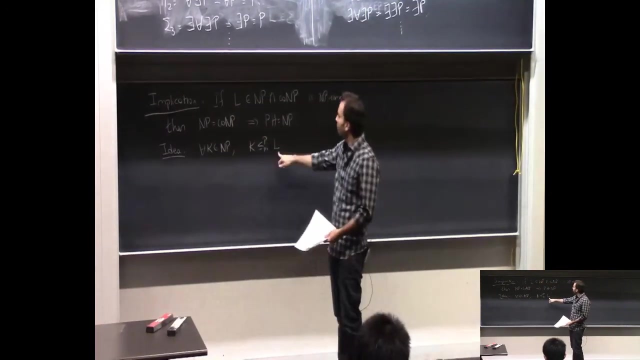 happened, then the whole hierarchy would collapse to MP. so a good example of this is, by the way, let me just like the idea of this is: what's the idea of this? so if, if, if L is MP complete, then for all K in MP, K reduces to L, but now L is in Co MP, so that implies 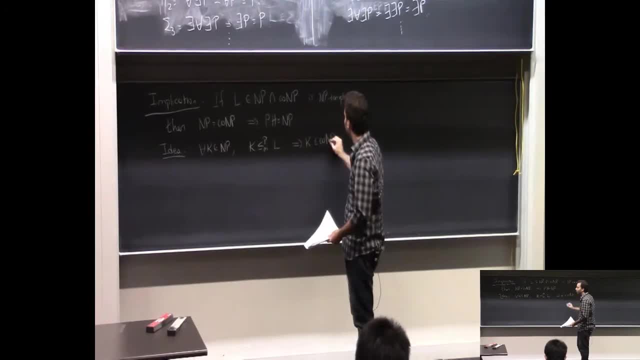 K is in Co MP. I don't know if you've seen this. have you seen this? like? if you, if K reduces to L and L is in MP, then K is in MP under these reductions. Similarly, if K reduces to L and L is in. 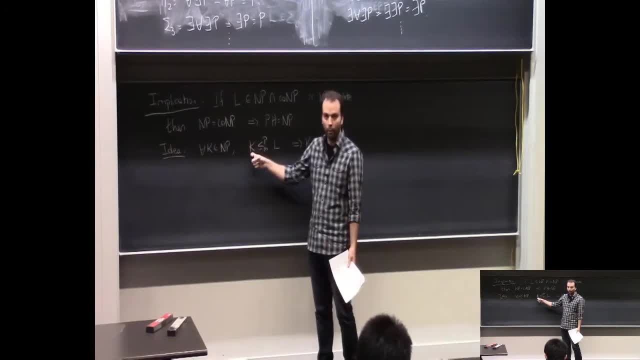 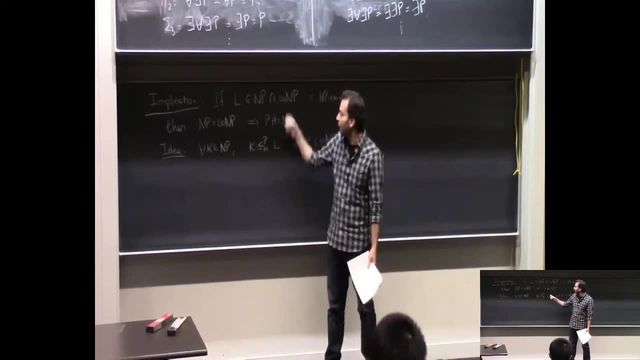 co-MP, then K is going to be in co-MP. You can also show that. So that's what I'm using here. K reduces to L, but I know L is in co-MP, so that means K is in. 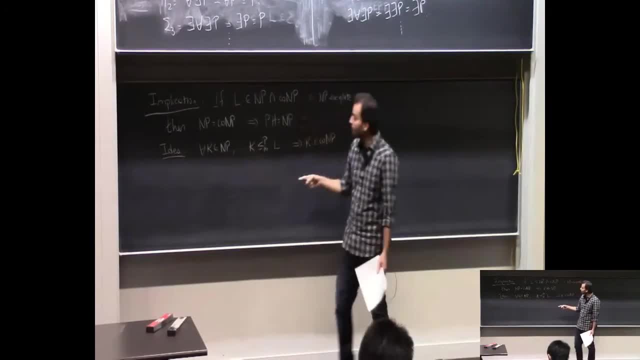 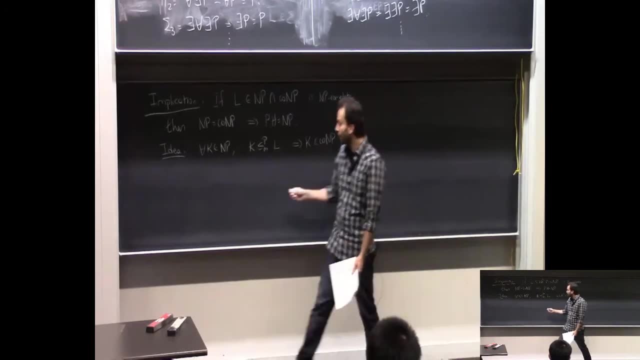 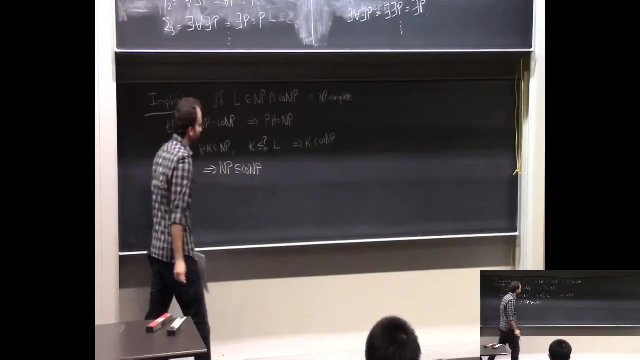 co-MP, But this is true for all K in MP. So that means all K in MP is also in co-MP. So MP is contained in co-MP. Okay, so this implies that MP is contained in co-MP And that actually implies from that. you can also: 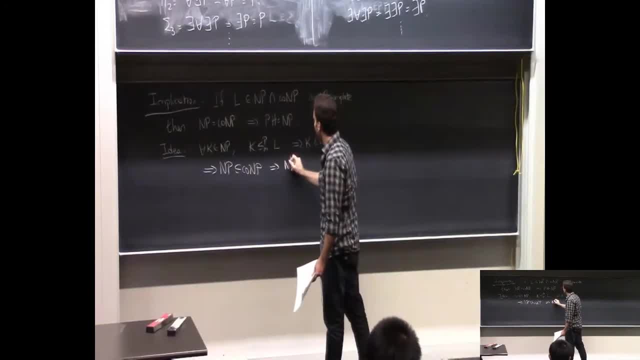 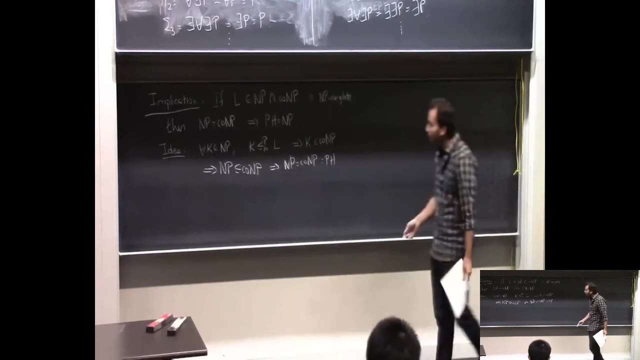 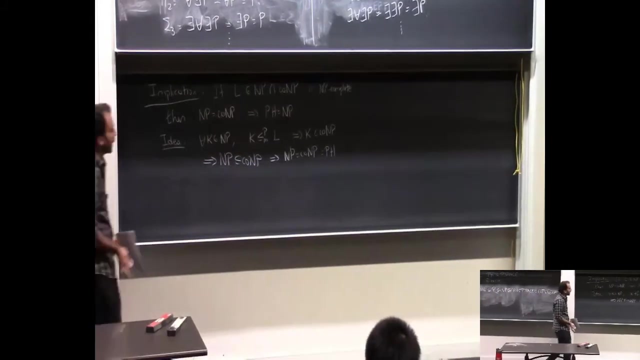 derive the other direction. MP equals co-MP, Okay, and then by this theorem that would imply it's equal to pH And yeah. so a good, good example of this was like: let's take like an integer factorization, Okay, very. 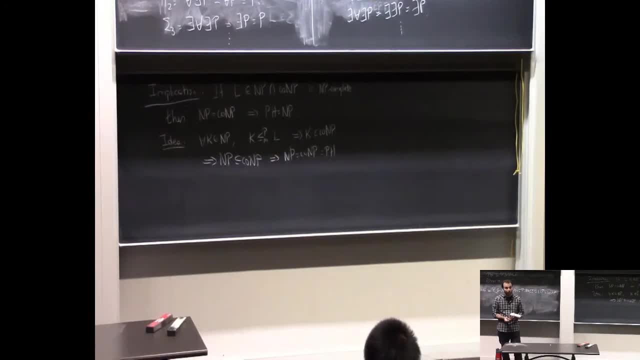 important problem in computational complexity. We hope it's hard problem because many of the crypto systems rely on the assumption that it's a hard problem. Now it would be great if this problem that we hope is hard is actually MP complete. That would give us more confidence. 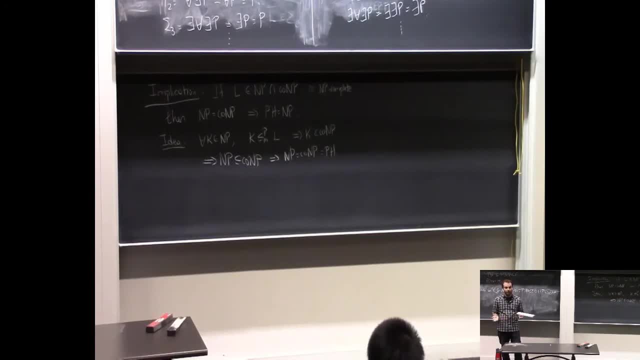 that it's actually hard. So then you could say: if P is different from MP, then we know factoring is hard, But unfortunately factoring problem. well, factoring problem is not a language, but the language version of the factoring problem is an MP, intersection, co-MP. So we don't expect it to be MP complete In. 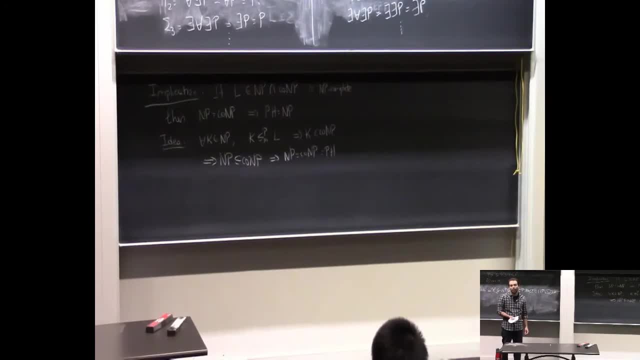 fact, we don't expect to be able to base any of crypto systems on the hardness of an MP complete language. So that's kind of sad, but yeah, so let me just say that. Let me just give you this example very quickly. So if we look at like a decision, 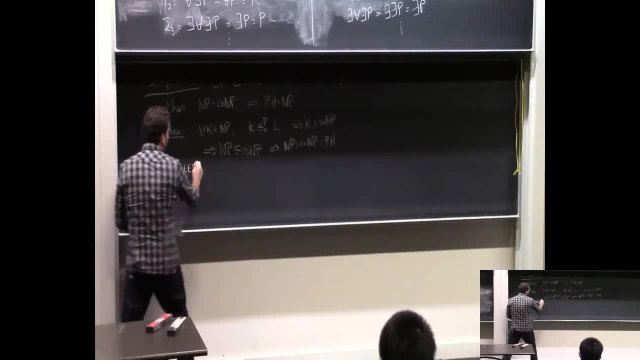 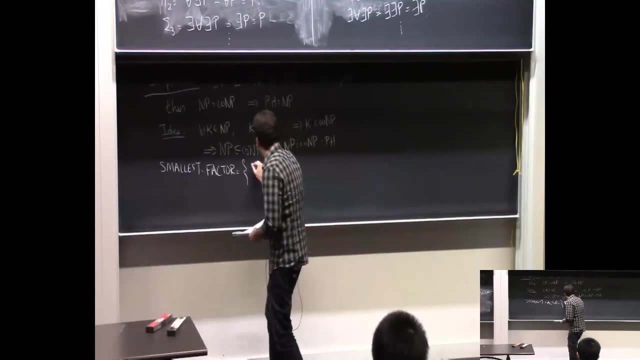 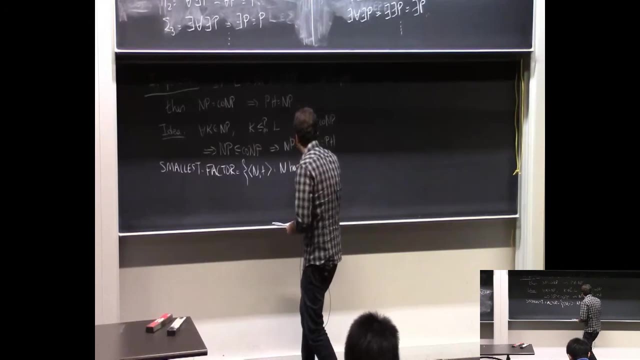 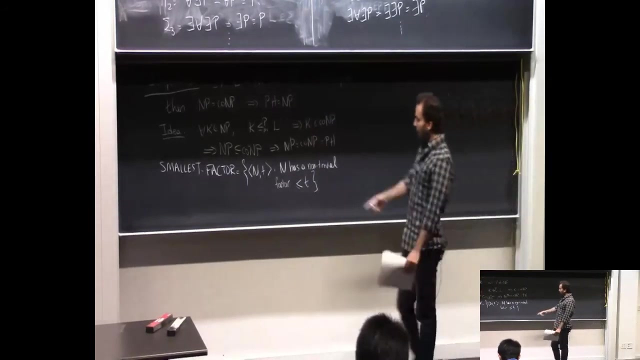 version of a factoring problem. let's call it smallest factor. So this one, let's say it's a pair of numbers- and T, such that N has a non-trivial factor Less than or equal to T. let's say, Okay, so given N and T, we want that N has a non-trivial. 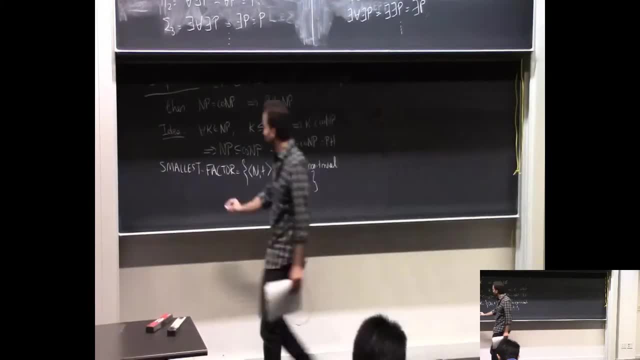 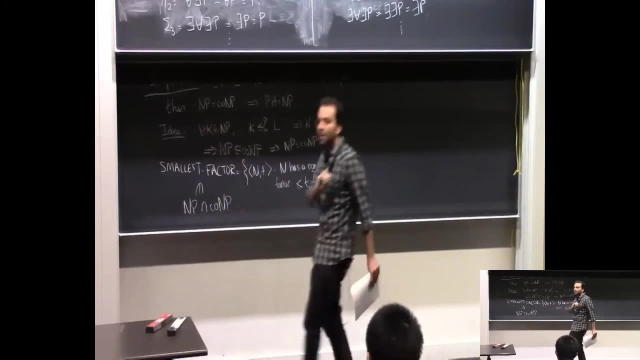 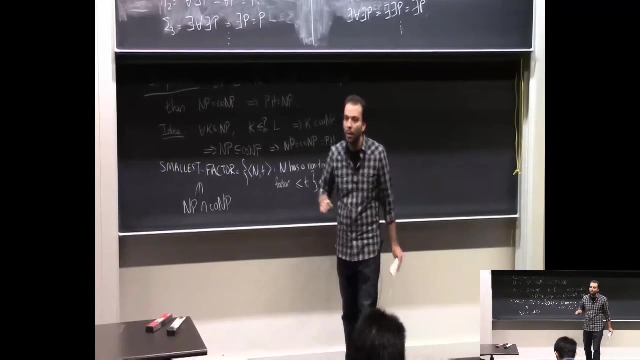 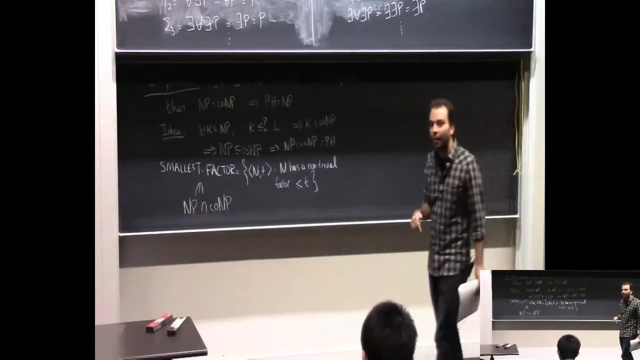 factor less than or equal to T, And this is, I claim, in MP intersection: co-MP. Why is this in MP? How can I prove to you that this is in the language and I give, yeah, I give you the factor okay. 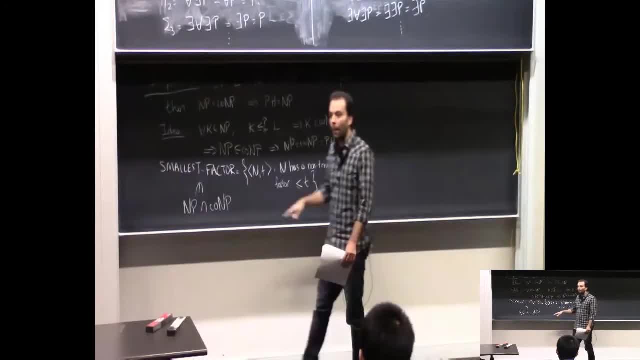 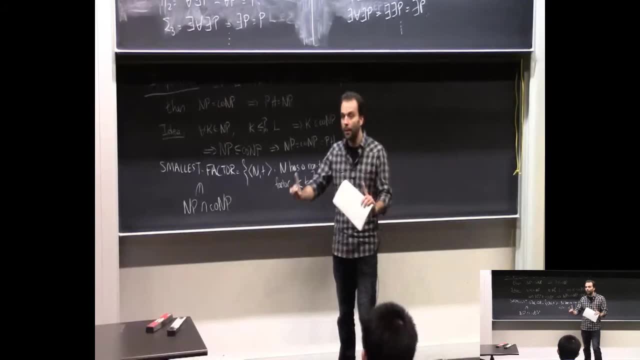 And you can check that it's indeed a factor. How do you show that it's in Co and P? How can, how can I prove to you that there is no factor between 1 and T? The prime factorization: Yeah, Give me the prime factorization. 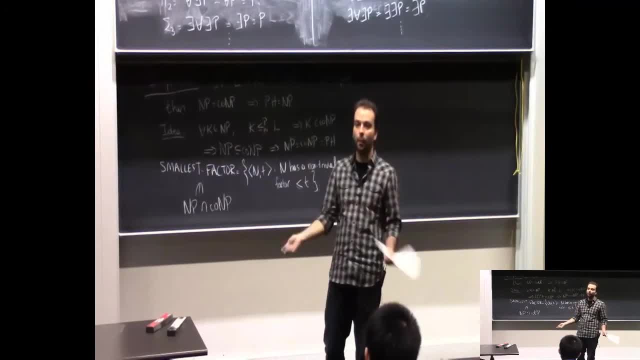 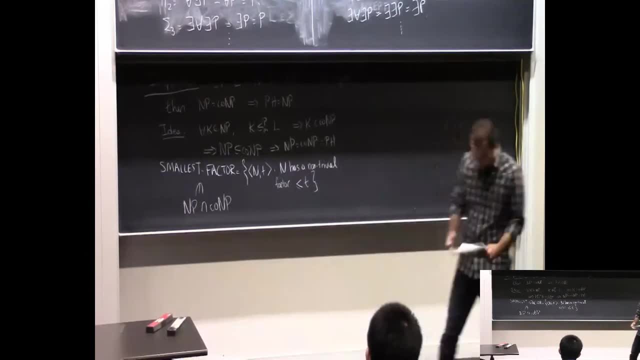 And then first I'll multiply things out and see that it's a prime factorization And then I can check that you know you don't have a factor less than T Good, So yeah, that's kind of a negative result, I guess. 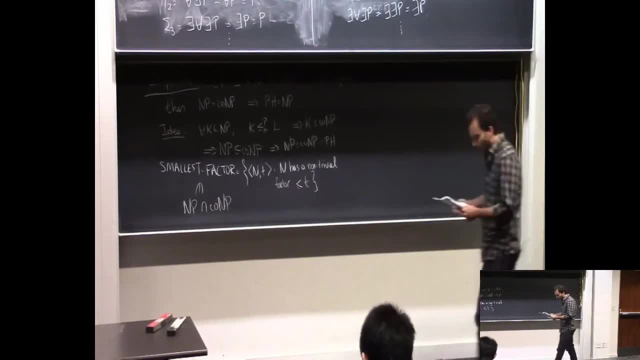 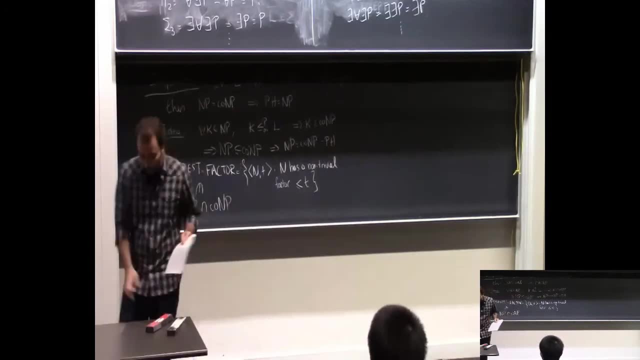 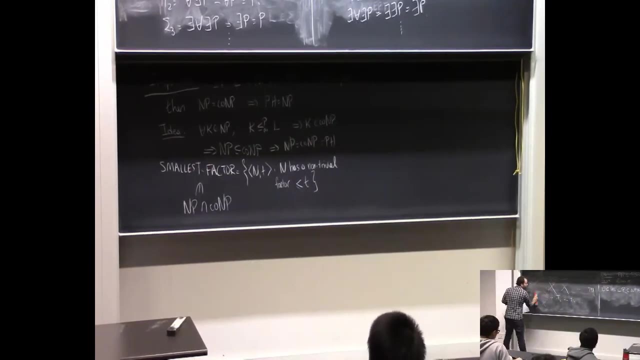 You know it's that this is not NP-complete. All right, so now, quickly, let me say a few things about like you might wonder. you might wonder now, like: does this class have, or these sigmites and pi i's have, complete. 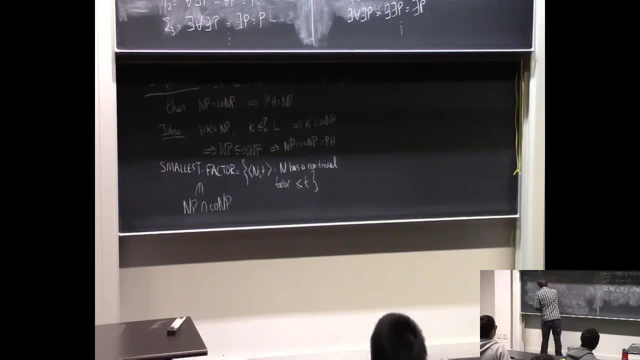 problems? Okay, You know, Ryan might have told you like a language or a complexity class is worth studying if they're like natural complete problems for that class. Has he said that? Okay, So when we certify that it doesn't have this factor smaller than T, we also have to certify. 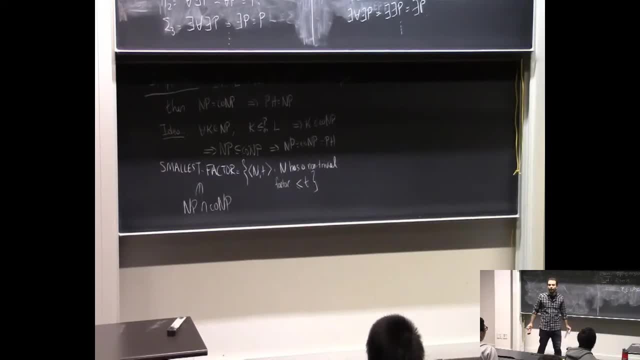 that the factors are prime, right? Yeah, You have to use primality, probably, right. So complete problems. So, indeed, there are some complete problems, Okay, But unfortunately I'm also going to negate what Ryan said, as you'll see. 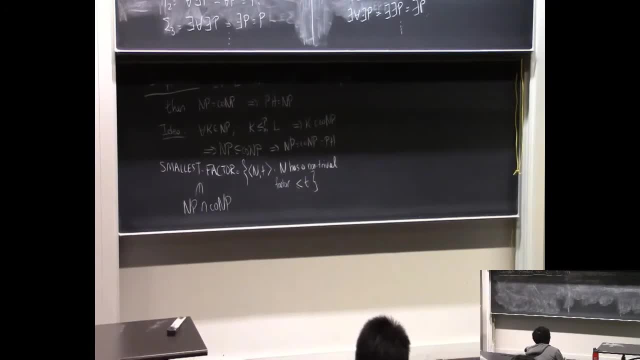 So do we have complete problems for these things? Okay, So there's actually a very, very natural. I mean you might, if I like, forced you to like, come up with a complete problem For sigma i. I think this is the problem that you would come up with. 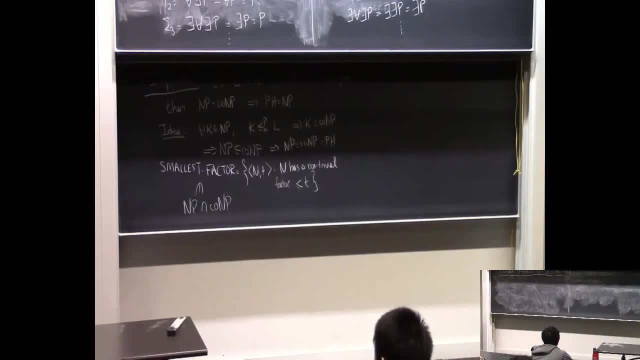 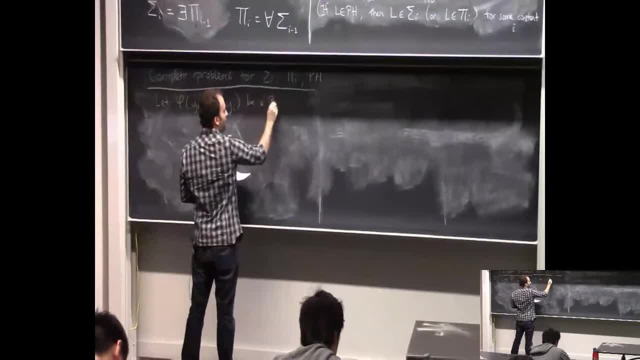 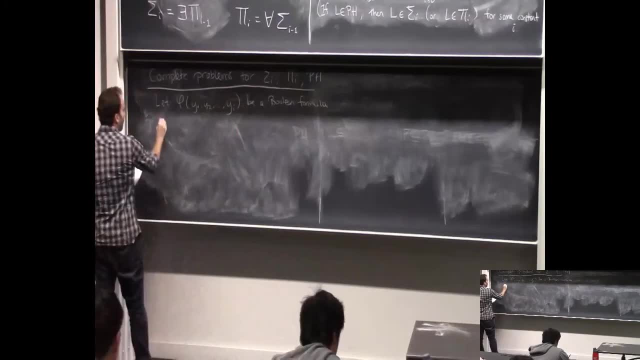 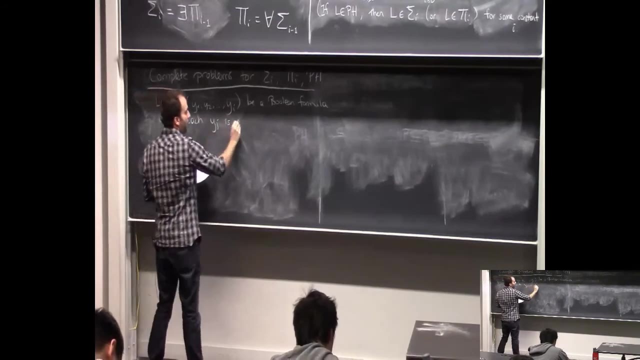 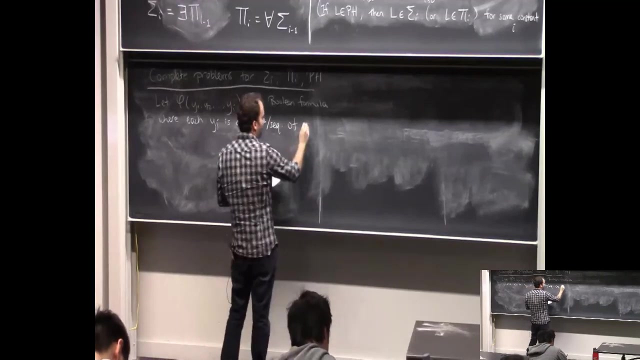 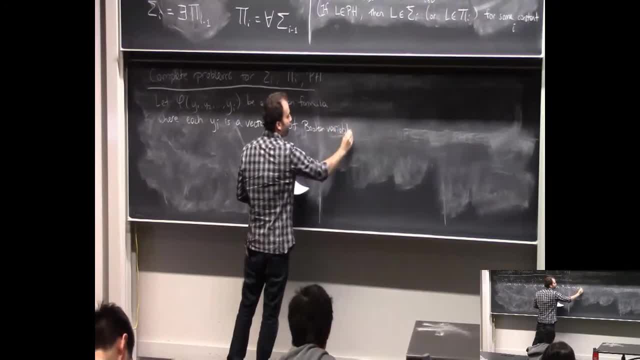 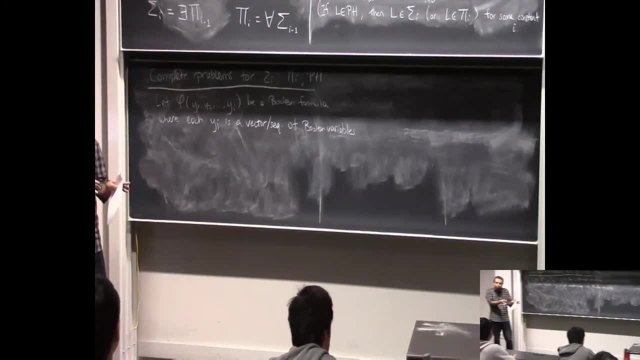 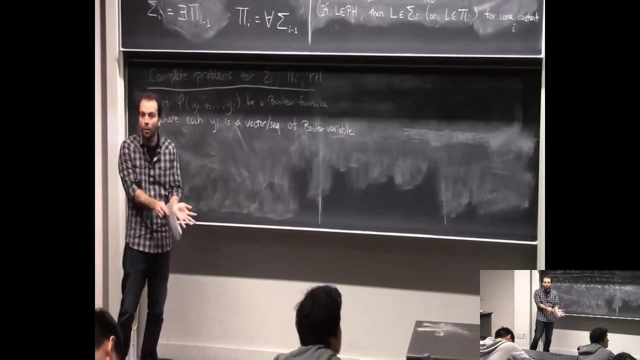 variables. Okay, So I'll think of it this way: I have variables x1 to xn And I partition them into vectors or sets. So y1 corresponds to some subset of the xi's, y2 is another subset of the xi's, and so on. 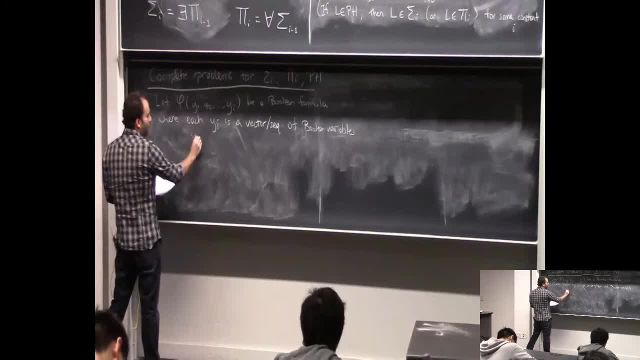 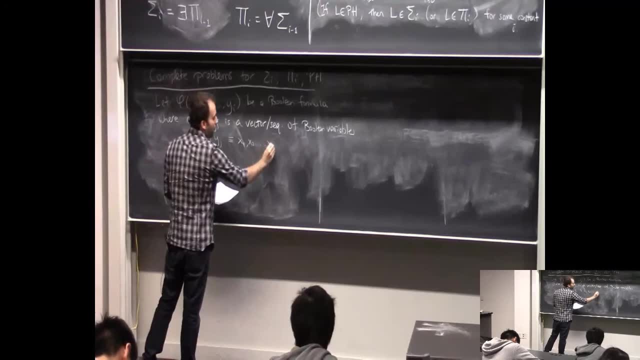 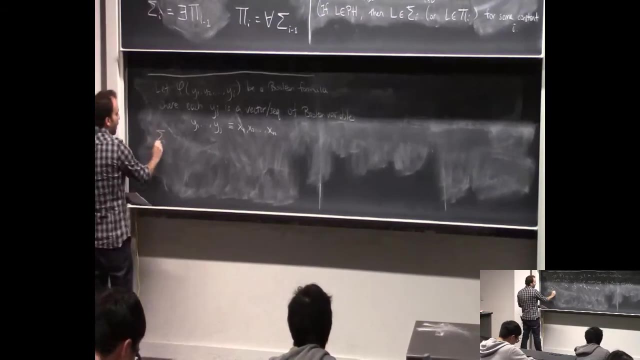 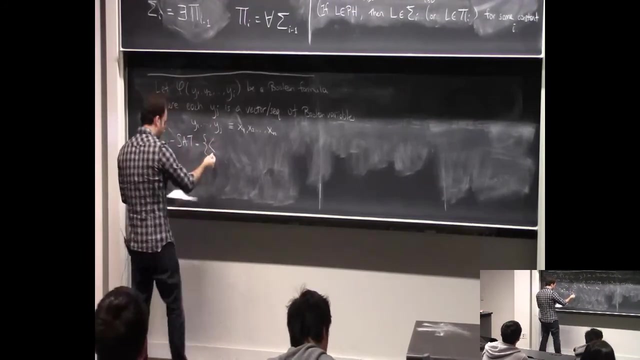 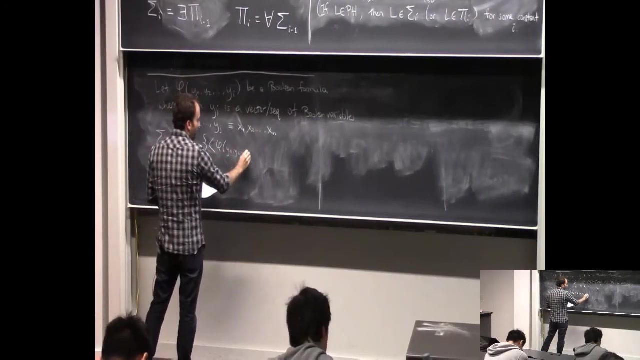 Okay, But together y1 to yj does correspond to all these variables x1, x2, xn. And then now I can define sigma, i set to be the language of all these formulas, y1, y2, yi, such that there exists some value, z1 for all, z2, and so on and so forth. 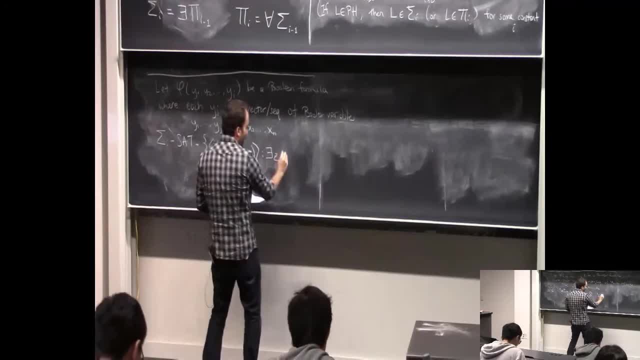 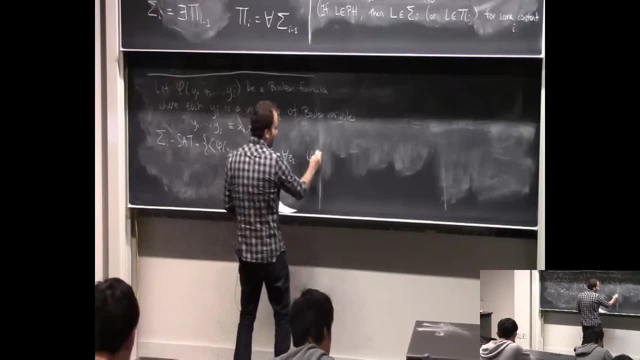 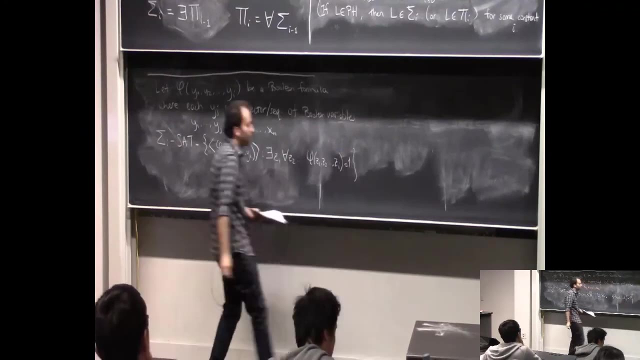 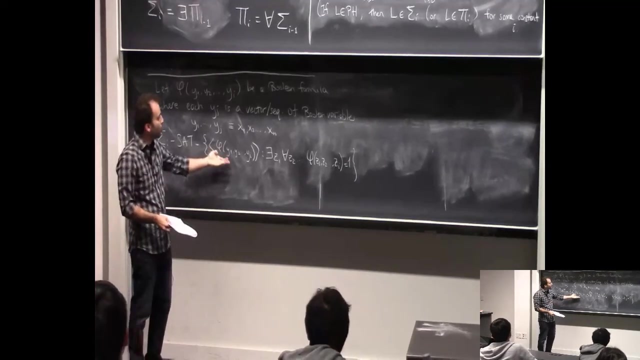 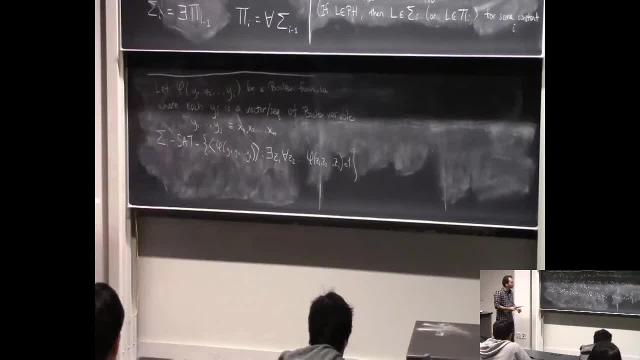 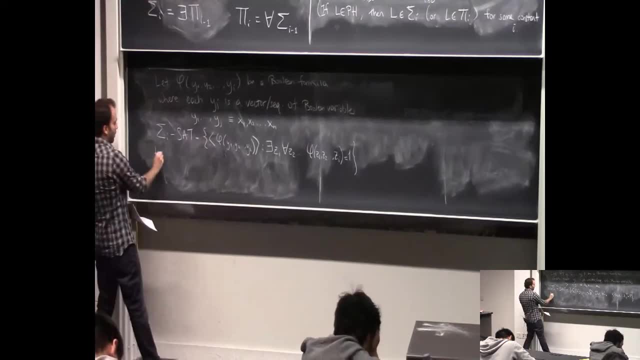 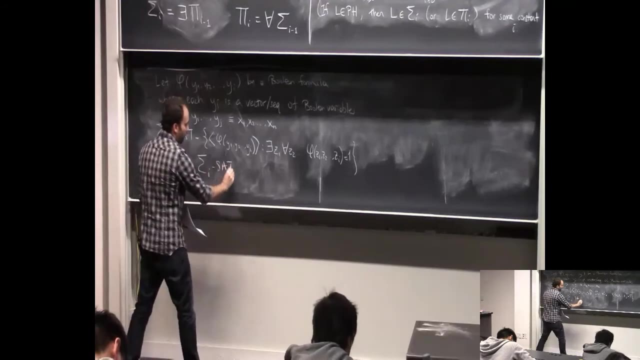 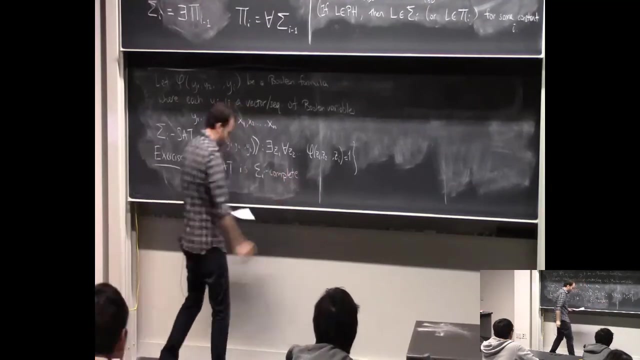 Okay, And then a full year, Yeah, Right, Okay, All right, Okay, Good, I'll leave this as an exercise to you. that sigma i sat is sigma i complete. Okay, similarly, you can define, although I'm not defining, I haven't defined. but 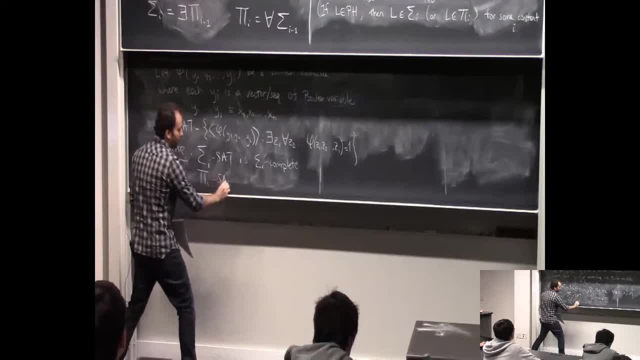 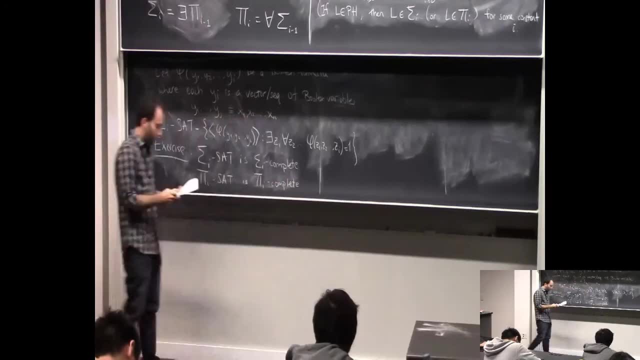 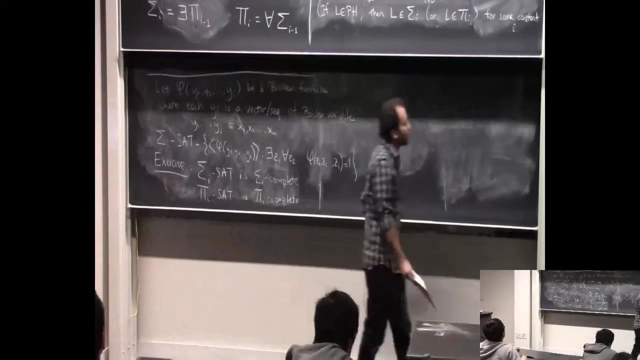 similarly, you can define pi i sat, obviously, and that's going to be pi i complete. Okay, and if you're like, how can I show this? Well, you mean one way is like just to think about, you know, Cook-Levin Theorem. 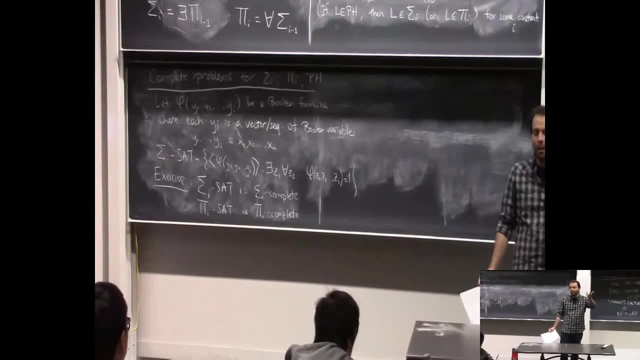 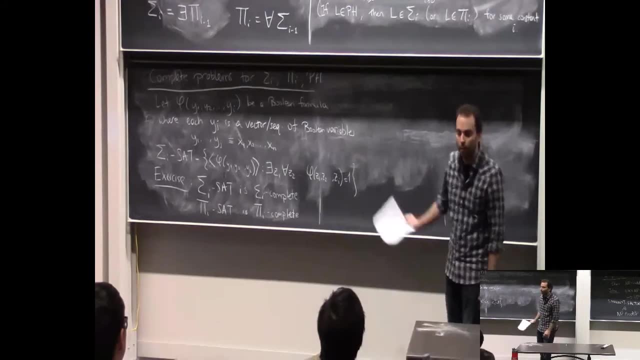 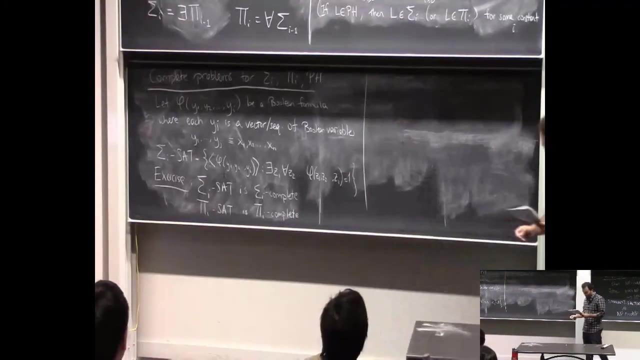 Just close your eyes, imagine the reduction, and then you will see like you can basically do exactly the same thing. Okay, it's like just copy the proof and you'll get the same thing. Obviously, I'm not going to do that. 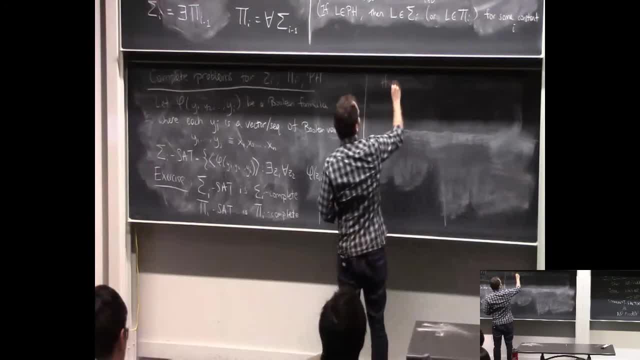 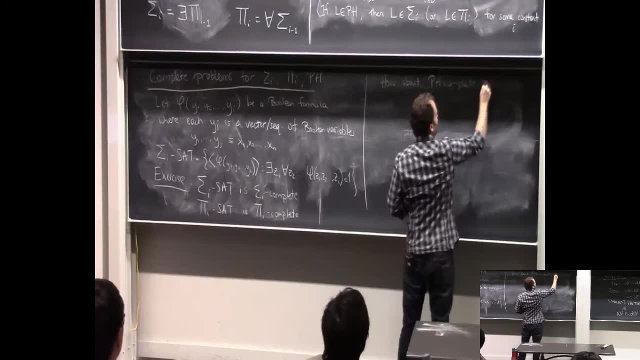 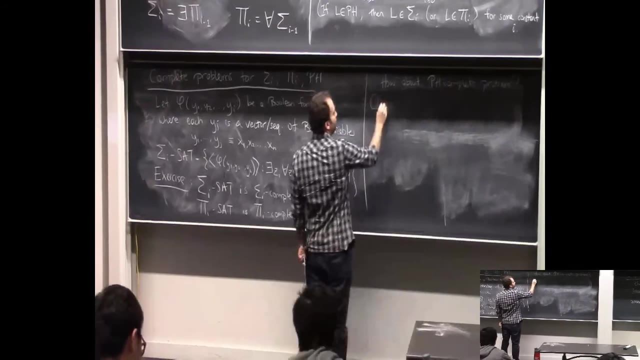 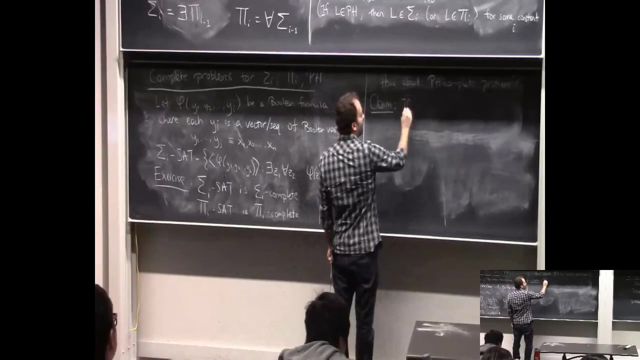 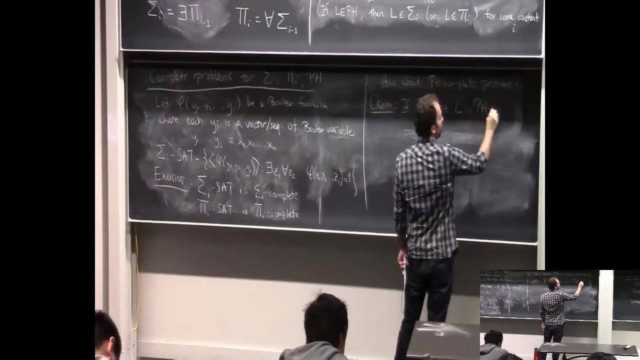 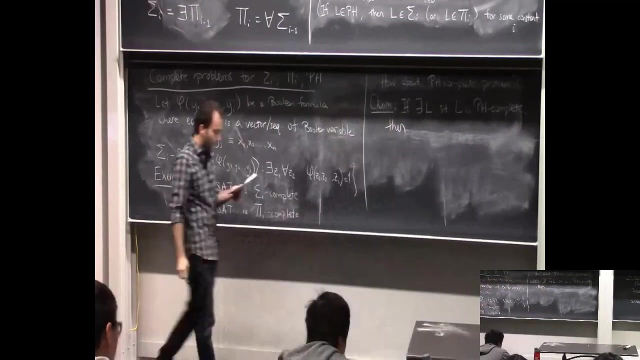 How about pi? i sat. How about pH? How about pH? complete problems. Okay, so now here's the claim: If there exists an L such that L is pH, If there exists an L such that L is pH complete, Then what do you think will happen? 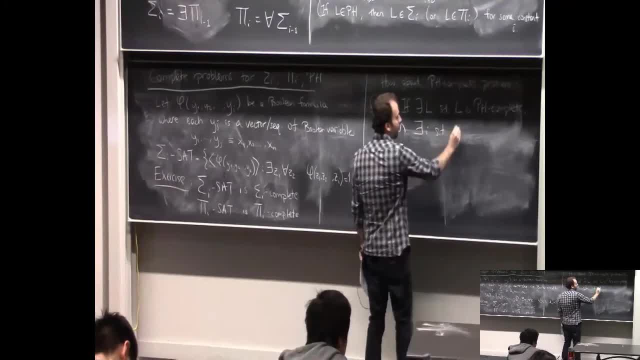 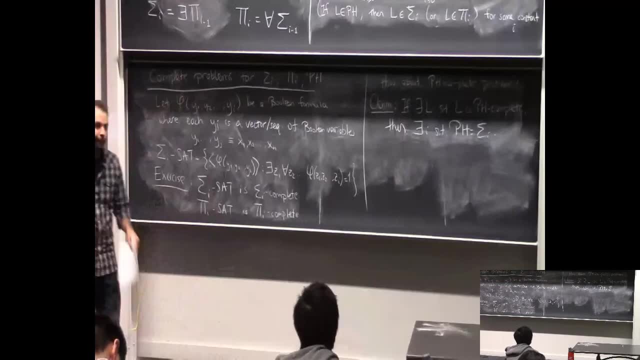 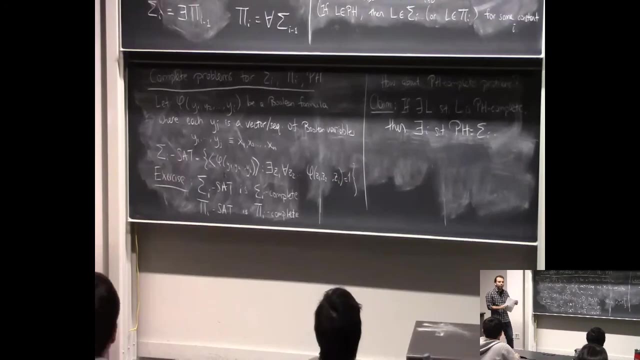 Then there exists i such that pH equals sigma i. The polynomial hierarchy collapses to the it level, And this is why I'm negating what Ryan said, because here's a complexity class, very natural one one, and if you believe that the hierarchy does not collapse, then it does. 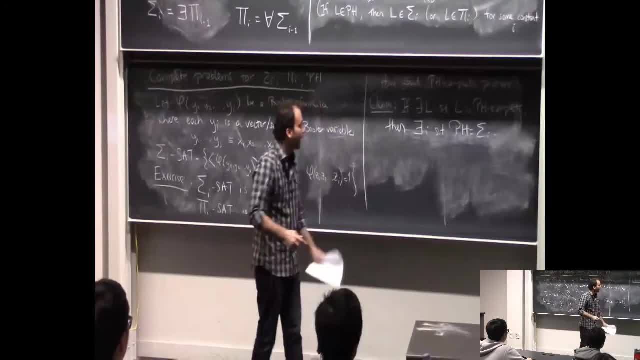 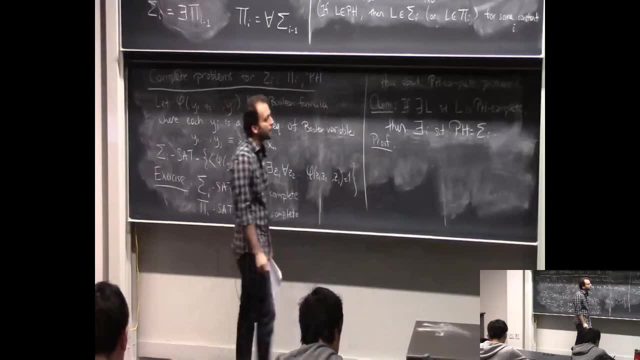 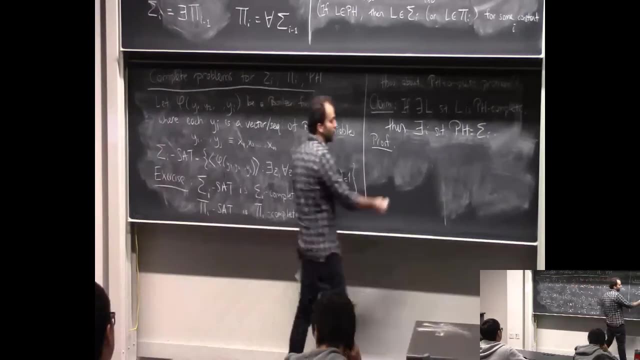 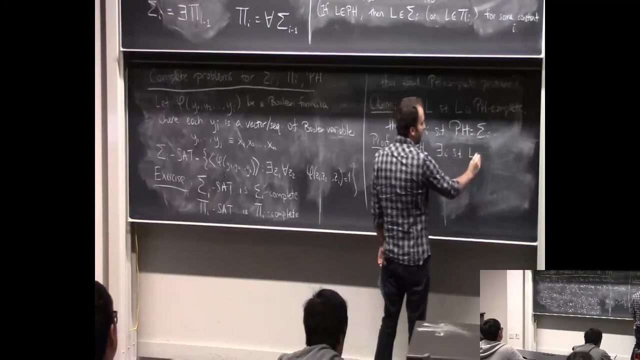 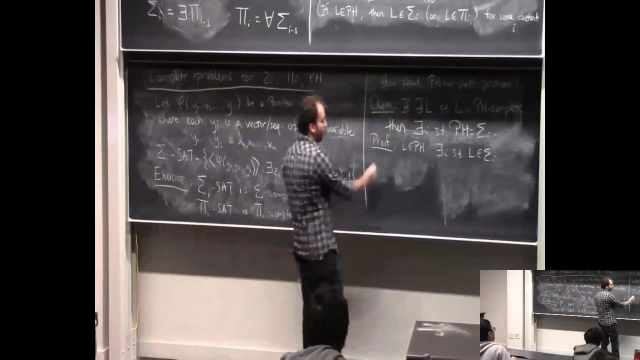 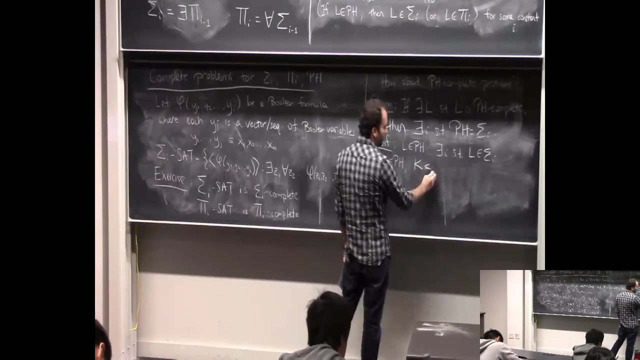 not have a complete problem, and the proof is actually pretty simple. so how can we prove this? if L is pH complete, then if, first of all, it's in pH by definition. so L is in pH, which means there exists some I, such that L is in Sigma I and we know that for all K in pH, K reduces to L. 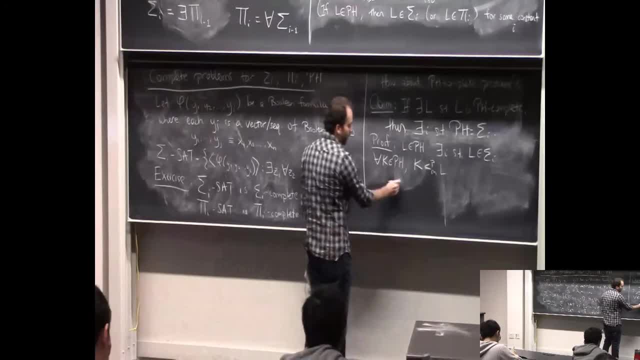 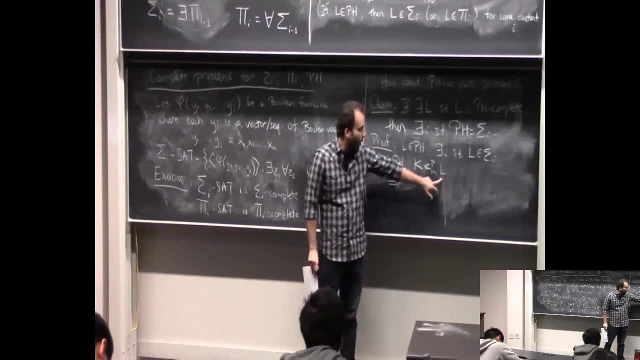 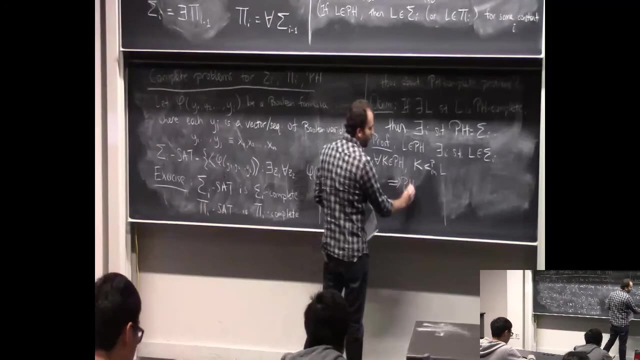 and then what does that mean again by like the similar kind of thing that I discussed before? so if K reduces to L and you know that L is in Sigma I, then K is also going to be in Sigma I. okay, so this implies that pH is contained in. 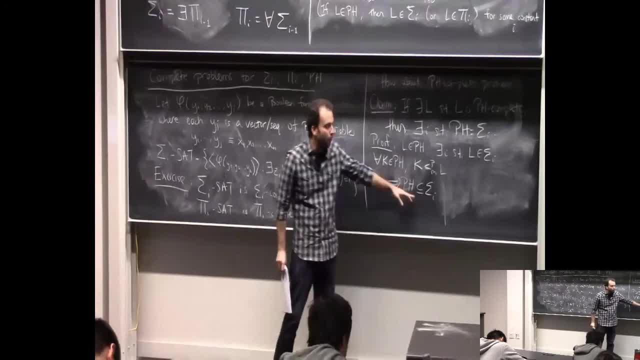 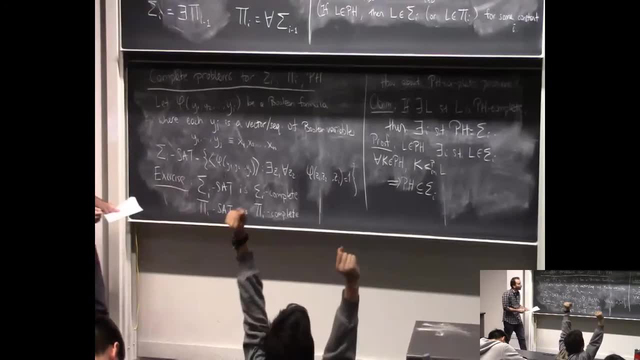 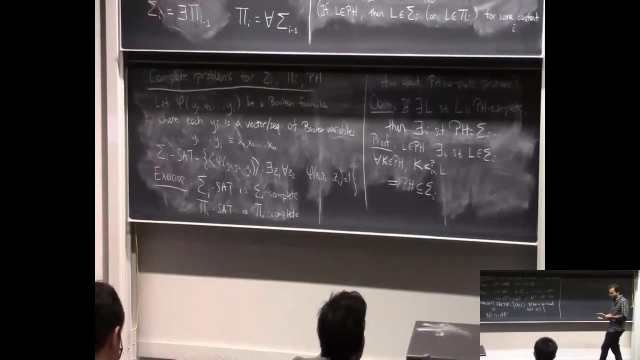 Sigma I. everything in pH can be put into Sigma I. okay, so now we can. last thing I want to explore is: okay, so what about the relationship between pH and p-space? so we saw that pH is contained in p-space. would you expect them to be equal? let's say hey, so you know. 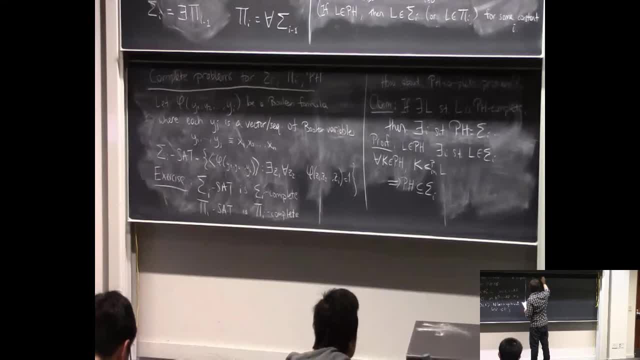 that you know pH is contained in P-space. But now I mean, I guess you can guess, but you also know TQBF is P-space complete. And you also know that if pH was equal to P-space, then pH would have a complete problem. TQBF. 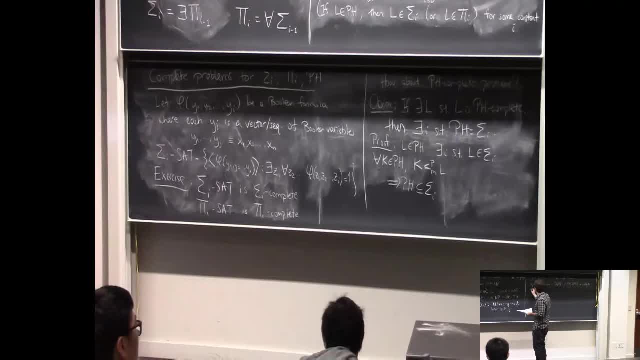 would be a complete problem for it. So corollary is: if pH equals P-space, then pH equals sigma i for sum i Collapses And so, and then we don't, you know, we don't expect pH to be equal to P-space.